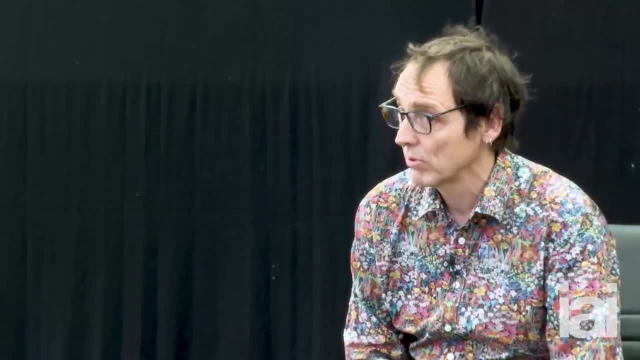 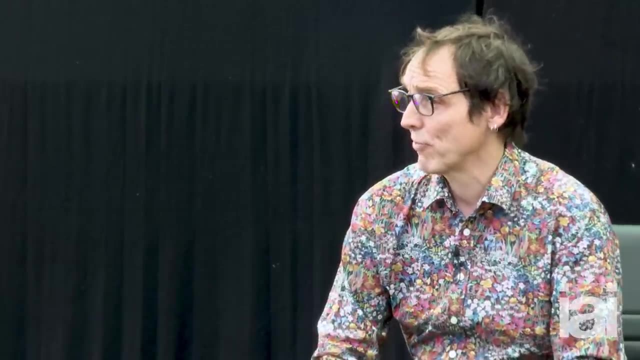 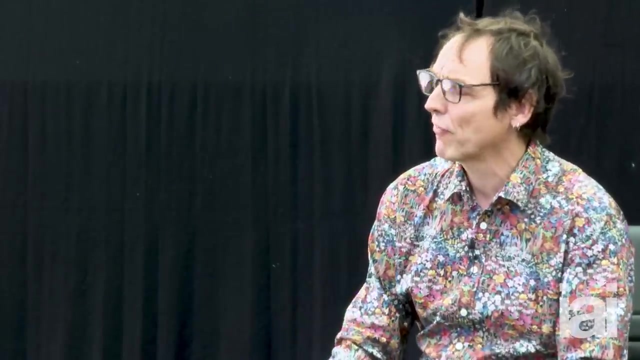 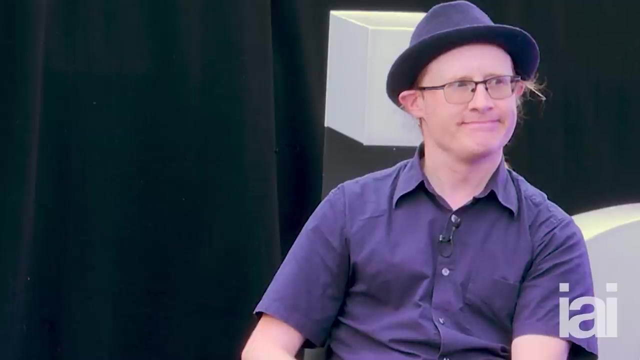 increasing number of challenges it faces. Or is the standard model fatally flawed, And is it time for the next great paradigm shift to a radically different account of the universe? Alternatively, should we conclude that all theories have their limitations and not worry about the flaws, however profound they might be? So to our speakers, Sam Henry is a 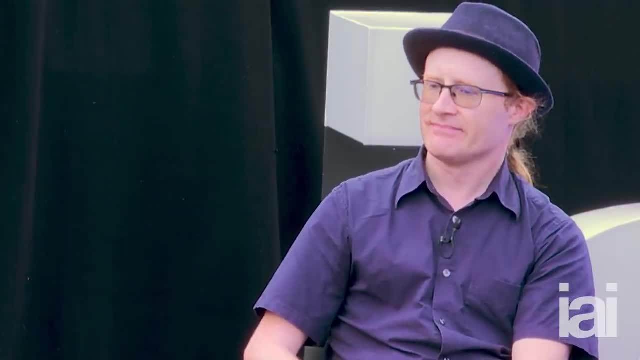 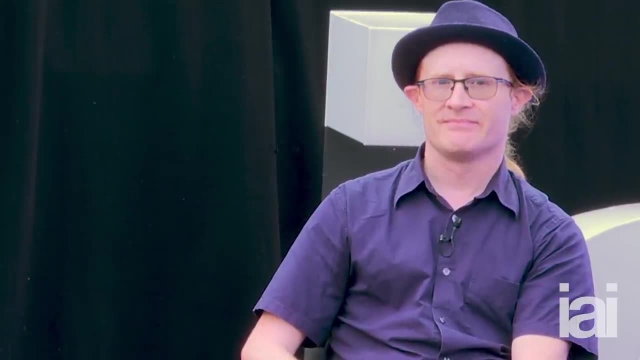 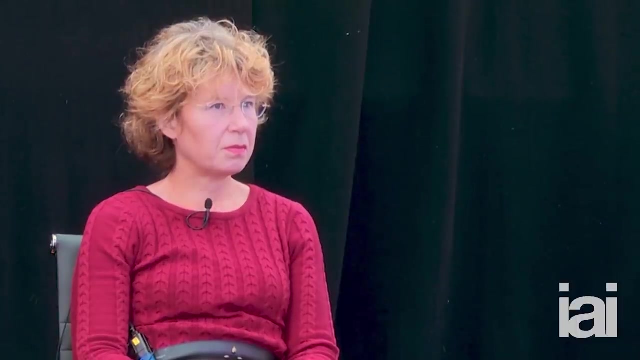 renowned particle physicist working at the University of Oxford. He's authored several academic papers, as well as maintaining his own blog and running several science outreach programs. Sabina Hossenfelder is a theoretical physicist. She's also the author of Lost in Math. 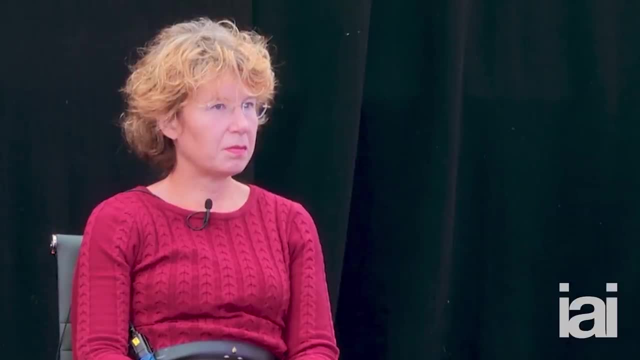 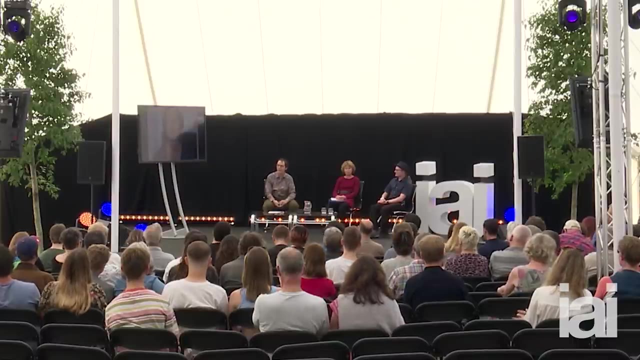 How Beauty Leads, Physics Astray, which explores the concept of elegance in fundamental physics and cosmology, And virtually today, we have Bjorn Ekeberg. He's an Oslo-based philosopher of science who researches the limits of scientific knowledge, And his book Metaphysical Experiments is a critical exploration of the historical foundations of physics and cosmology. 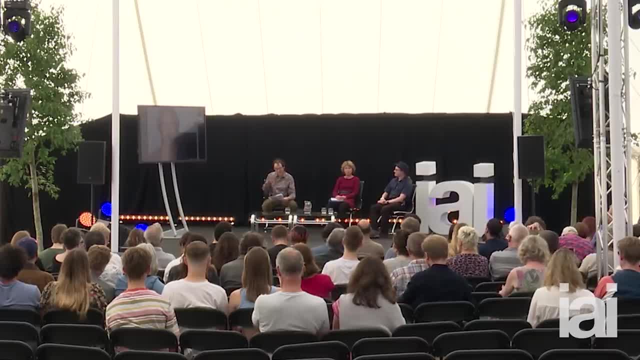 So we're going to begin. I'm going to begin by asking each of the three speakers if they would please. So we're going to begin. I'm going to begin by asking each of the three speakers if they would please to put across the case that they want to make in this discussion. 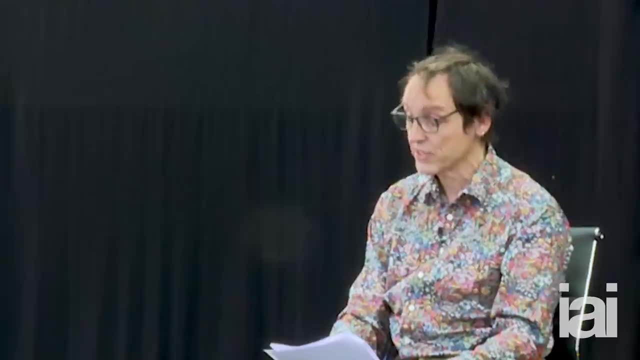 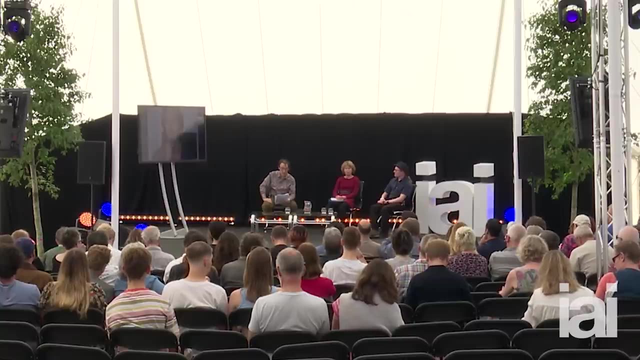 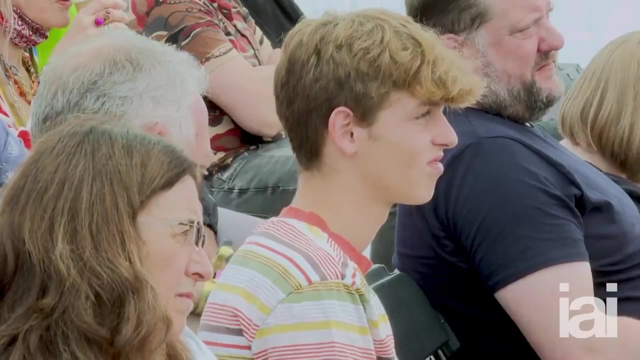 To address this fundamental question that we're asking: is the standard model fatally flawed and is it time for the next great paradigm shift? So first of all, I'm going to go to Sam. I do like the sound of a next great paradigm shift because, although particle physics is never dull, 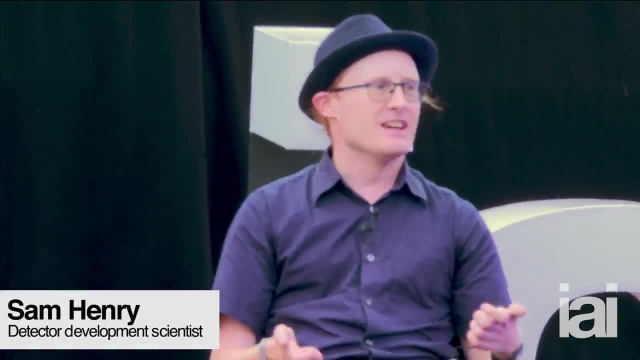 at the moment. we'd really like to see a bit more excitement. It's been 12,, 13 years since the last one and we're still in the process of doing it. So first of all, I'm going to go to Sam. I do like the sound of a next great paradigm shift, because, although particle physics is never dull at the moment, we'd really like to see a bit more excitement. 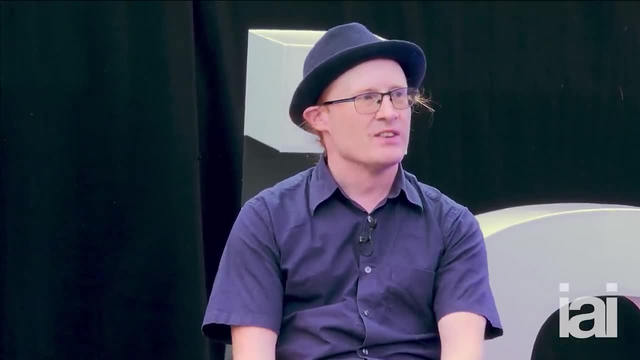 So first of all I'm going to go to Sam. I do like the sound of a next great paradigm shift because, although particle physics is never dull- and we found the Higgs boson and we then hoped that we'd see more discoveries- 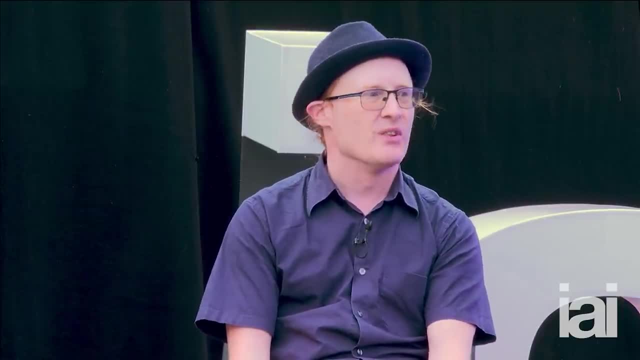 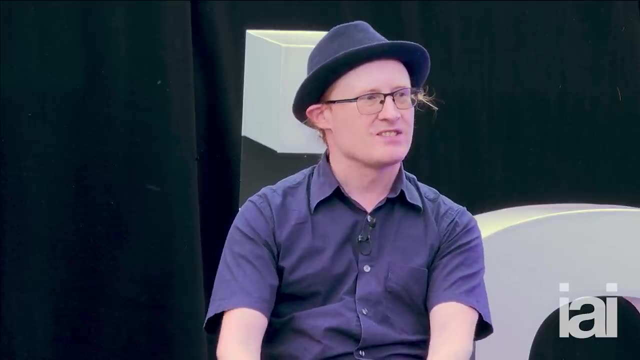 supersymmetric particles, dark matter, some sort of new physics beyond the standard model, But we haven't seen anything like that. In a way, the problem with the standard model is not that it's flawed, but that it's too good. Nearly every measurement that we've made has matched the standard model prediction perfectly. 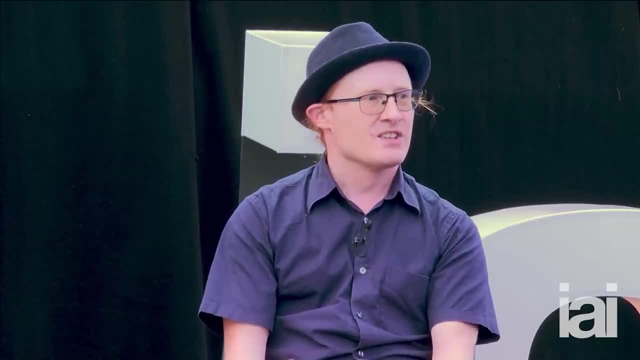 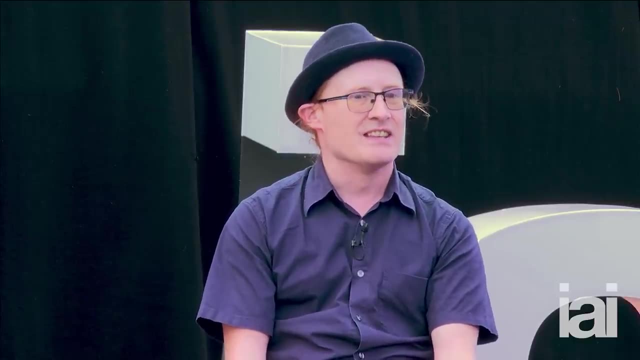 But we know that the standard model can't be the final theory because there are too many unanswered questions that are going to need some sort of new science to explain. So two of the big ones are dark matter and the matter-antimatter asymmetry. 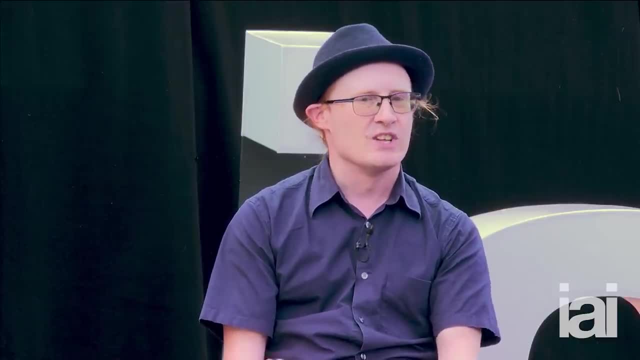 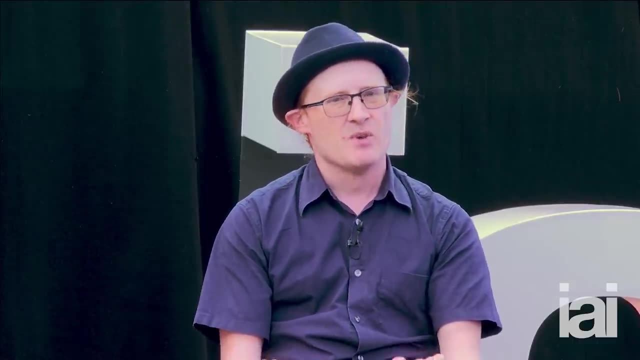 We know the majority of the mass of our galaxy can't be explained with known forms of matter, So there must be some new invisible particles out there, or else something else that we don't yet understand. The standard model predicts that particles and antiparticles are so symmetric that they should have just annihilated after the Big Bang. 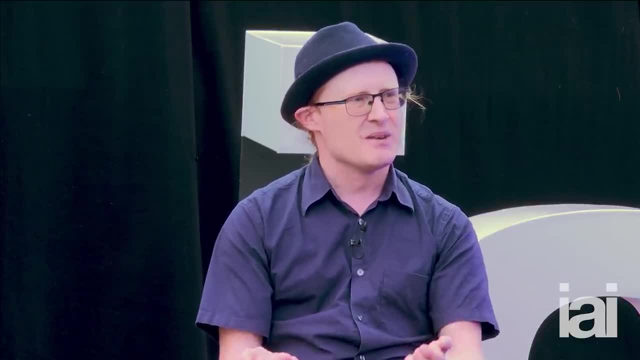 and the universe that we see shouldn't exist. So there must be some subtle asymmetry that we don't yet know that can explain why we're here. Since we know the standard model, we can now look at the universe. Since we know the standard model, we can now look at the universe. If we know the standard model is incomplete, then we would expect to see some cracks forming by now, some measurements that don't quite match the theory, And that's why the muon g-2 result from this year was so interesting. The Fermilab laboratory in the US measured the g-factor of the muon. 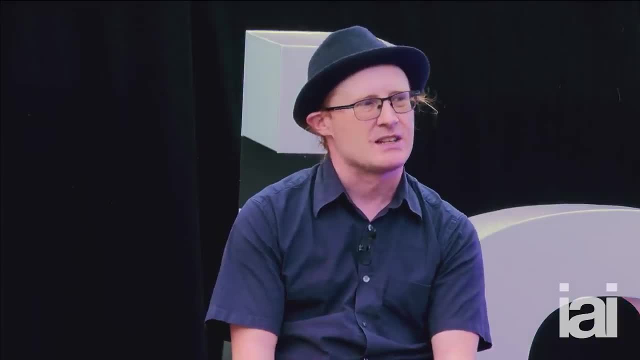 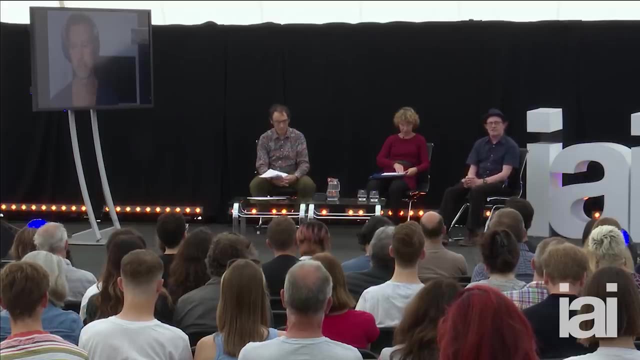 the measure of the magnetism of this particle and they showed that it didn't quite match the standard model prediction. So this could be a sign of something new, a new force we don't yet know. There never seems to be any shortage of theories of physics beyond the standard model. 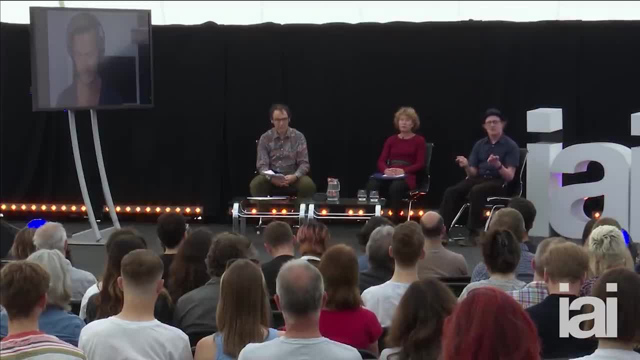 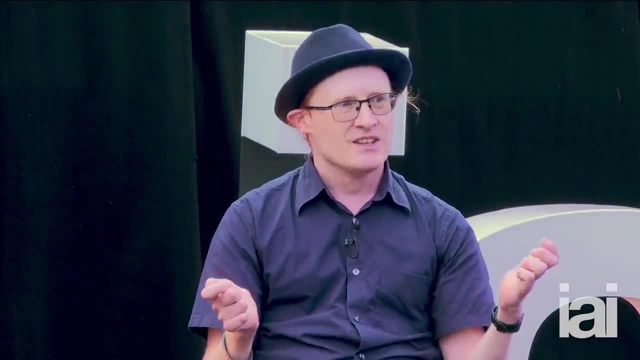 We used to be able to find lots of papers that were using these theories to predict papers just beyond the sensitivity of current experiments. We then built better experiments, did the measurements? we didn't see anything. So does this mean that these theories are wrong? Well, when you check a small print, it's a bit more complicated. There were assumptions made in these predictions and if you change these assumptions, these particles could still exist, just heavier and harder to find. But it's now getting harder to find papers making clear predictions. 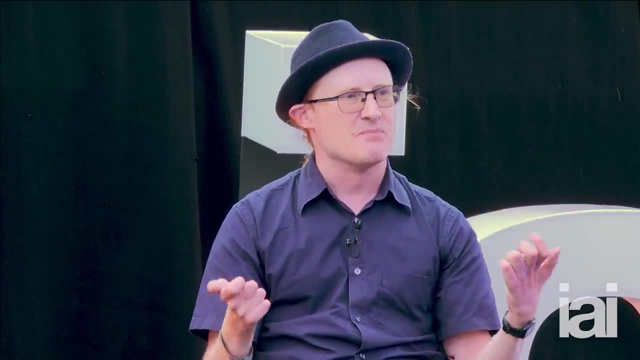 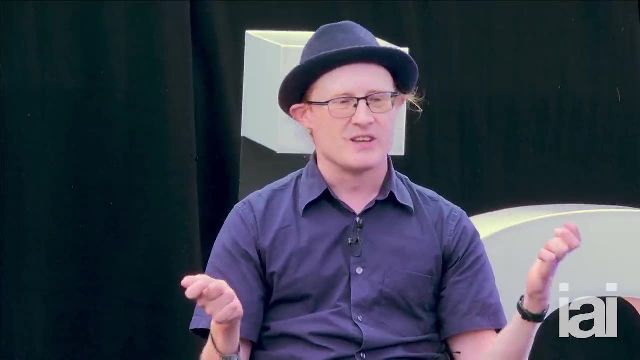 and theories like supersymmetry- that we were once told would be the next big thing in particle physics- that now seem to be terminally out of fashion. At this point, it'd be really great if something unexpected happened, if we saw something that nobody predicted, or some radical new idea came along. 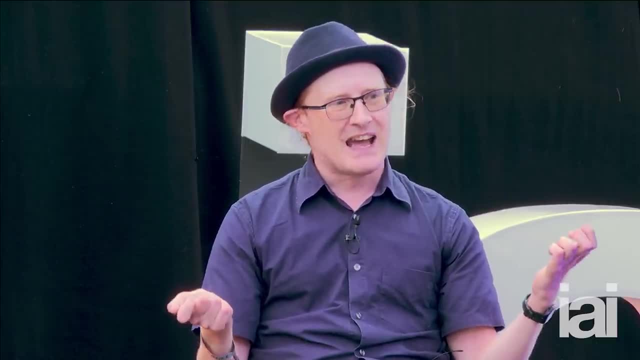 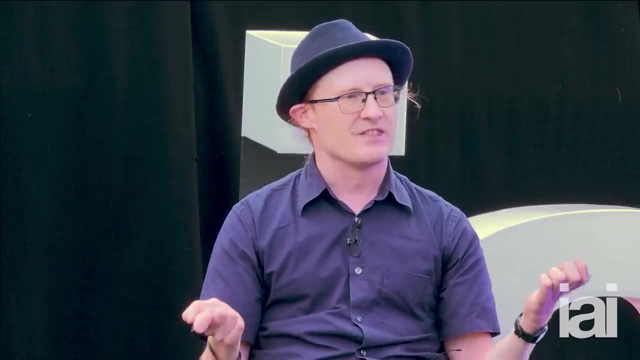 that would really shake up the field and make it exciting. But is that going to happen? Probably not. The less exciting interpretation is that we were just too optimistic about what we could see in the first 10 years of the Large Hadron Collider. 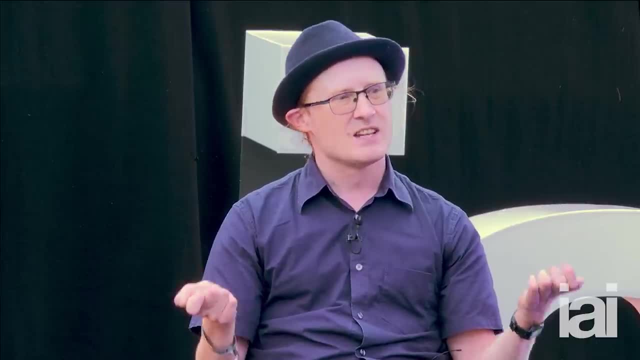 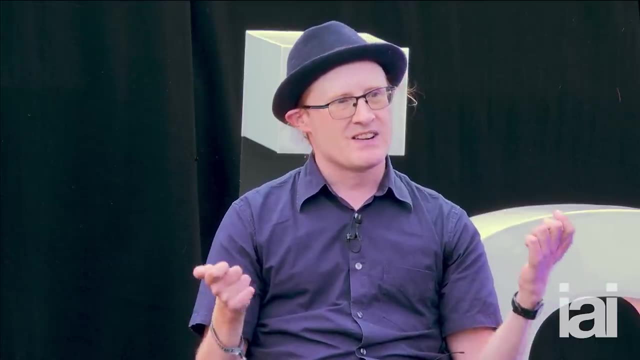 and some variation of supersymmetry or another established theory is going to be correct. but seeing its effects is just going to need more data and maybe another generation of experiments to see that. But a great paradigm shift does sound like more fun. Thank you, Sam. 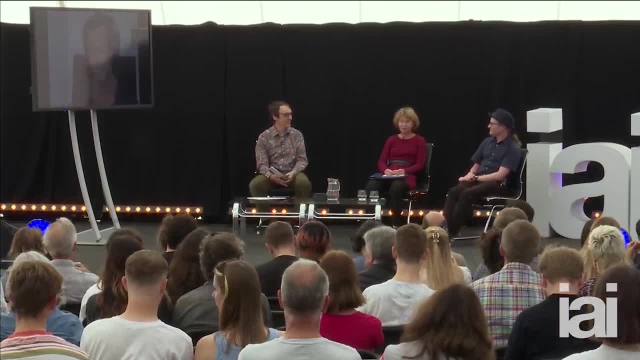 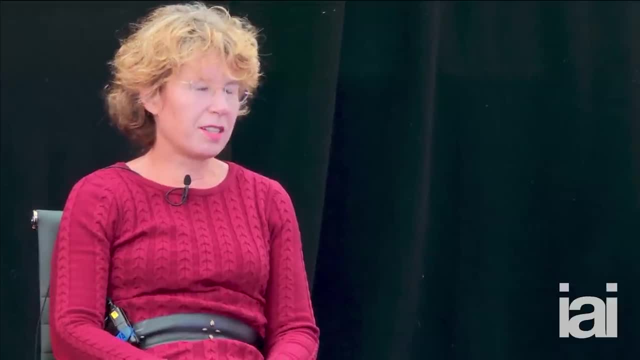 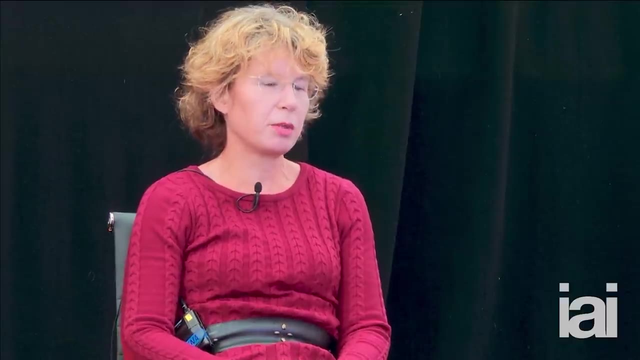 Sabina, do you think we just have to wait, or have we seen flaws in the Standard Model that reveal something deeper? Well, I have to side with Sam that saying that the Standard Model is flawed is a little bit too harsh a judgment, I would say. 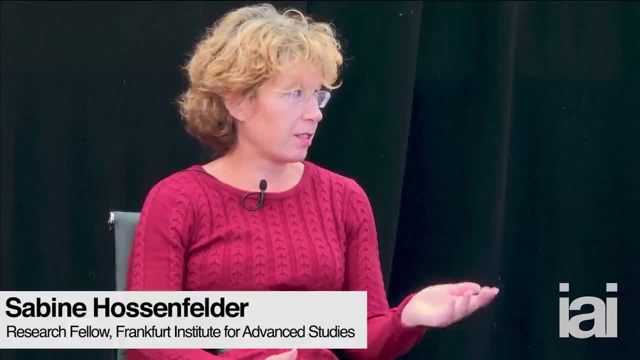 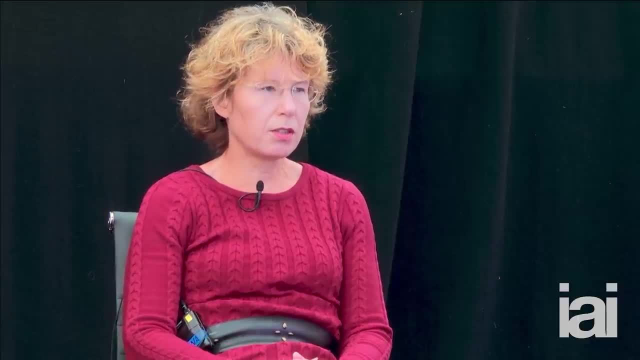 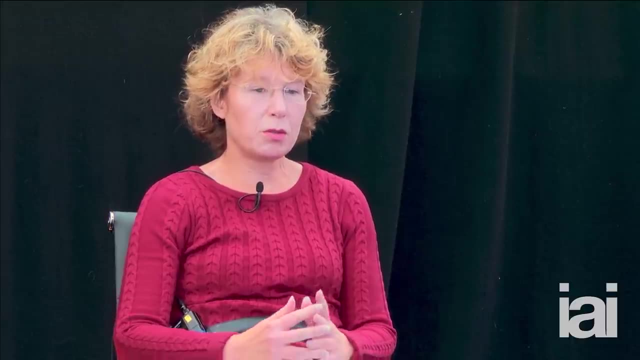 because we know it works perfectly fine, And indeed that's kind of the problem. We would be happy if it turned out to be more obviously flawed, so to say. But we do certainly know that it has some shortcomings, though interestingly I seem to see different shortcomings than you do. 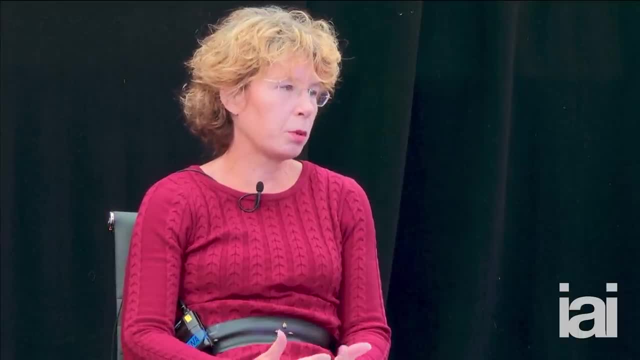 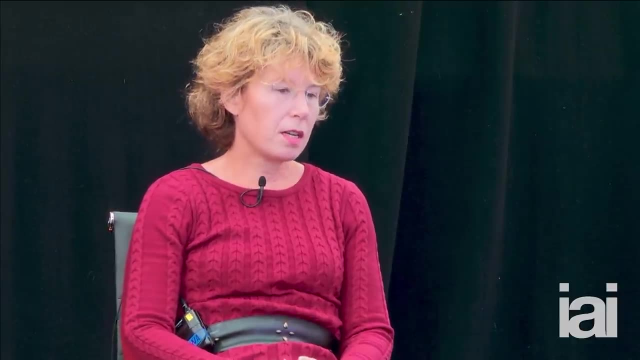 So dark matter, for example, it may be a particle, but maybe it's not a particle, So maybe it's not necessary to change the Standard Model at all. It may be something with our understanding of gravity. That's the problem. The muon g minus 2, yeah, it's kind of intriguing, but I mean for one. 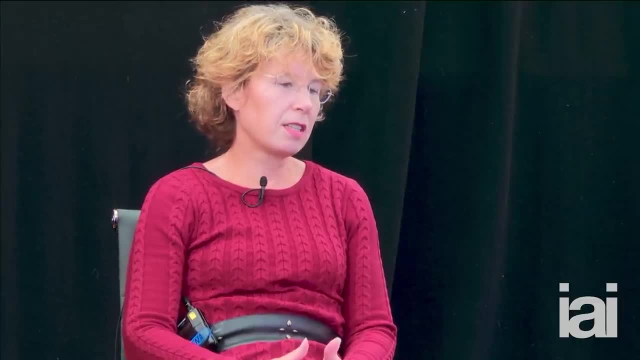 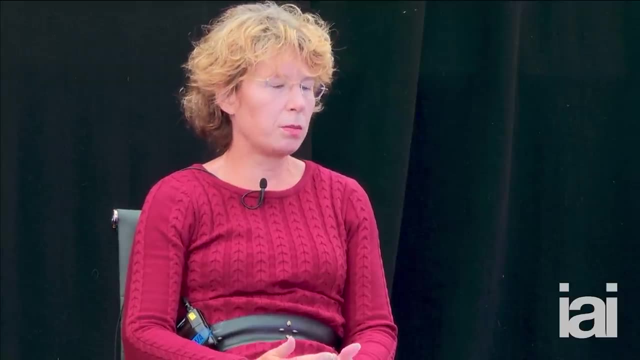 it hasn't reached 5 sigma. That's the one thing, And the other thing is, as you certainly know, it's a hideously complicated calculation. It might very well be that there's just some problem with the prediction from the Standard Model. 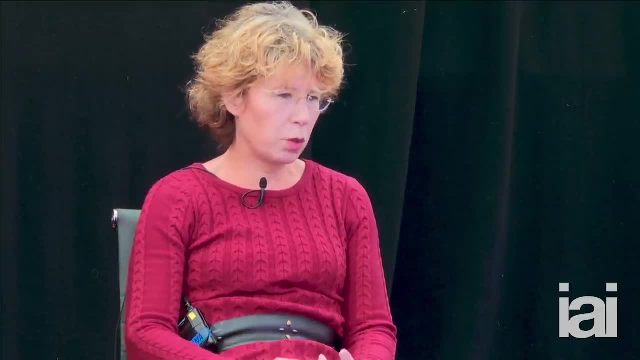 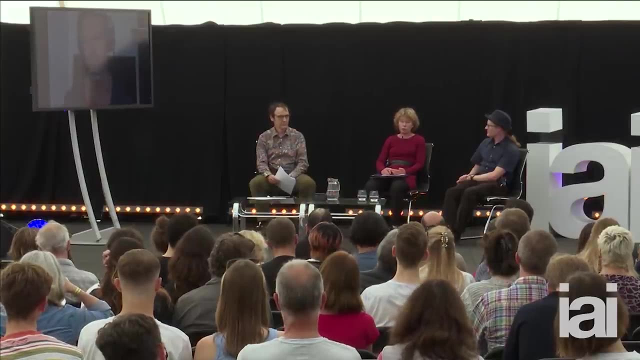 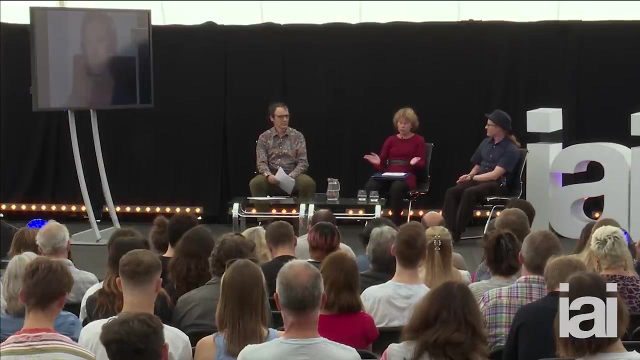 and that it doesn't actually hint that we have to look for new physics. But there are other problems with the Standard Model. One is what you already mentioned: it doesn't contain gravity. In some way we have to combine the Standard Model with gravity. 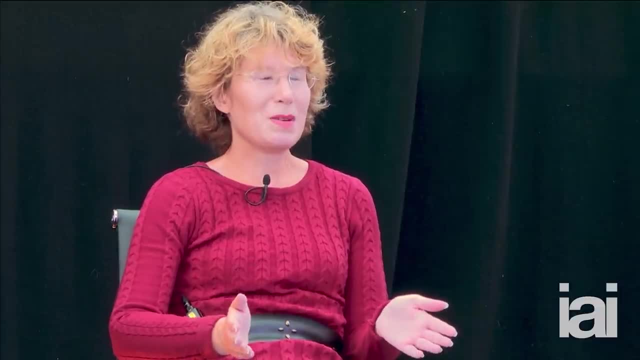 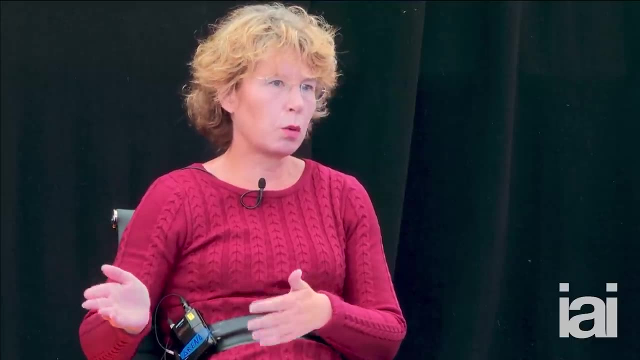 because the particles in the Standard Model do gravitate. We know it, but we don't really know how it works. So that's certainly a big shortcoming. So we need a theory, which is called quantum gravity, that no one really has any idea what it looks like. 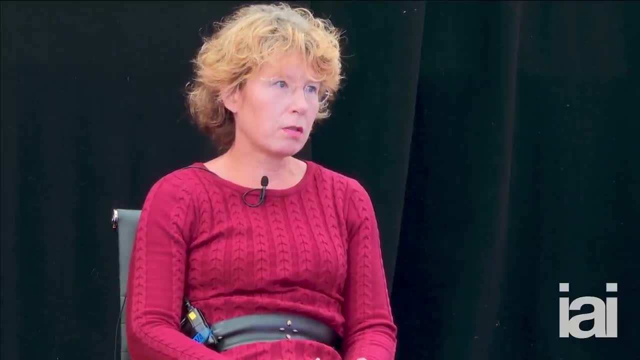 And the other peculiar thing about the Standard Model are the neutrinos. So the neutrinos particle physicists, you know, who work on accelerators, usually don't talk about them much because they're somewhat hard to detect. So the neutrinos particle physicists, you know, who work on accelerators, usually don't talk about them much. 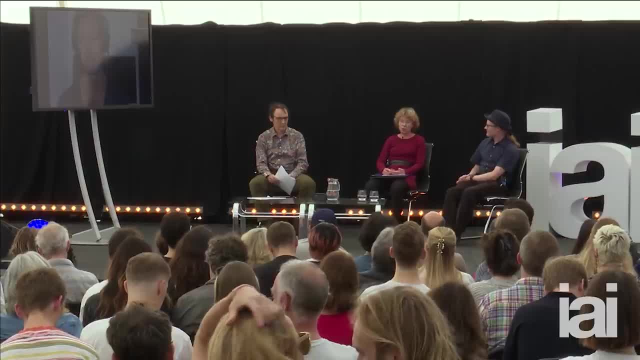 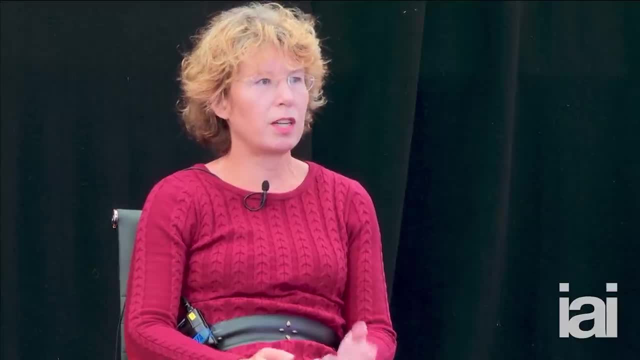 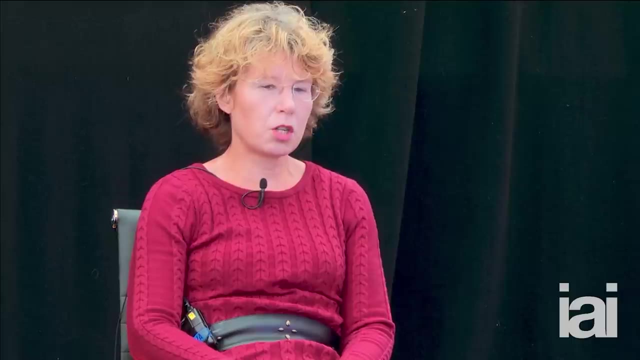 because they're somewhat hard to detect. But the neutrinos are really, really puzzling because from all the other particles in the Standard Model we have a left-handed and a right-handed version from the particles that have masses, But from the neutrinos we've only ever seen the left-handed version. 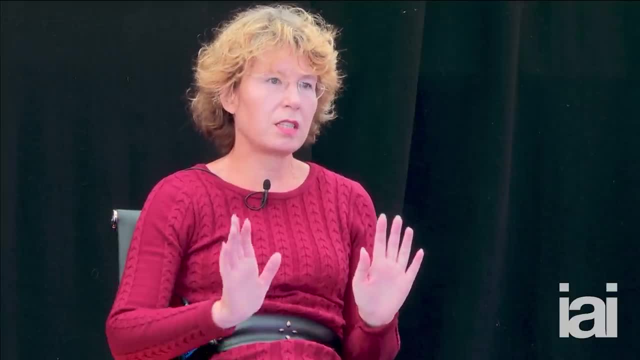 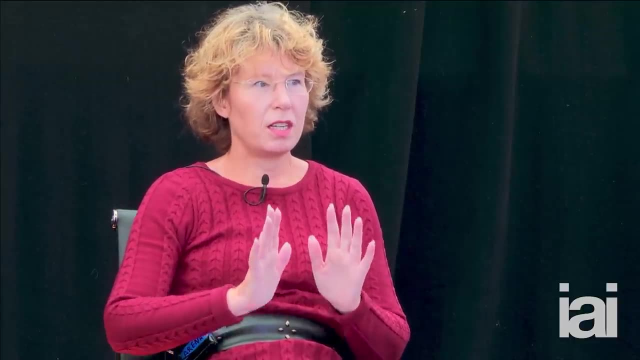 And that's a problem, because we need both the left- and the right-handed versions to give masses to those particles, and we know they have masses. So how does this come about? We know, for this reason, that there's something missing in the Standard Model. Either there have to be right-handed neutrinos which are just so heavy that we haven't seen them, or there's something weird with the neutrinos and they're just different to all the other particles in the Standard Model. And there's actually another anomaly which was not on your introduction. 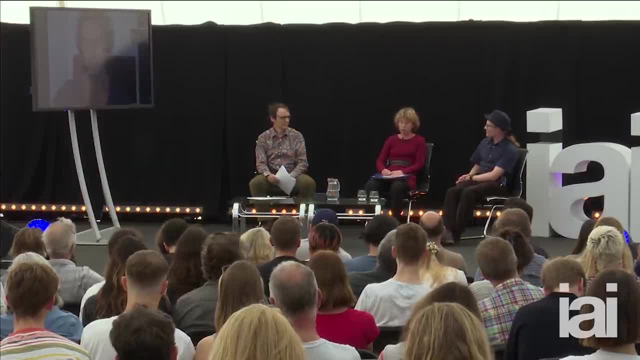 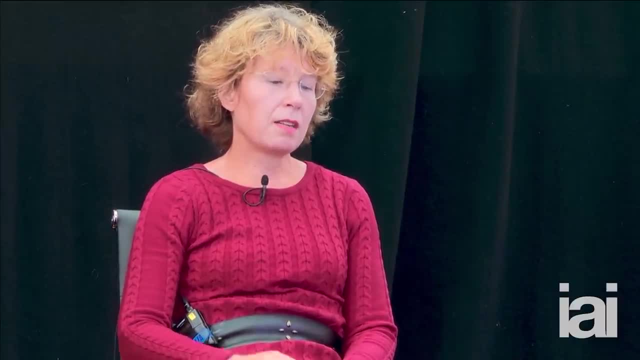 in the Allison D Miniboon data, which looks for neutrino oscillations. That's a signal for Yeah Or neutrino masses, And that signal cannot be explained with the Standard Model And it's actually now at six sigma. last time I looked 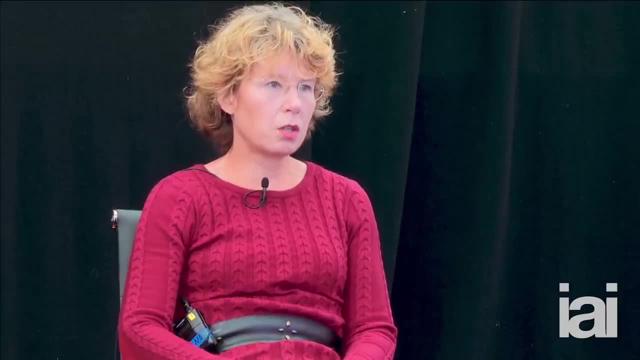 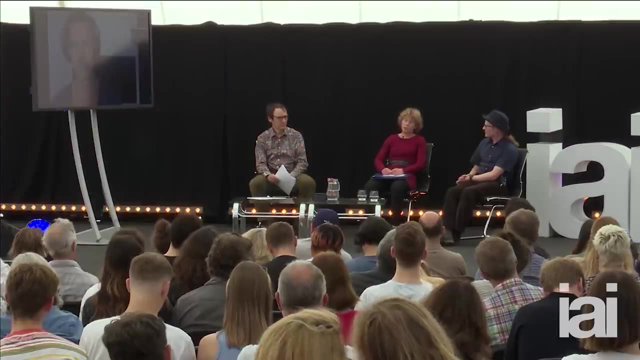 So that's really, really puzzling and indicates to me very strongly that the Standard Model has to be completed. There are probably some particles that are missing, But- and here's the thing- you don't actually have to change the Standard Model all that much. 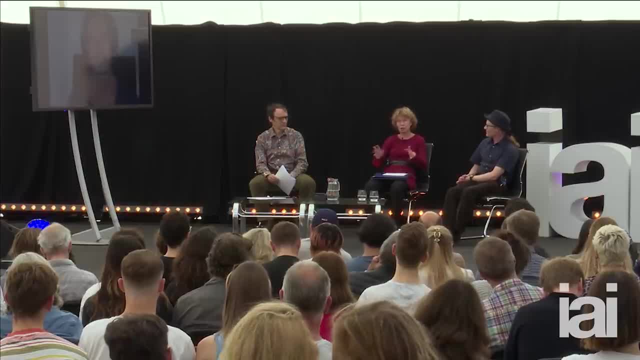 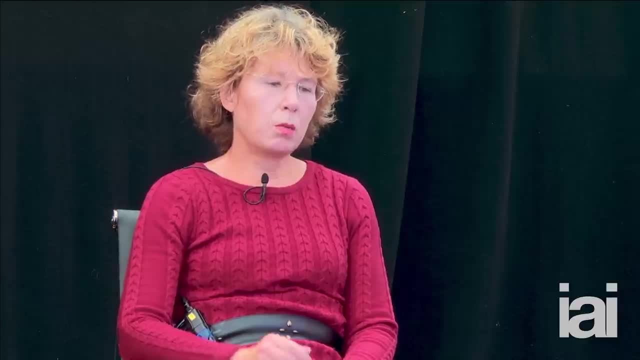 to add a few more particles. You know you can continue using the same mathematical framework and I don't think it will really be a big paradigm. I think where the big paradigm shift is going to come from is it's another thing that particle physicists like to forget. 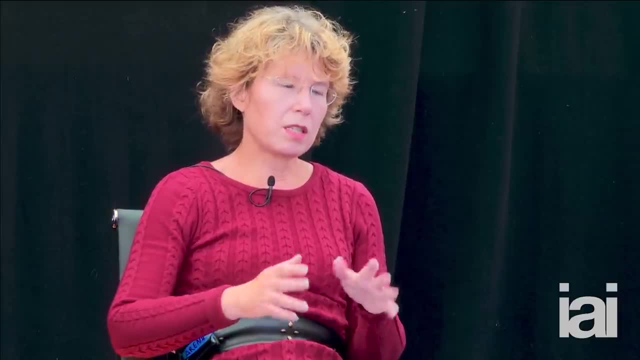 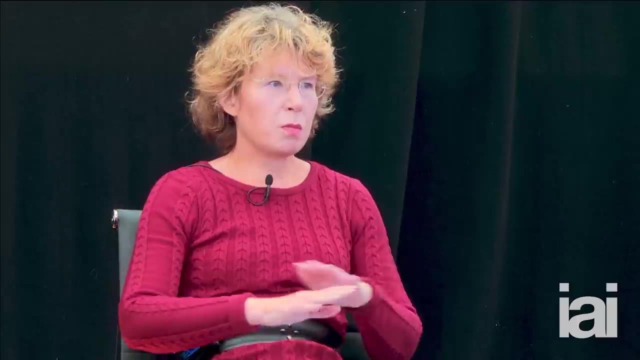 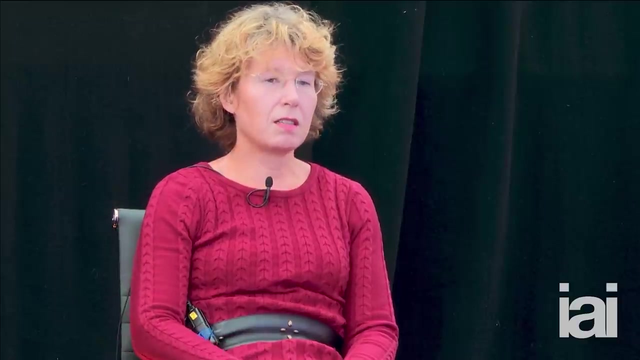 is that the Standard Model deep down is based on a quantum field theory which brings in quantum mechanics onto the entire measurement process, And how a measurement works in quantum mechanics is something that physicists never really understood, And so that's where I think the big paradigm shift is going to come from. 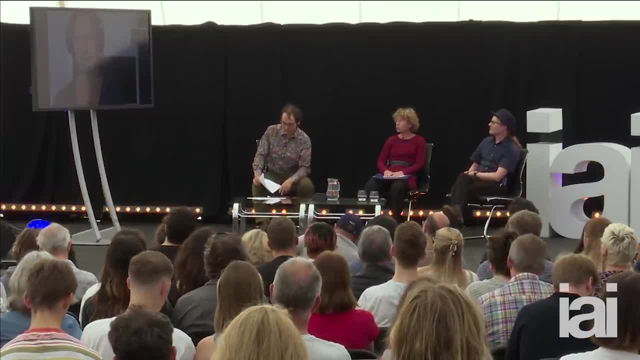 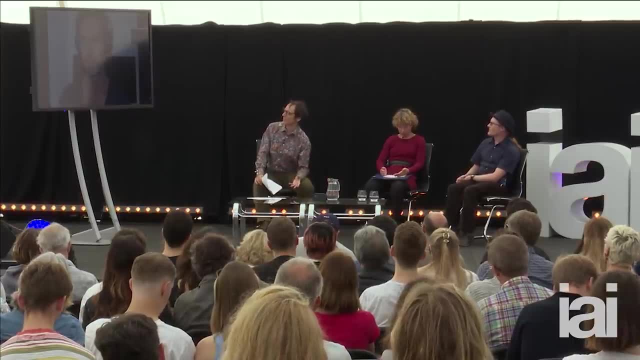 Thank you, Bjorn. we're going to turn to you And this question, the way it's posed, is the Standard Model fatally flawed. You have made the point that actually we should be thinking about there being two Standard Models. There's a Standard Model of particle physics, but there's also a Standard Model of the way. 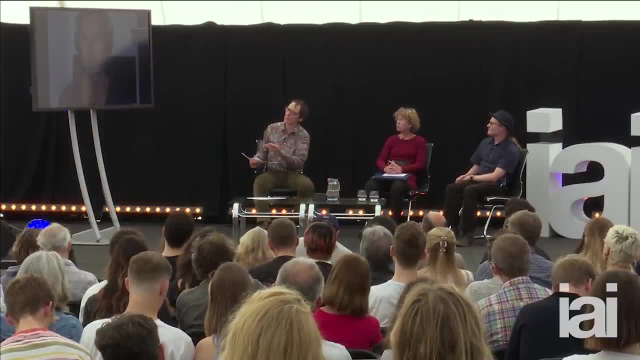 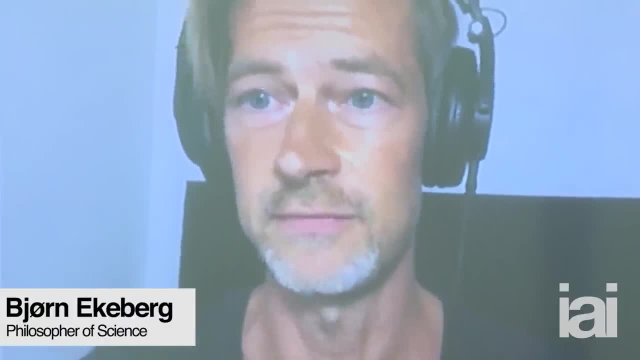 we think about cosmology and that they're not the same thing. So over to you. Yeah, thank you. So there is in practice, these two overlapping spheres of Standard Models. We use a Standard Model also in cosmology And not just in quantum physics. 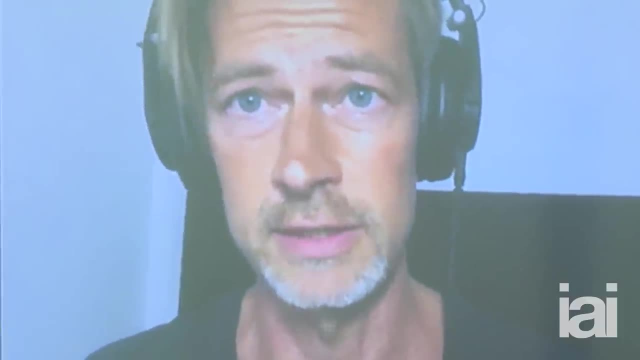 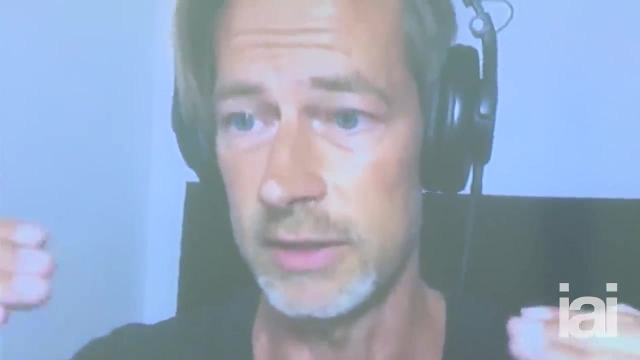 Yeah, In theoretical physics, And the Standard Model in cosmology is more built on the Big Bang theory, with dark matter and dark energy and other building blocks on top of it. So since we're talking about the universe and making sense of the universe, 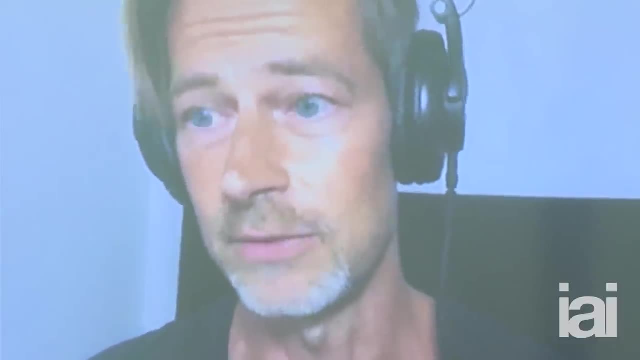 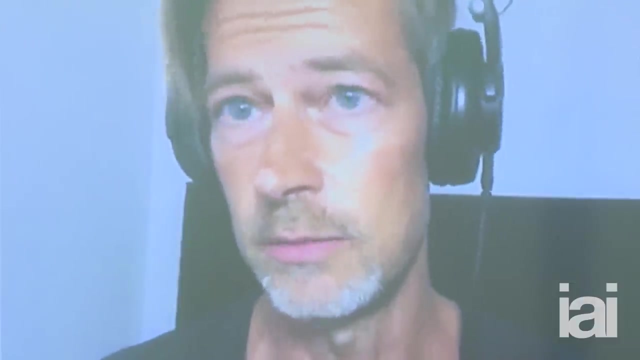 as the theme for the debate. I'd just like to point that out from the outset. I may be speaking to more of the problems I would see with the Standard Model in cosmology than in physics, And so, from my point of view, having followed 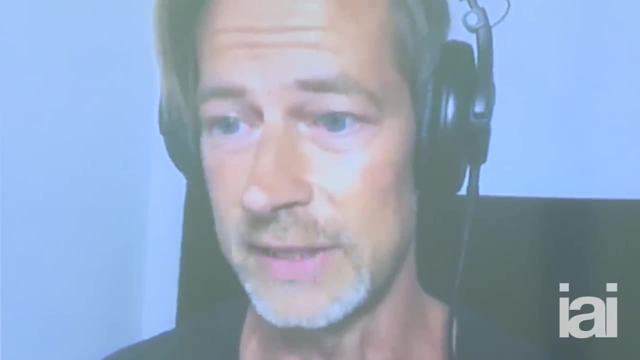 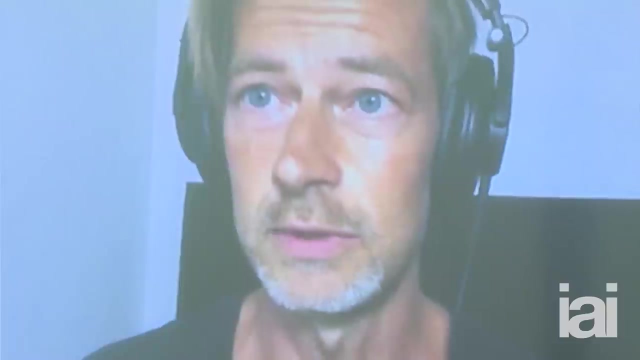 studied and followed this discourse for over a decade. the Standard Model of cosmology looks quite flawed in, I would argue even deeply flawed. But you posed the question of whether it's fatally flawed. And so fatally flawed supposes the science will sort of die out the moment it's shown. 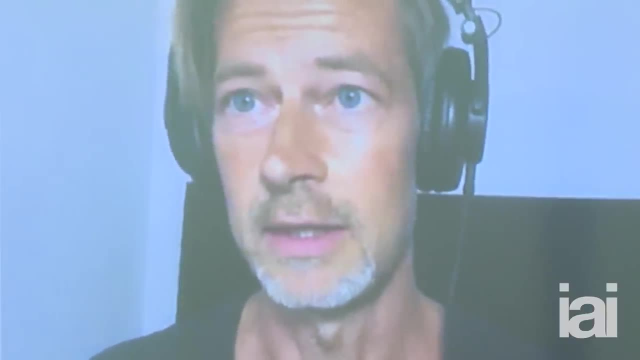 to be wrong or inconsistent in some way, And this is a very idealist notion. Instead, I would suggest it's actually possible in practice. And this is what's happening is that the model can be flawed and it will keep persisting as the only operative model because it's 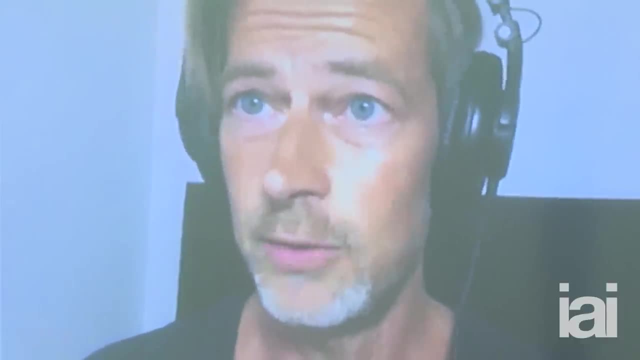 the only one that's put to use. So, in a sense, the point I would like to make is that the science- and here I'm talking about cosmology in particular- is kind of stuck. The paradox is that it relies on a theoretical framework that 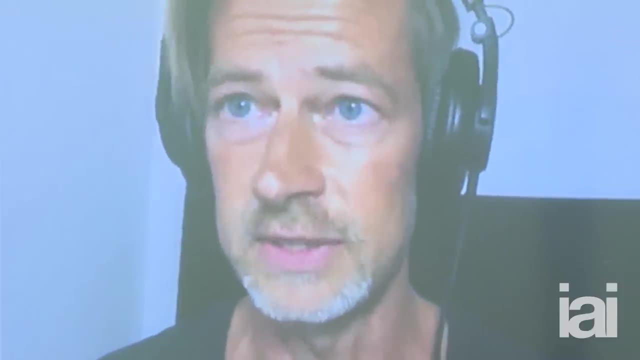 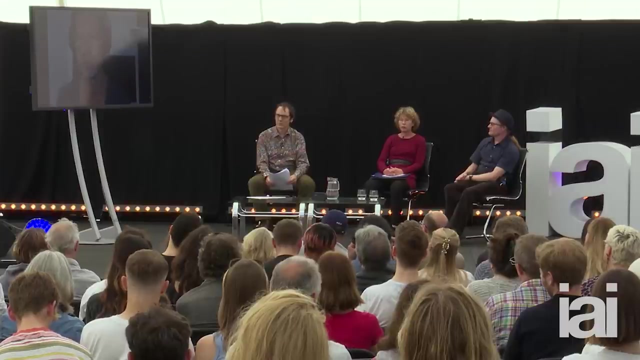 struggles to make sense of and fit some of these observations that we're making, But the model itself is so entrenched that very few cosmologists would want to seriously reconsider it, And reconsidering it is very hard work. So in a sense, physics and especially cosmology have become dependent or path dependent on. 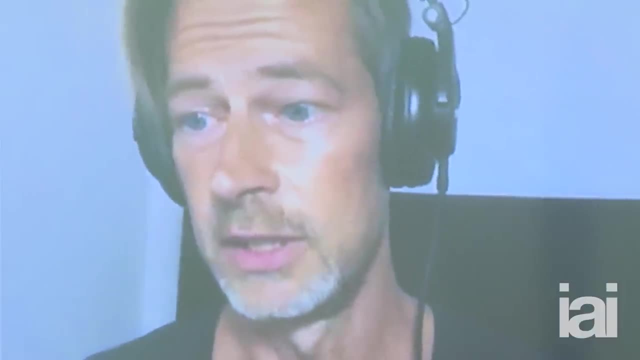 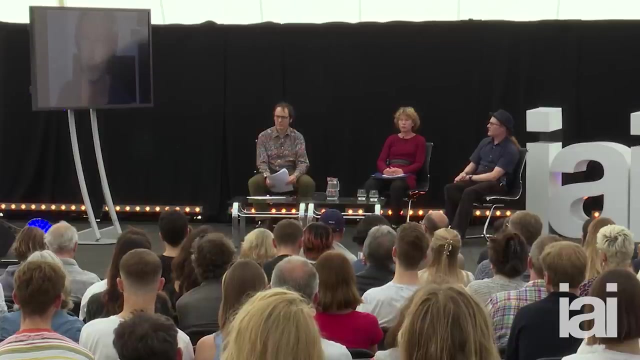 the Standard Model is how I view the situation. So it is, in practice, the one and only model, And some would claim that this is because it's simply because it's right. Maybe, more modestly, you could say it's because it's the best one we have. 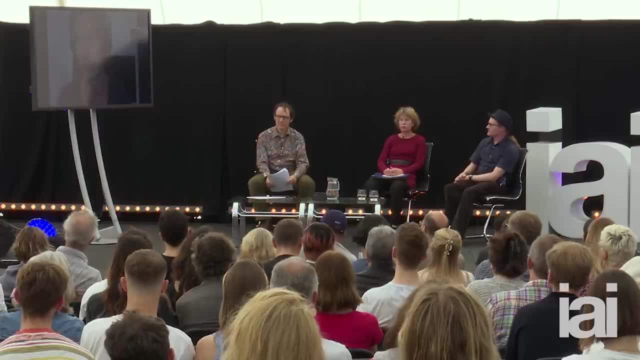 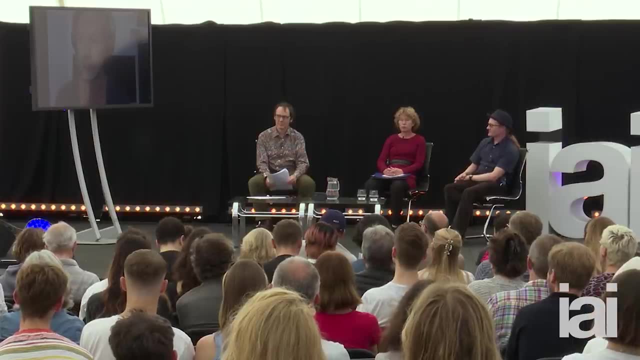 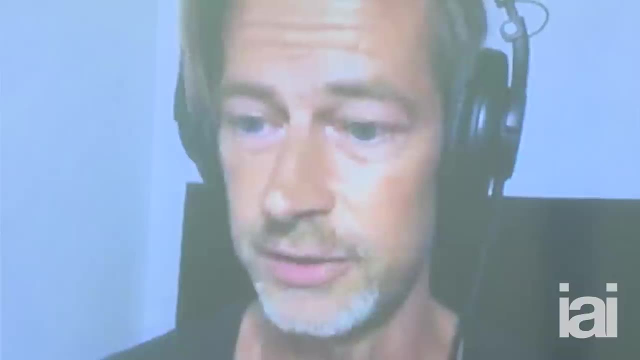 I'd like to argue instead that it's become too late to fail. The reality is, it would take enormous funding and work to develop an alternative theory that could explain all our observations better than a model that has been put to operative use for more than half a century. 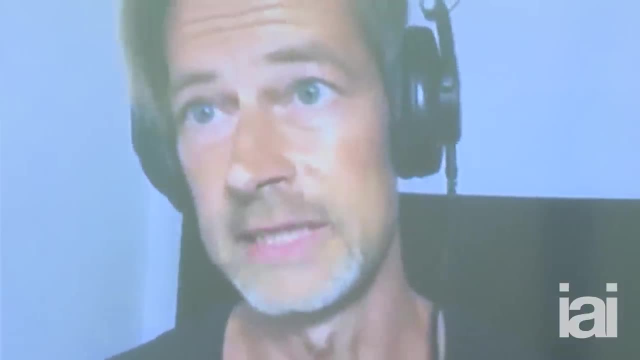 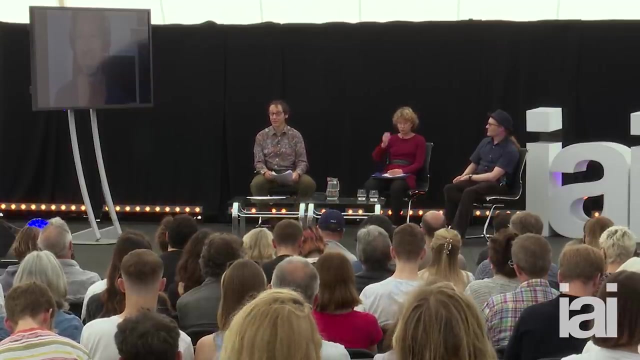 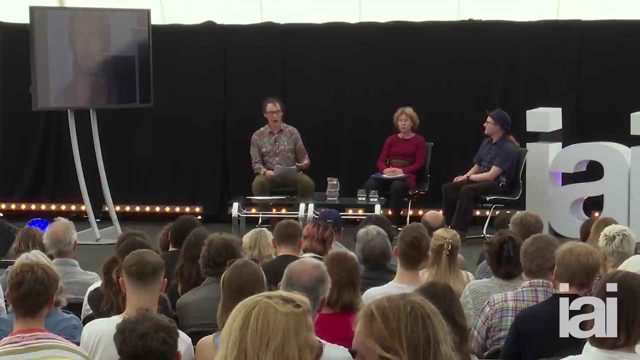 And without all that collective work, there will never really be a paradigm shift. Okay, thank you, Bjorn. Well, maybe we'll get on to what such an alternative theory might look like Later on. I think I want to start off the general discussion by thinking about where we are at the moment. 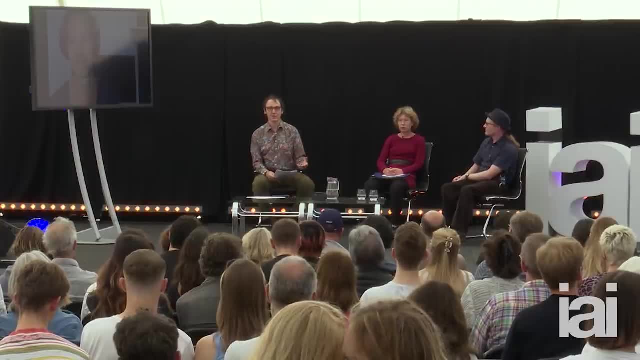 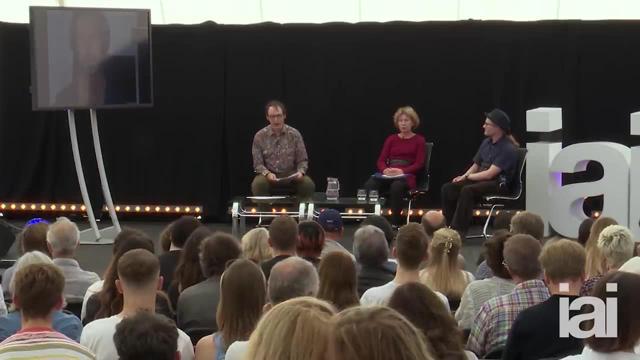 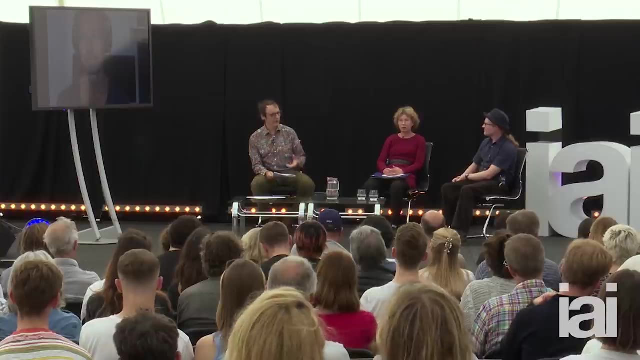 and how we got here, Because one often hears talk about a crisis in physics, or at least in fundamental physics, in particle physics, And I wonder whether that's actually true and if so, why is that the case? Why is it that we have this model that we know does a very good job of a lot of things? 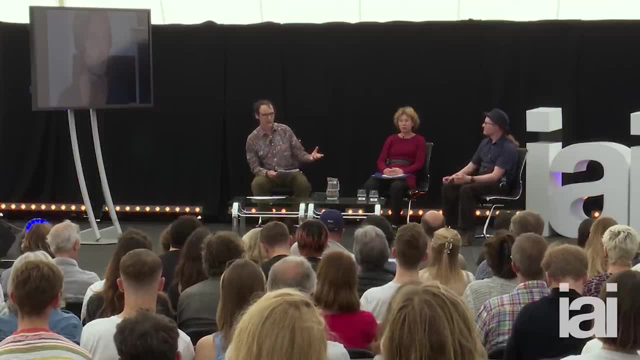 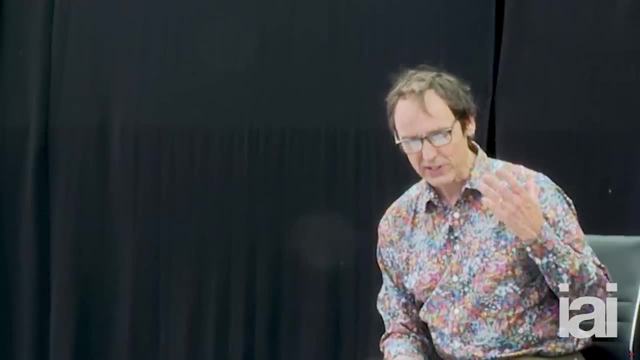 but we know that it can't be the final word, As I think you've all said, And yet we're struggling to make progress on that. It seems that it's proved incredibly difficult to find any hint of how we develop it, where we go from here. 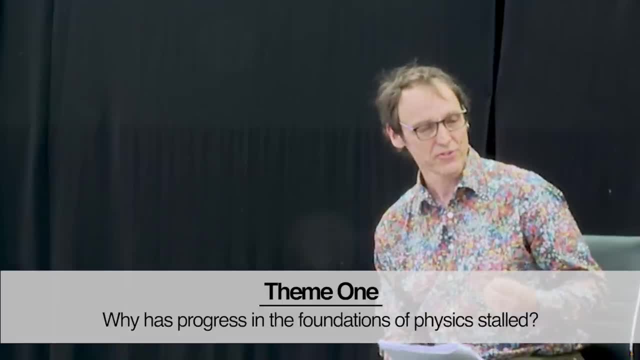 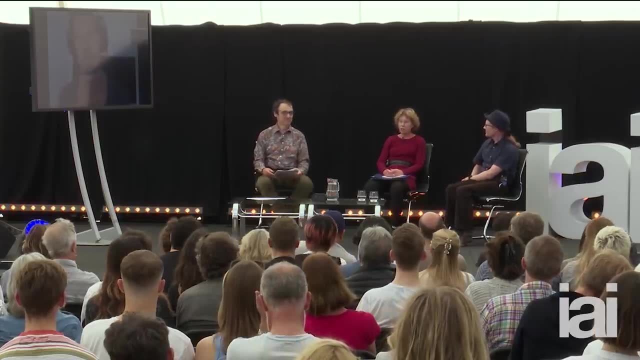 So why has the progress in these fundamental questions of physics seemed? why does it seem to have stalled recently? Sabine, if you could talk about that first of all, Sure, Before I answer your question, though, for the benefit of the audience, I want to explain. 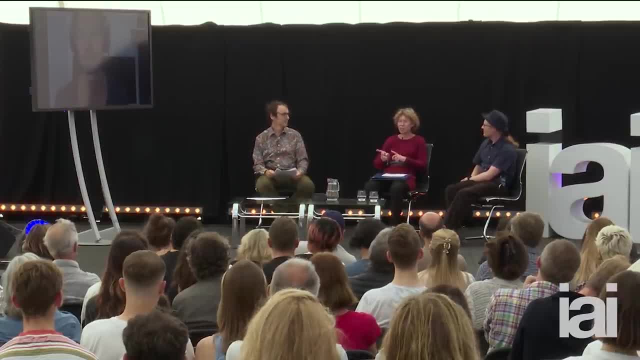 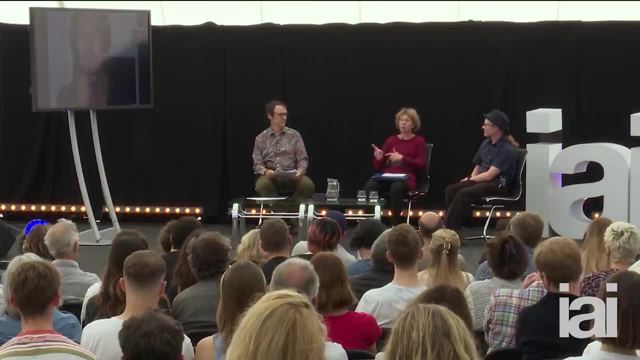 that There are two different standard models. There's the standard model of particle physics, which I believe is what we were talking about, And what Björn was talking about is the standard model of cosmology, which is based on Einstein's theory of general relativity. 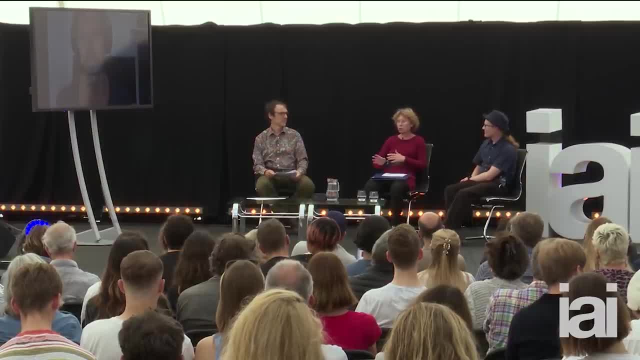 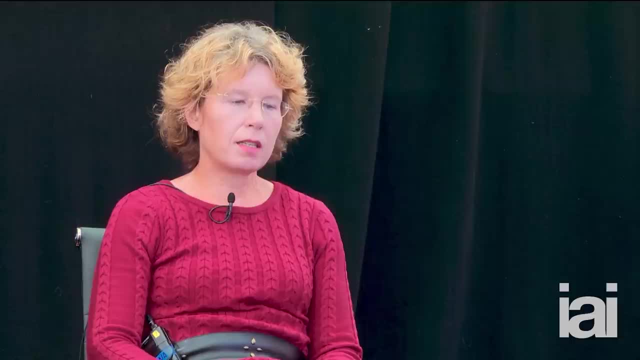 That's kind of a different thing. It's more commonly called the concordance model or lambda CDM, So just you don't get confused. So yes, about your question like what's going on, why we're not making progress. I think it's a combination of two things. The one thing is- I guess that's the obvious thing to say- the easy things have been done, like a hundred years ago, and as scientific discipline becomes more mature it becomes more difficult to see new things. 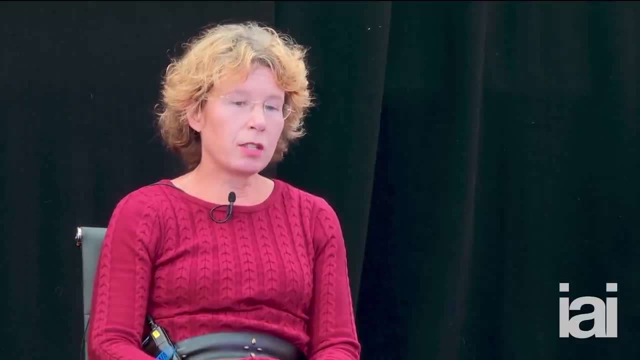 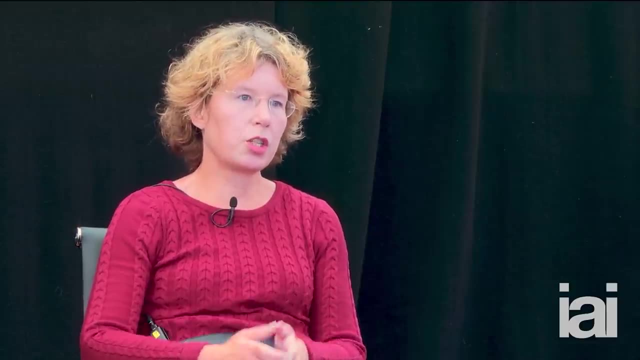 And so it just takes more time. But I also think that physicists have not been as careful in thinking about what they're doing as they should have been, So it's on the one side There's a problem. There's a problem with theory development. 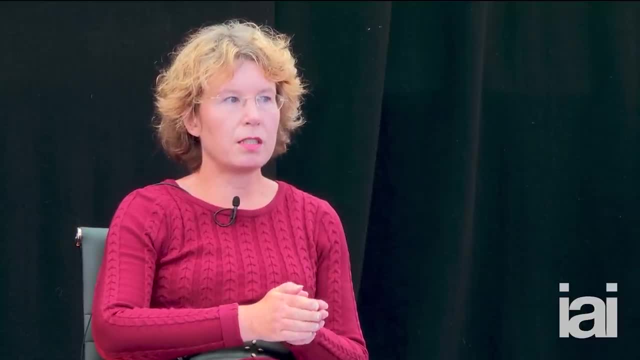 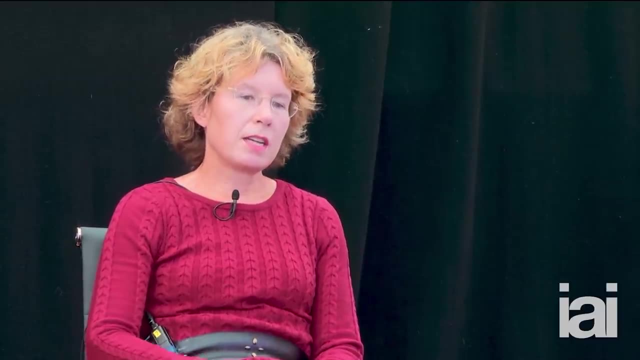 After the completion of the standard model in the 1970s, physicists were really, really convinced that symmetries are great and you can use symmetries for everything, And this is why they constructed a whole new bunch of theories based on symmetry principles. 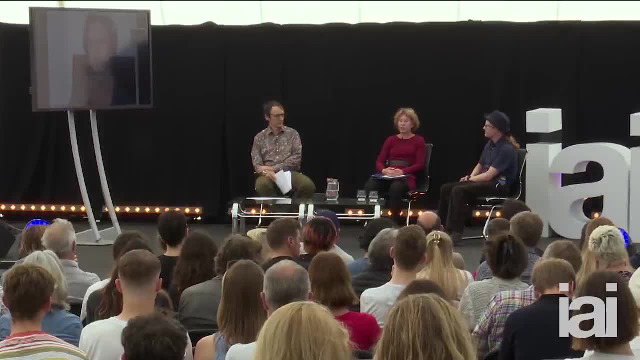 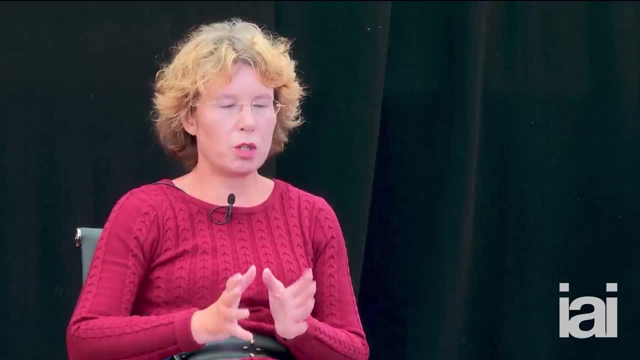 grand unified theory, supersymmetry, as the name already says, And they looked for evidence for them and didn't find it. And now I think you know we're in the middle of a new era. I think that the idea that they tried it was all well and fine, but at some point they 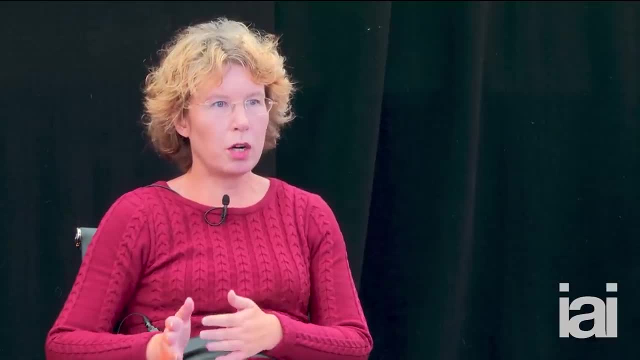 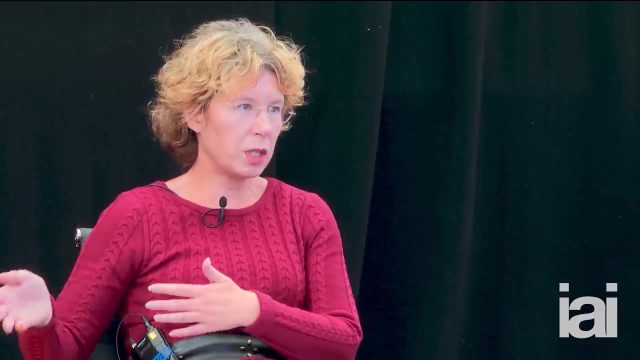 should have learned the lesson, because they tried it. It didn't work, but they never learned it, And so they just continued doing the same thing over and, over and over again and built bigger and bigger detectors, and they keep not finding something new. 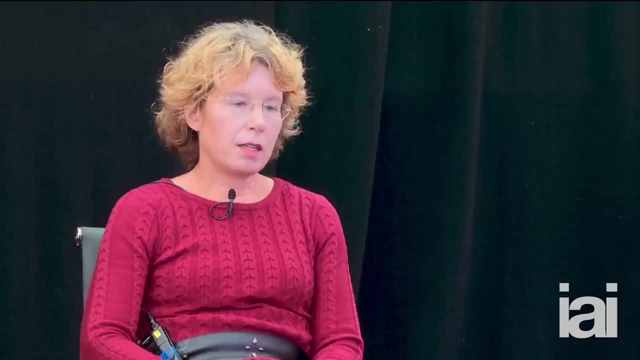 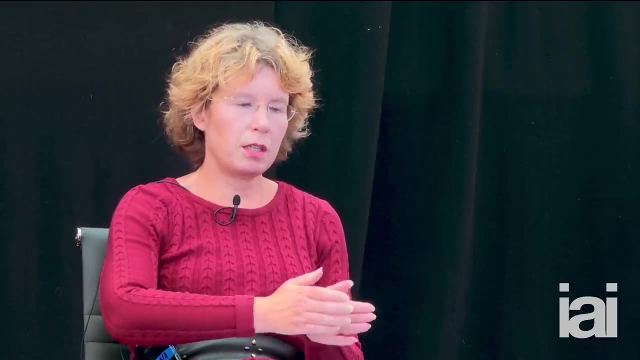 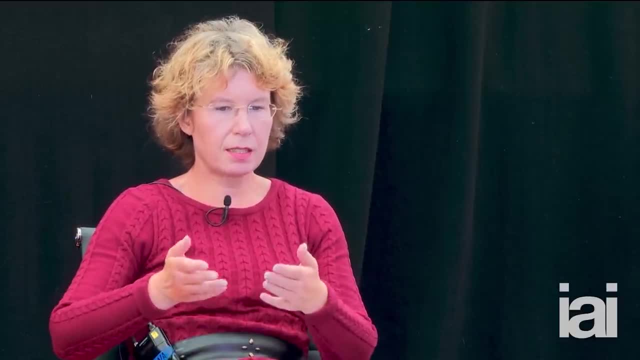 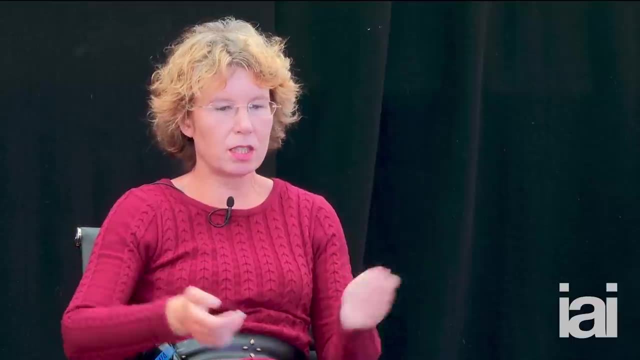 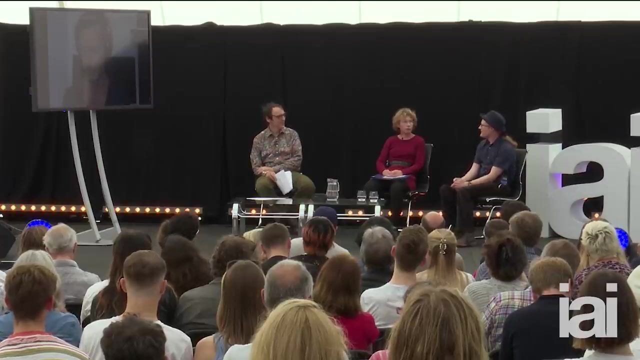 And so if we have theoreticians not being careful enough thinking about what might be the next prediction to look for, then we build experiments that don't find anything, And so we just, you know, continue to not make any progress. Well, Sam, you're involved in some of those experiments, so what's your perspective? 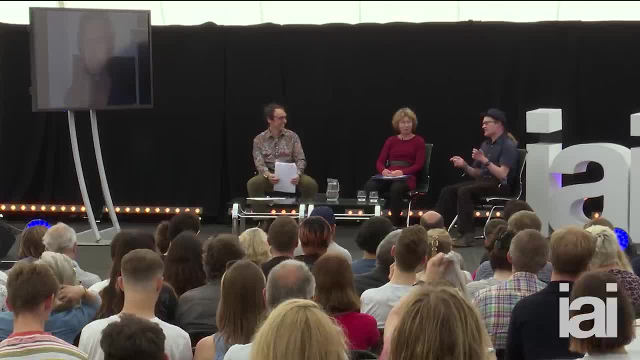 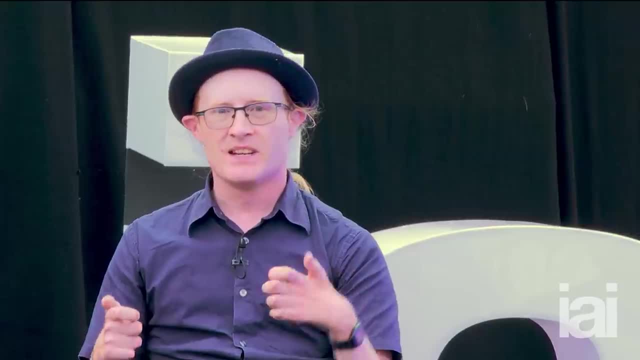 on this question. Yeah well, first of all I'd like to say that progress hasn't completely stalled. It's just not going as fast as we like and maybe we're not seeing the kind of progress that we really want. But in experimental particle physics, you know, we are doing things. 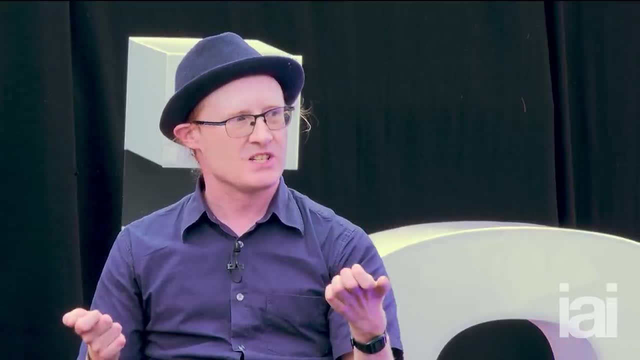 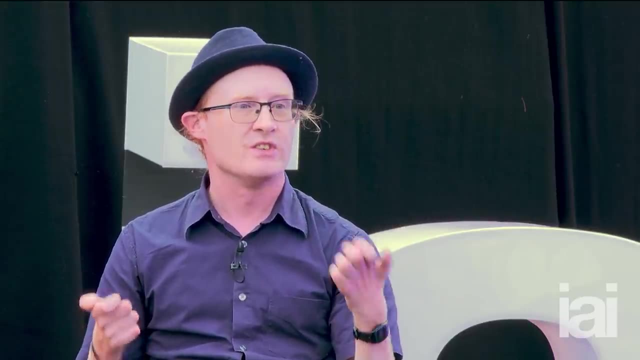 Ten years ago we didn't know that the Higgs boson existed. We've now done precision measurements of its properties- Well, maybe not precision measurements, but measurements of its properties and of the particles it decays into- and we're using it as a tool to search for new particles. 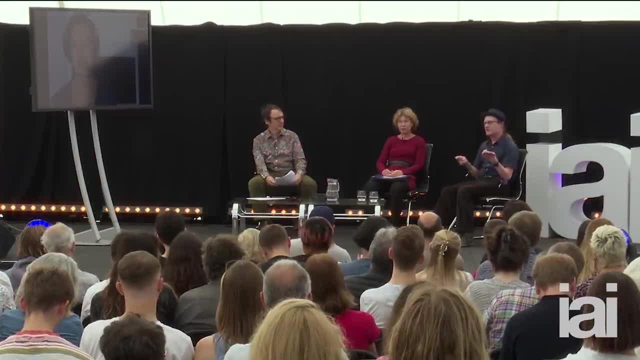 I guess also we're doing a lot of searches and we're getting a lot of null results, searching for new particles and effects, but we don't see them. And null results are not as sexy as discoveries, but they're still an important part of the 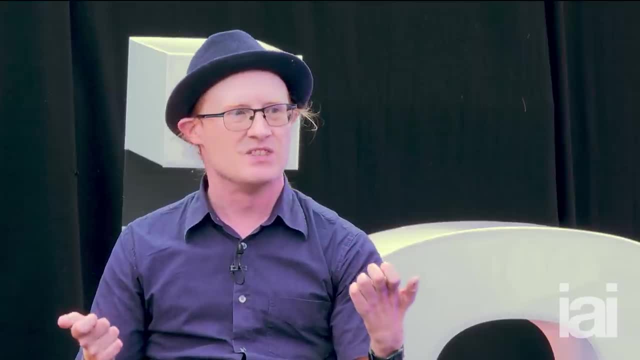 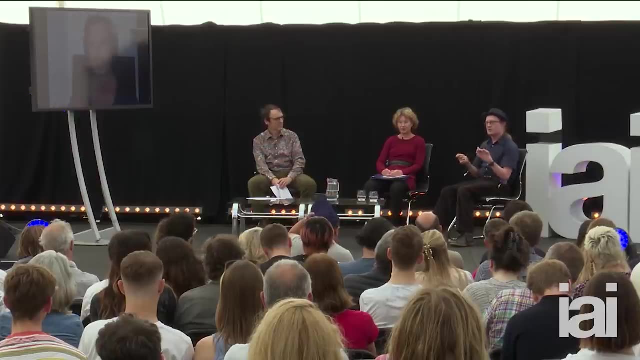 scientific progress, And so let's not dismiss the effort of these teams. you know They're not going to win a Nobel Prize, but these students do deserve their PhDs. But I think, as Sabina said, it's true that we've now reached a point where I think there's 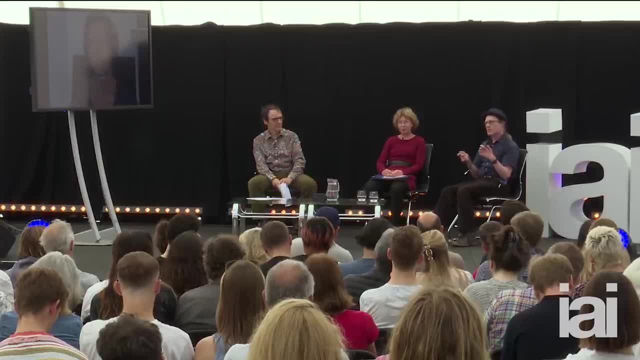 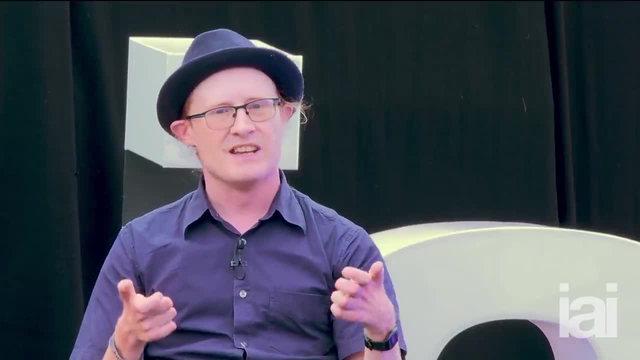 a bit of a disconnect between the theory and the experiments. One of the problems is that the theory is so far ahead of the experiments because by the time we reach a point where we've built a new bit of apparatus, it now takes so long. 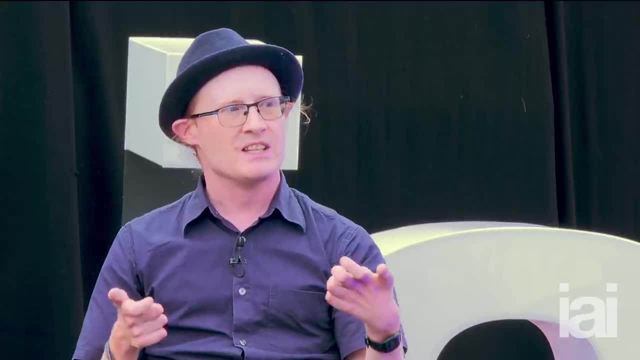 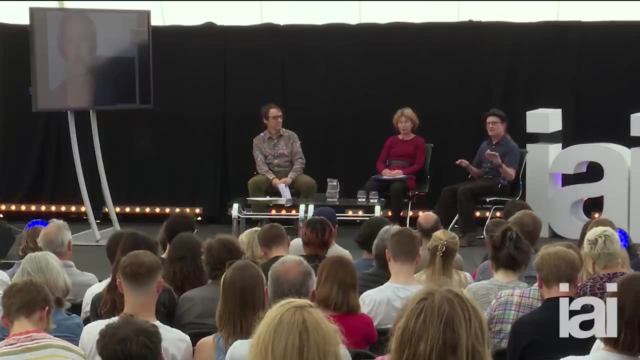 to build these accelerators. the theory has moved on, So we find the experiments we're doing were built- the design was chosen based on the theory 30 years ago, Which is obviously not the best way to do things, And I don't really see an easy solution to this, because these experiments are now very 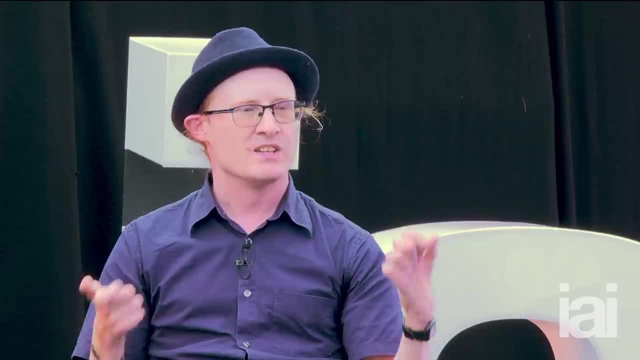 difficult and they need huge collaborations to do it. Now, even the smallest particle physics experiments are several hundred scientists And these collaborations, they take a lot of time to put together and to build the projects. Everything is getting more complicated and the next upgrade of detectors at a Large Hadron 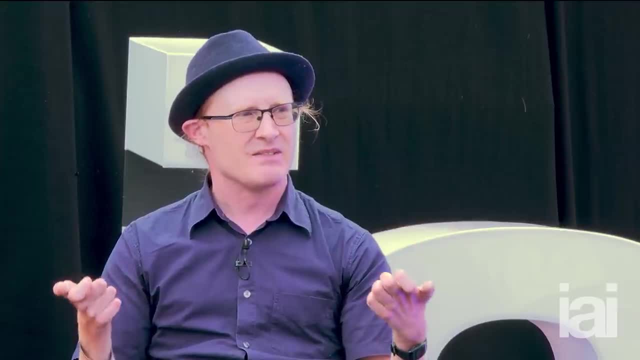 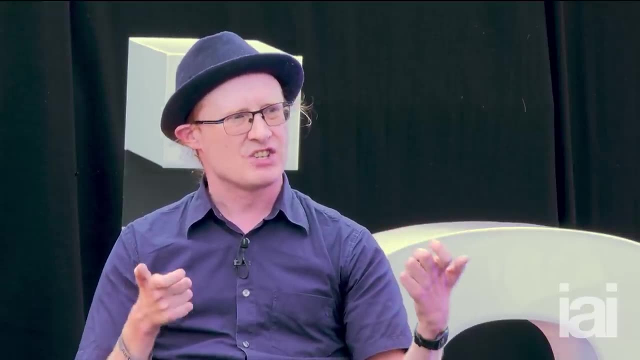 Collider, we could be seeing a hundred protons colliding at the same time. That leads to over a thousand particles And you have to keep track of every one to micrometer precision, just to have a chance of identifying the signature as something new. 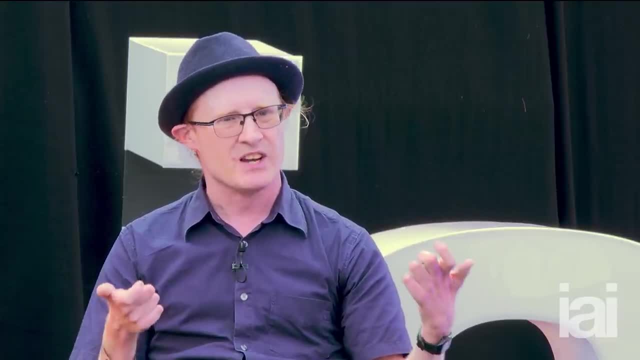 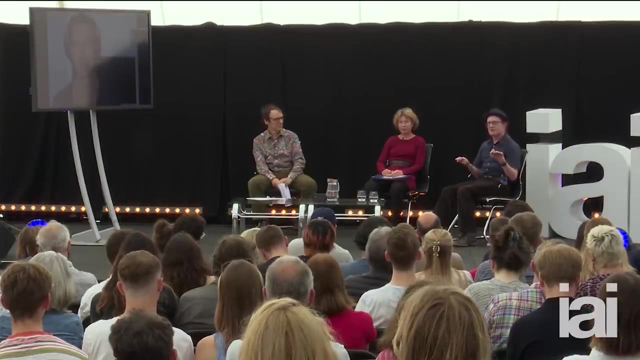 So even the small sub-detectors of your component have teams of a hundred people working on it. So yeah, it's going to be a lot more challenging and I don't really have a solution to this. I think maybe we do need to rethink about the connection between experimental physics. 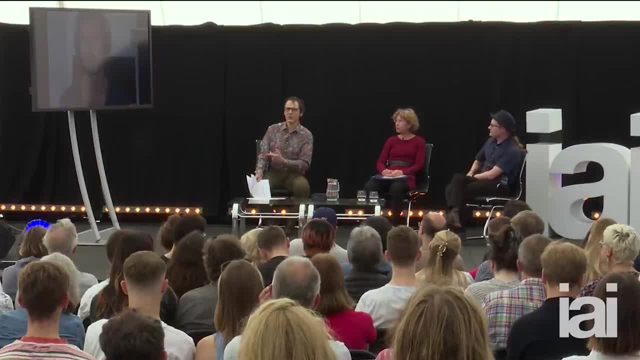 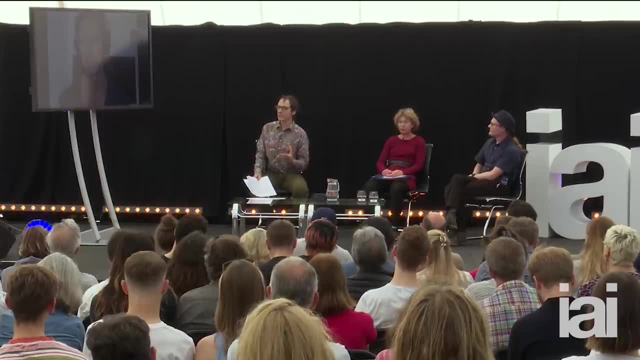 and theoretical physics. Well, that touches, Bjorn, on the issue that you raised about path dependence, Because you know what Sam has said is that purely by the nature of these experiments, by the nature of this big science that is involved, one has to commit almost to 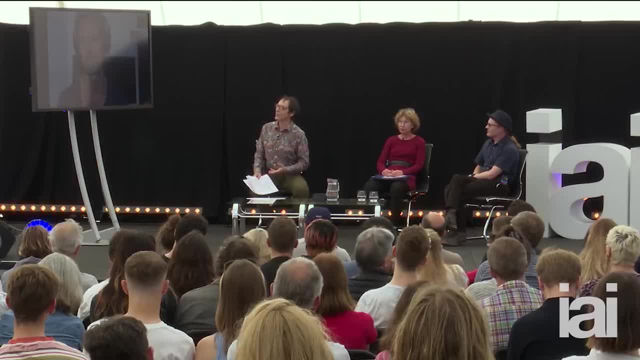 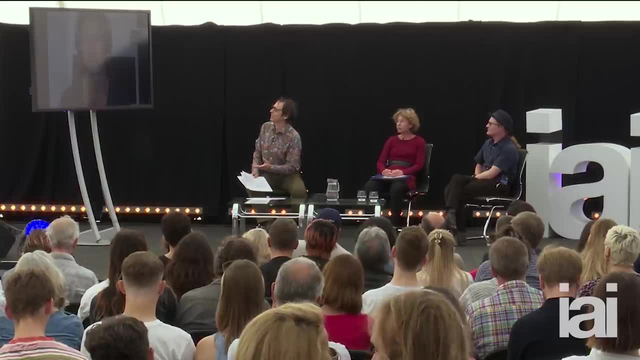 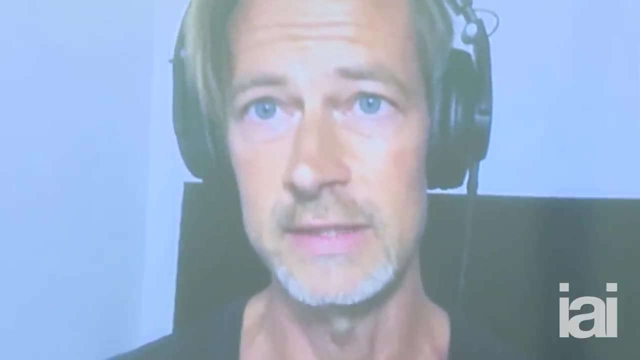 a theoretical position, perhaps decades in advance of having the experiments to test it. Is there, from the point of view of a philosopher of science, is there a problem in that way of doing science? Well, there is a general problem for the development of the sciences, like of physics. 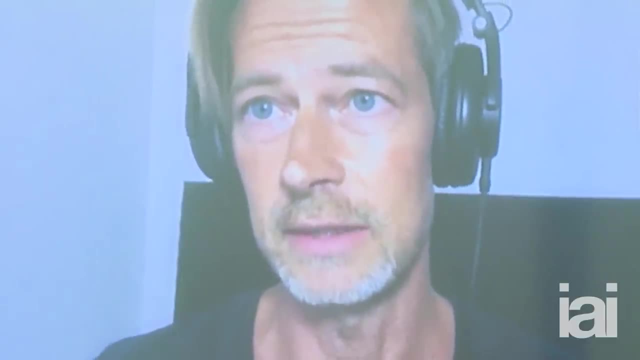 and cosmology. This is part of the historical picture. It comes up against certain limits, that there are fundamental limits. You know, the history of science is this amazing trajectory of how we are able to measure and expand our knowledge within the universe. 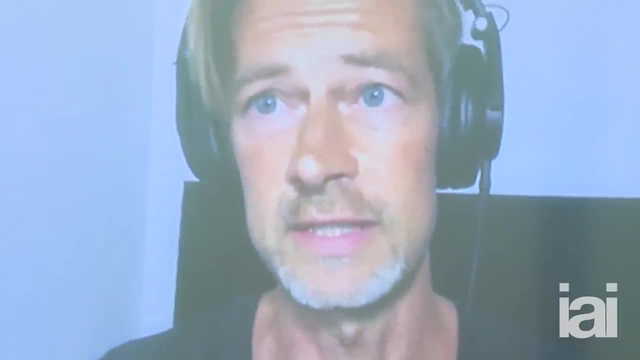 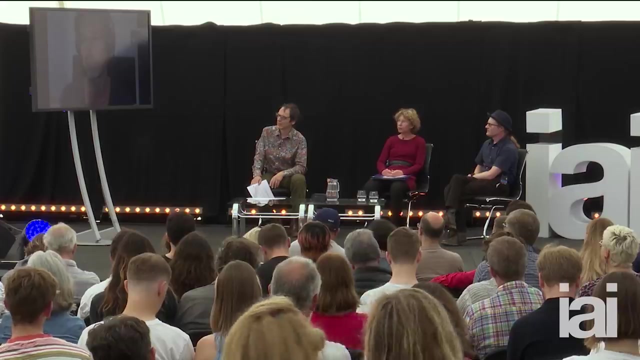 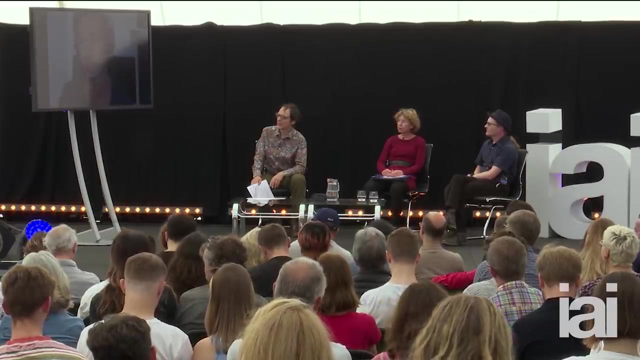 But there are fundamental limits that are always that the history is about surpassing, And I think what both Sabina and Sam are pointing to is that progress seemingly stalls because we have this idealist notion of progress from a century ago, And it's harder and harder to get further into nature, whether we're looking in the 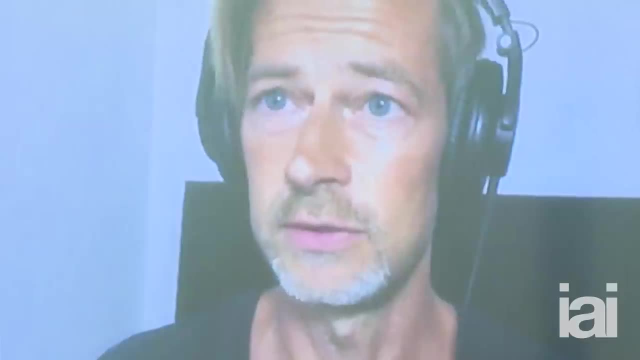 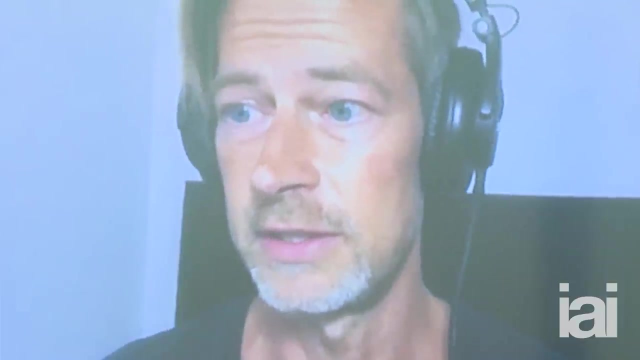 micro-physical scale or further out into the universe. So in this perspective too, I want to point out that the situation in cosmology is a little bit different from particle physics in that, like physics and the micro-scale, you can do experiments under controlled conditions, as Sam is pointing out. 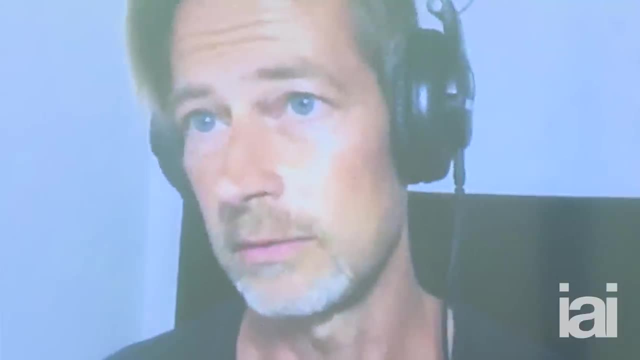 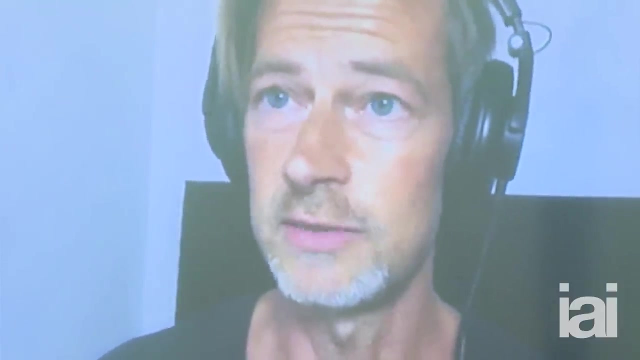 In the macro-physical universe as we know it, we don't, we can't do repeated experiments the same way, And we're talking about a scale here that is 20 orders of magnitude higher than the scale of particle physics. So this leads to certain kinds of problems just with basically how confident we can be. 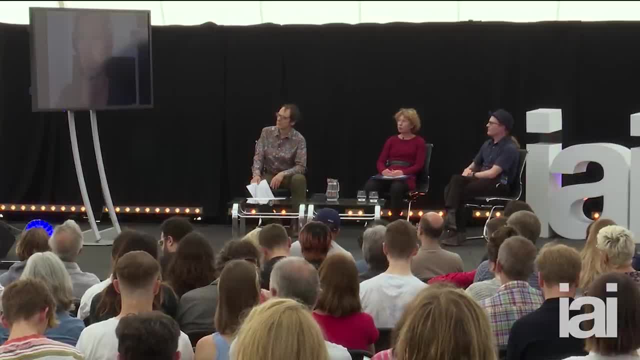 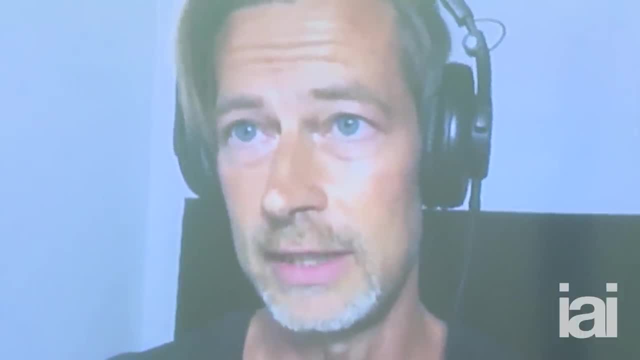 in our own measurements about the scale itself and so on. So I think it's important to keep in mind that, with this subject matter, whether we're looking inwards, to the inner part of particle physics, or outward in the universe, it's important. 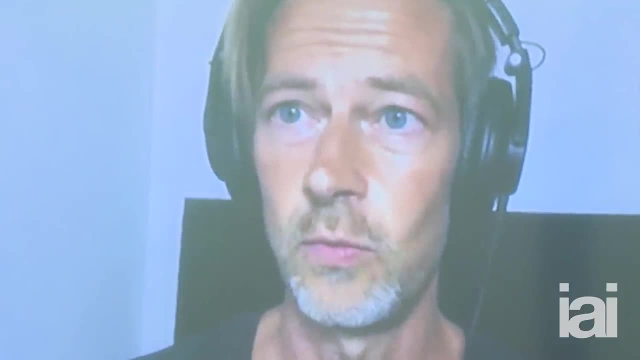 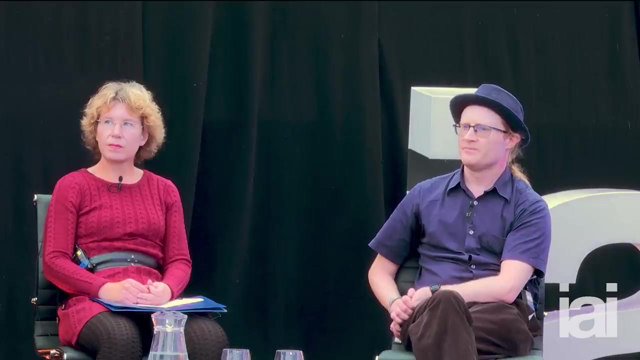 to keep that in mind. So the number of different aspects. part of the interesting aspect that I think is so important to think about in cosmology is how do we measure the scale of the universe, and then this insight we've been trying to derive is really important. 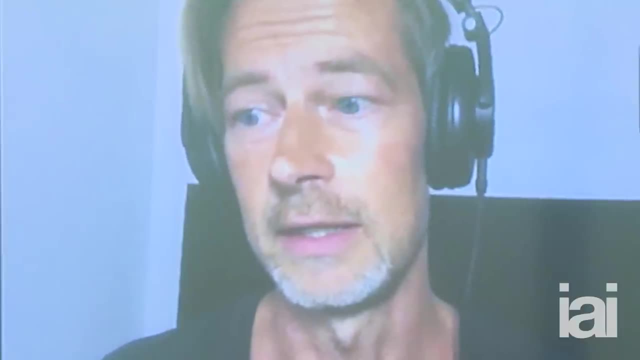 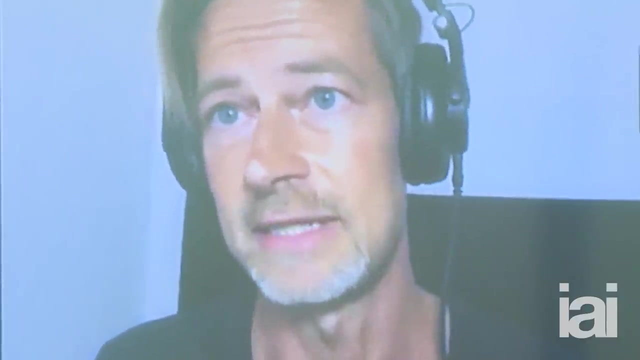 This is something that the researchers have done. This is something that we've been doing for a long time now And it is a very interesting fact And, yeah, I hope it's something you've been up and basing from one analysis now. and I hope you had a good time. I do. Thanks man, Thanks guys. Thanks Sam. Thanks Sam. Thanks for the interview. I'll just say thank you, Thanks Sam, Thanks Sam, Thanks Sam. 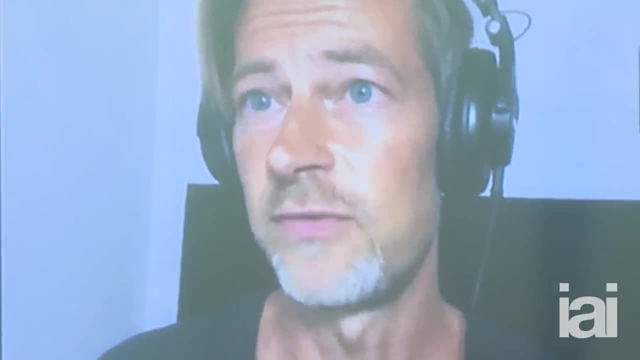 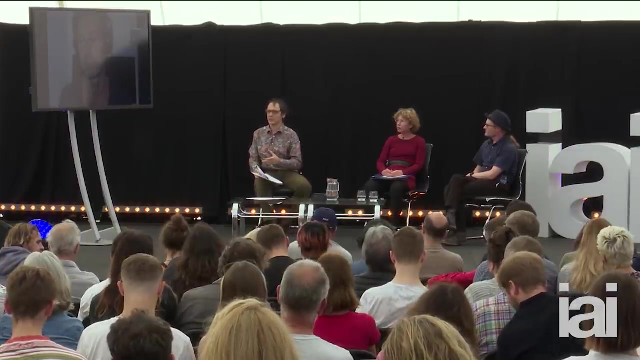 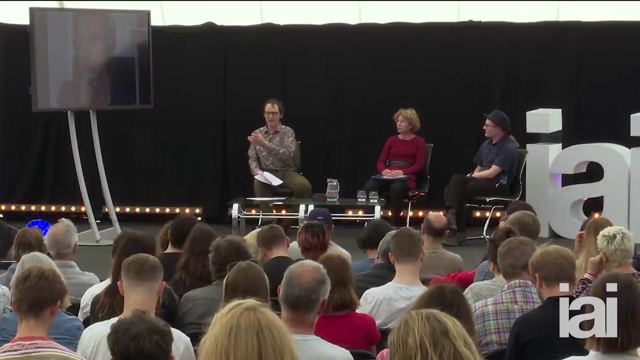 work, but yes, it is. um, there are some fundamental problems here. i mean, it sounds as though perhaps some of the problem is that the understanding of this area is advancing on these two fronts that are quite, in some ways, quite distinct. that, as you know, as you say, uh, you can turn a telescope. 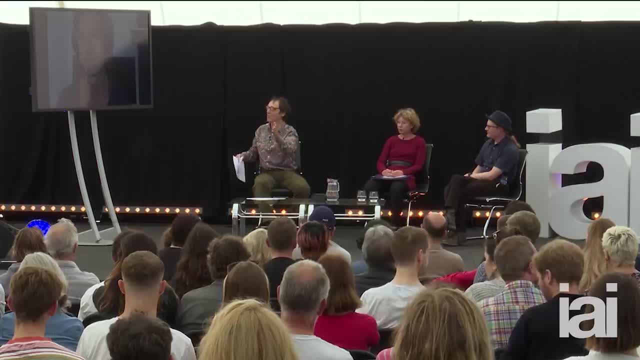 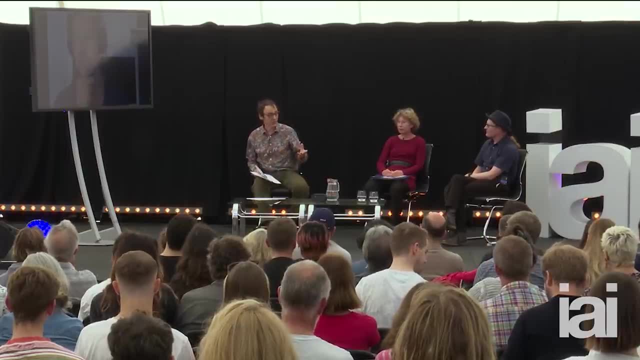 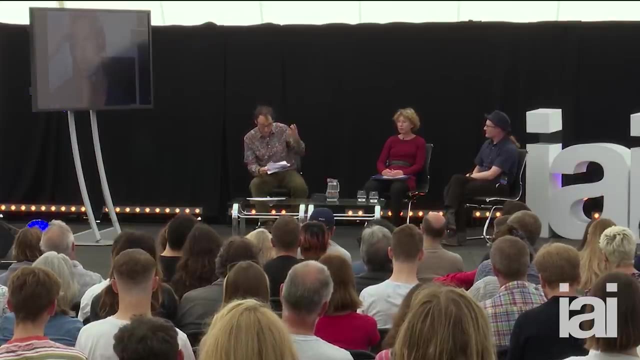 onto a certain object in the sky and make an observation tomorrow, and, as we have found, those sorts of observations can fundamentally change the challenges that theorists and perhaps even experimentalists have to face. so you know, no one was necessarily. i mean, we've known about dark energy. uh, we've known about dark matter for some time now. um, but you know, that came out of. 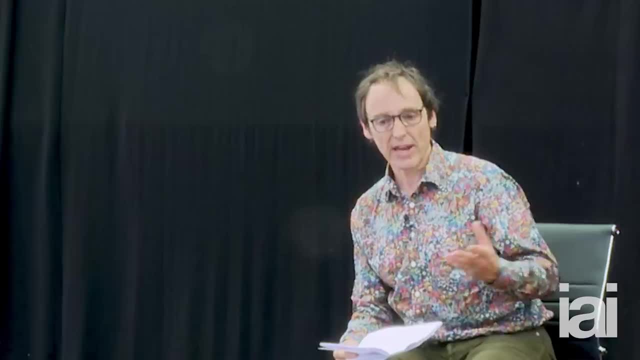 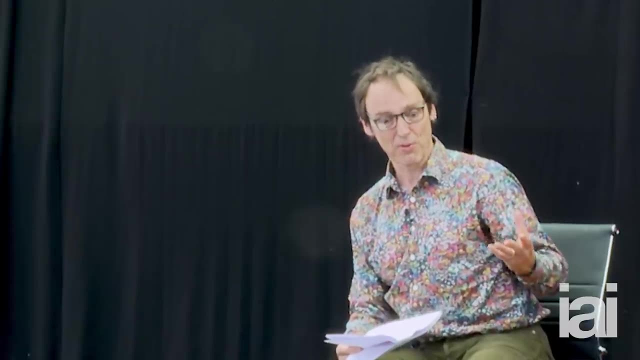 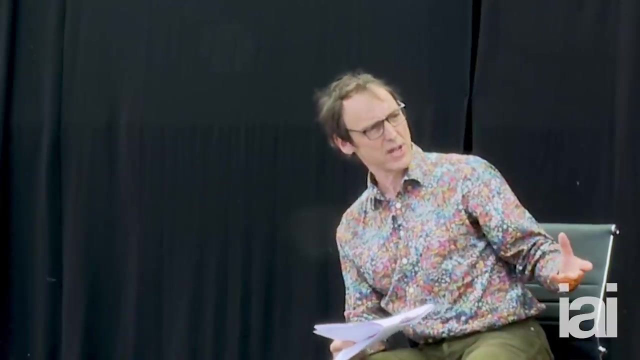 observations rather than any theoretical motivation. dark energy came as a surprise, uh, back in the 1990s, but you know it's confronted high energy physicists with a new problem, a quite you know deep, fundamental problem that wasn't originally on their agenda, i guess. i mean, does that create problems that actually astrophysicists and 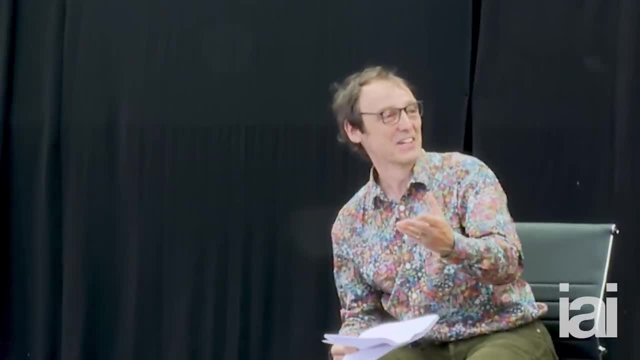 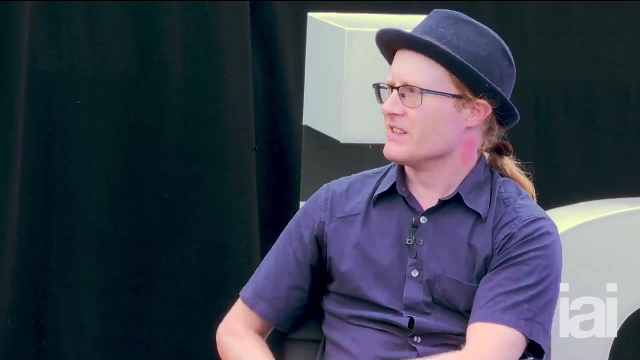 cosmologists can create problems for you overnight, you know, whereas you've already sort of launched on a particular program of experimentation. i think that's? yeah, that's certainly true. that can be a problem. and, um, maybe the problem is that one field of physics is often looking to another. 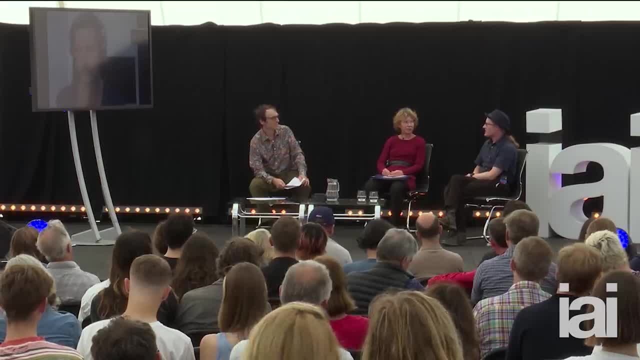 field of physics to solve their problems. so the astronomers are all convinced that dark matter exists and they're just waiting for us to find it. um, but of course, as sabina has said, there's many possible ways to solve it, and i think that's a good point. and i think that's a good point. 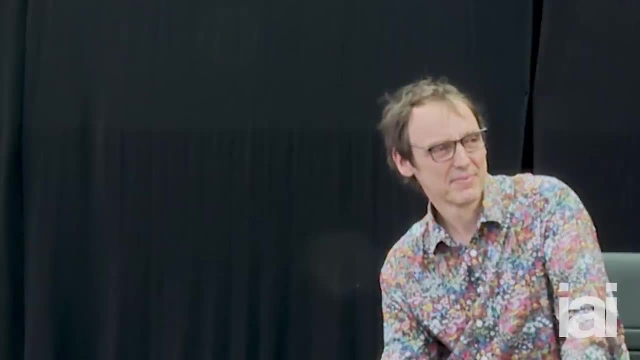 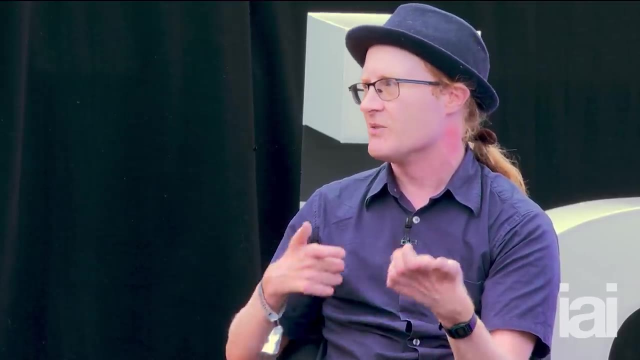 there's many ways of solving the dark matter problem and you know, new particles are one way, but there are also theories of new physics and, uh, new gravity, modifications to gravity, and uh, it seemed- uh, i can't keep track of all of the developments. in theory, it seems that, uh, these 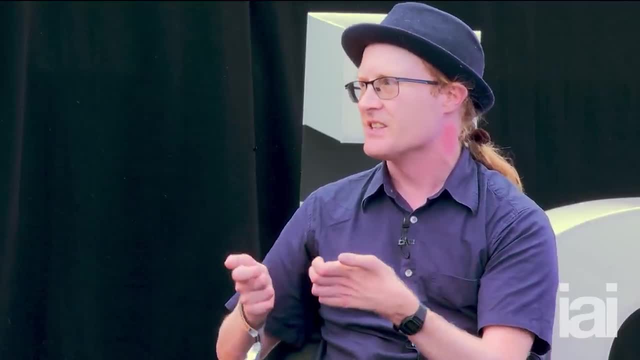 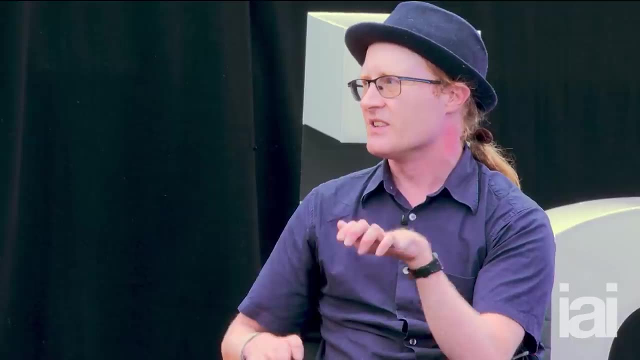 things go in and out of fashion. at one time everyone thought it was particle dark matter. now it seems that, uh, modified newtonian dynamics might be coming back into fashion. um, but, uh, but i think you know the astronomers, they don't they? they just seem to say right. 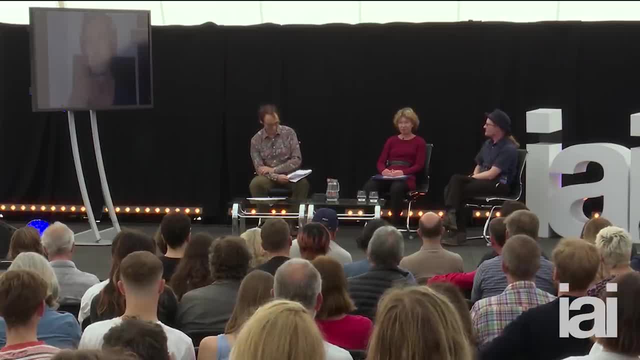 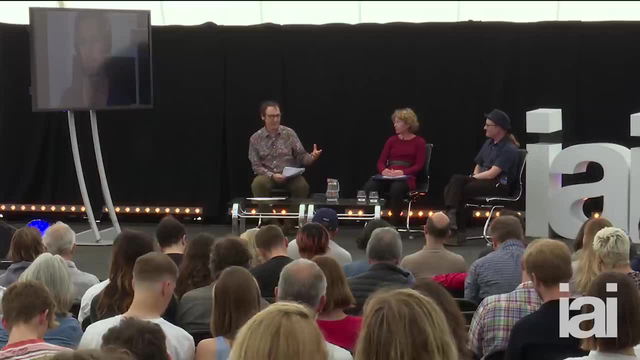 dark matter exists. we've shown it. you go find it right, okay? um well, there's more we could say about that, but i want to move on to the, to the next topic that we want to, which i think follows on quite naturally from that, uh, from that issue, which is really to. 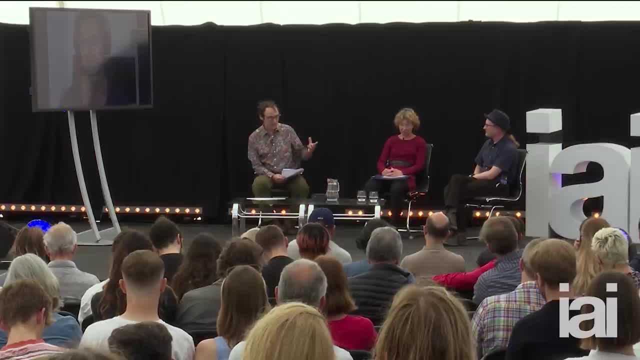 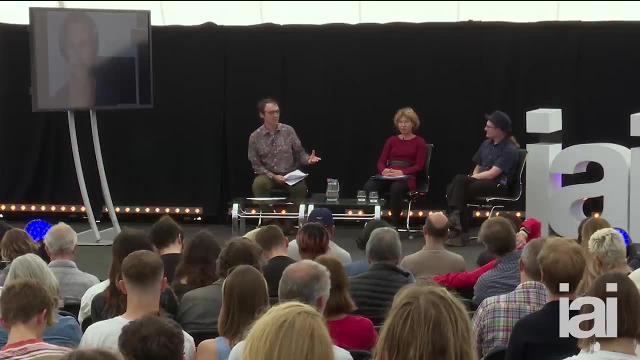 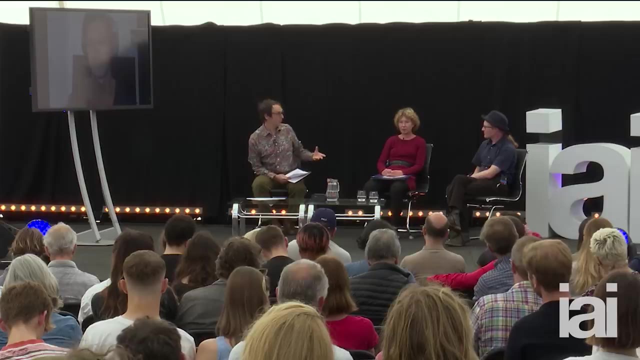 ask how serious, uh, this problem is. you know you? you said, sam, that um, perhaps, uh, we were too optimistic in what the large hadron collider would find, um, and so far it hasn't found, for example, any clear evidence of the idea of supersymmetry, which people were certainly hoping was going to be the next step. 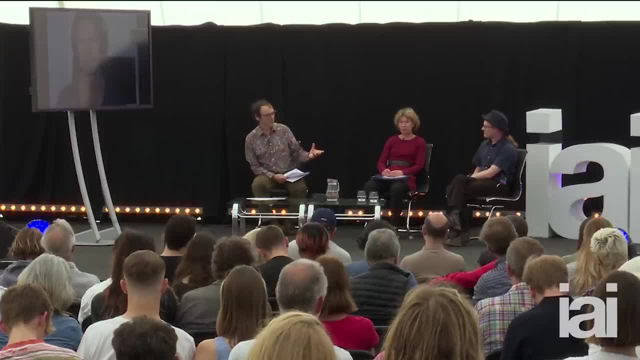 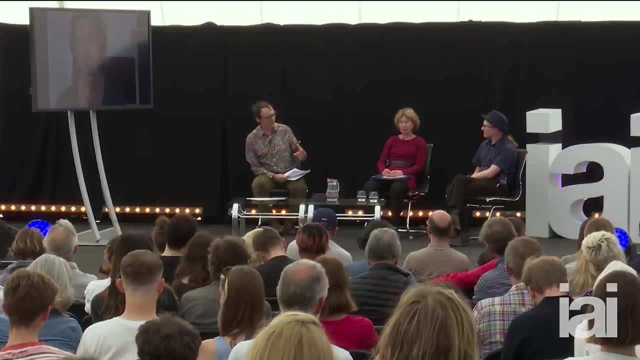 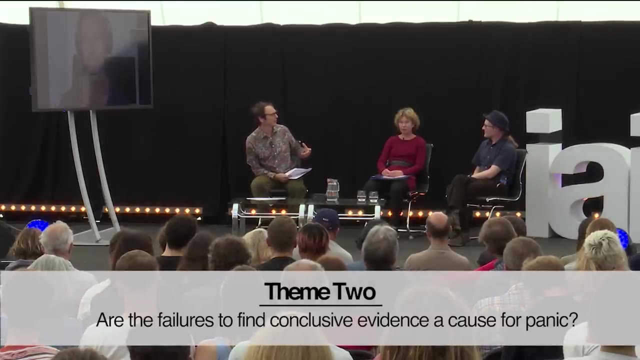 forward. so, uh, and now we have the muon g minus two. results that you say, you know, suggest that there may be something that we don't really understand. how serious are those problems? and in particular with, with supersymmetry, i mean, is it causing panic amongst you know? uh, particle. 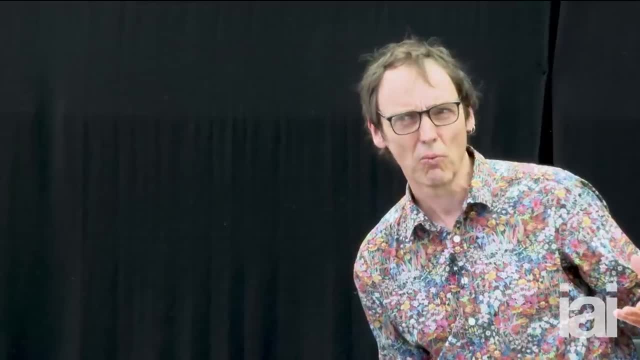 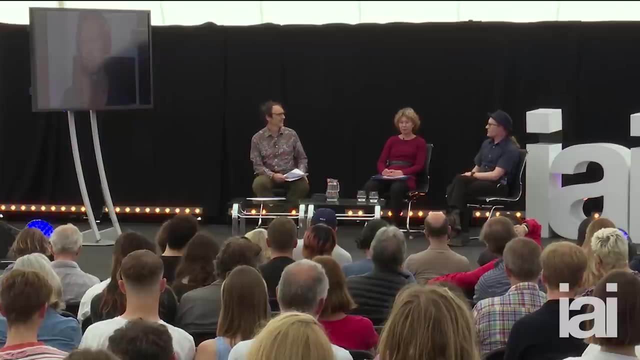 amongst theorists that there is no sign of it, or are they? is it? did they expect this to be an extremely hard thing to to detect? um well, maybe to first mention the, the anomaly we've seen, which is the, the muon g minus two, uh thing i mean. 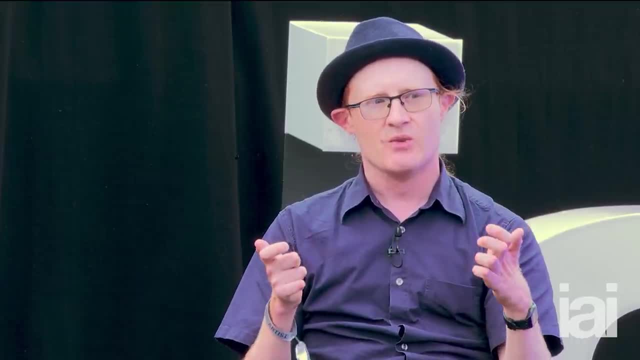 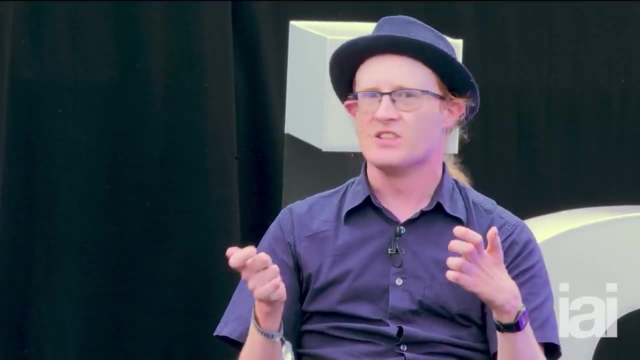 what this is showing us is that there's something that's interacting with the muon, but that's not in the standard model. and the muon is a great particle to study because it's it's heavy enough to be sensitive to new physics, but it also lives long enough that you can actually put it in beams, and 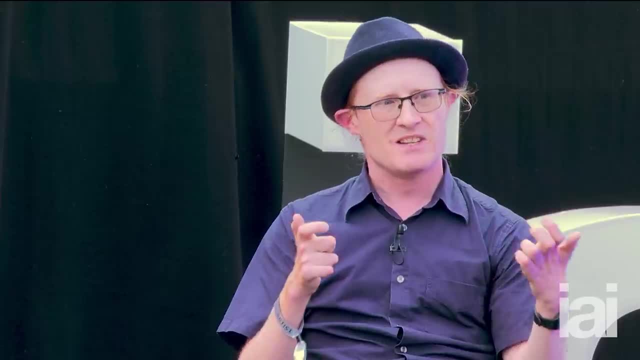 storage rings and actually study it properly. and uh, so there seems to be something that's either interacting with the muon or it could be interacting with something that's interacting with something that's interacting with the muon. it could be a second or higher order effect. 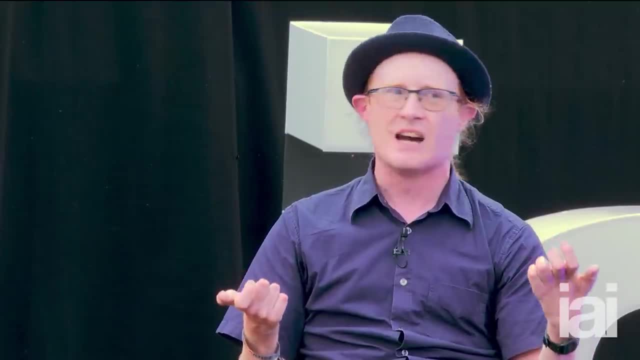 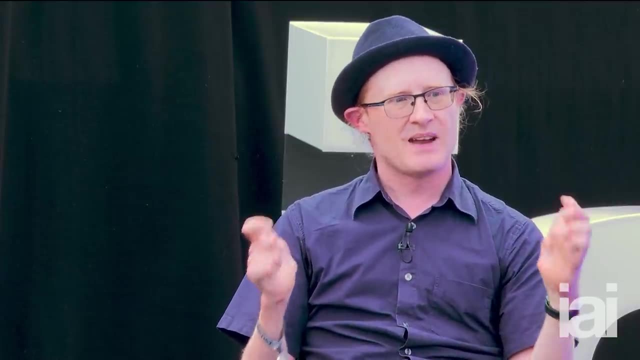 this could be a a new force, but really we don't know how it's best to describe it. it could be a new particle interacting by an existing force, or some variation of an existing force, and the muon g minus two experiment is a brilliant probe for searching for new physics, because it depends on so many. 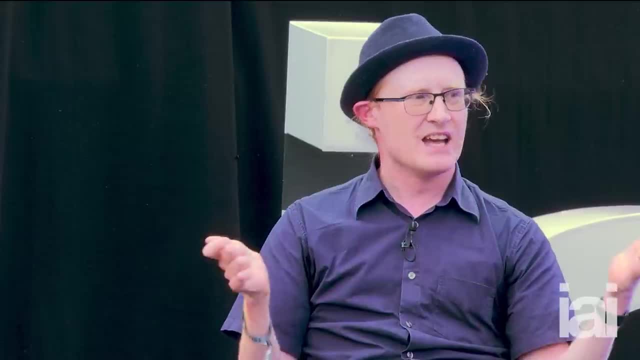 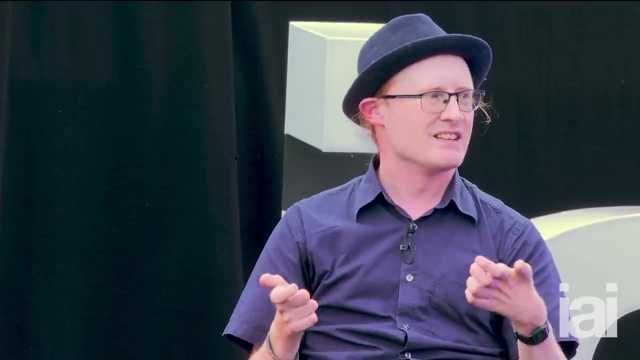 things, but this also means that, having observed it, we don't really know what it means. you know, there's so many possible theories that could explain it. supersymmetry was one, but then supersymmetry hasn't been seen at the the large hadron collider, so maybe we need to look at other. 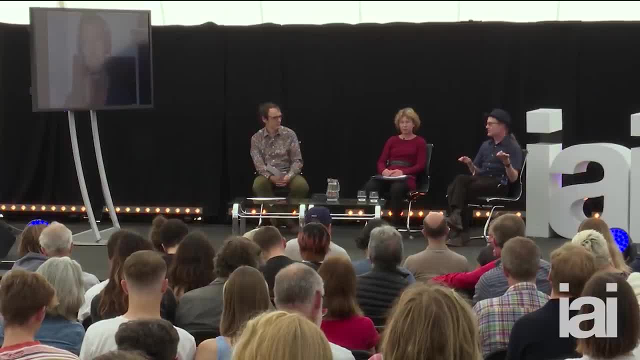 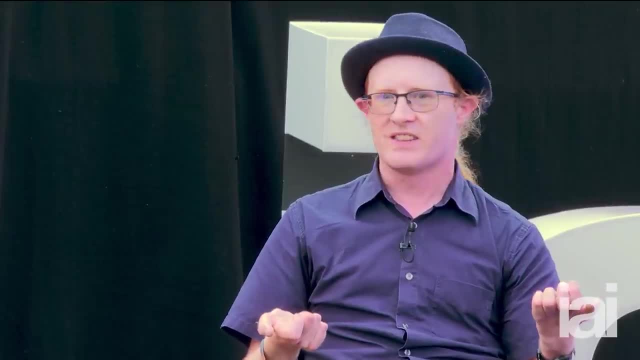 yeah, when you look at these other theories, what does it tell us? well, we know that the vanilla flavor of supersymmetry seems to be out, but maybe some alternative version of supersymmetry could still be correct. but there seem to be no shortage of other theories. collute-succline. 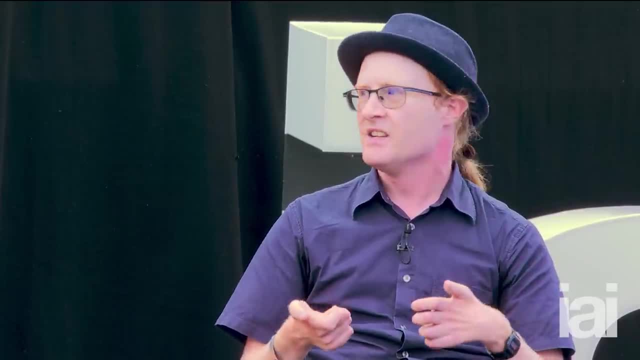 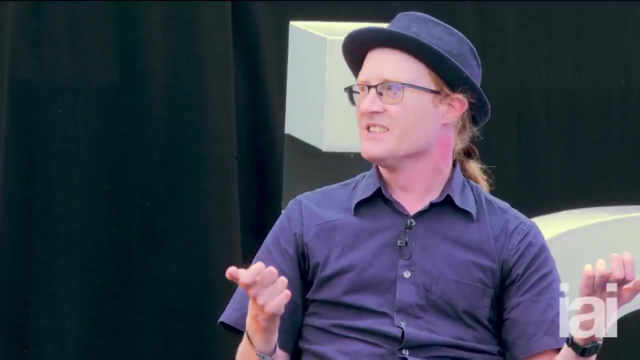 particles, extra dimensions, z, primes, lepto, quarks, uh, technicolor baryons that you know. there's so many theories that, as an experimentalist focusing on the hardware, i can't keep up with them all, so i just have to uh to listen to people like sabina to tell me which ones i should be paying. 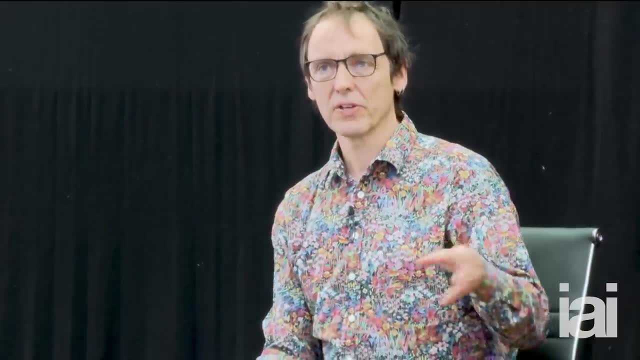 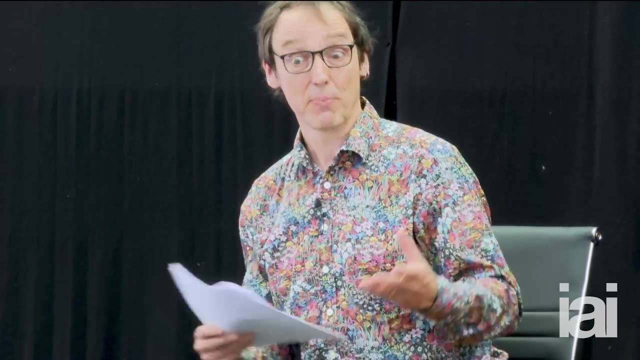 attention to. well, i was very struck by that, that how, once, as soon as i was able to understand, the results came out: um, the, uh, the, the physics, um community in the pre-print server where physicists post their papers, were flooded with theoretical explanations. you know so many that 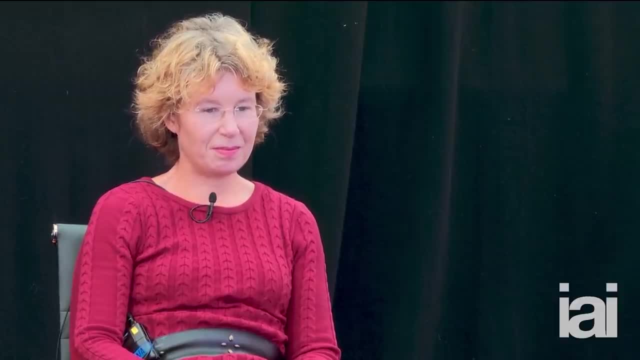 you, you, you kind of have to wonder how, how constrained at all is this problem if so many, um, theoretical explanations for something quite new can seemingly be cooked up almost overnight? um, i mean, sabina, maybe you can talk to that issue, you know? do we really know? 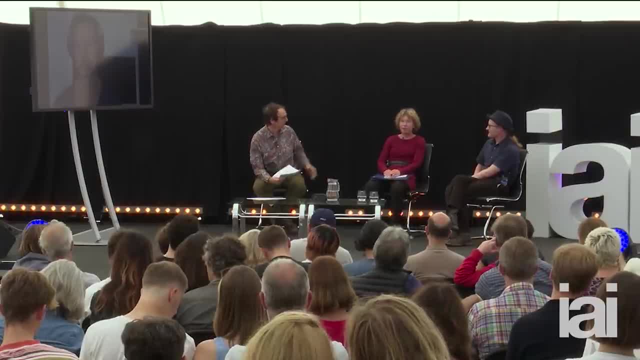 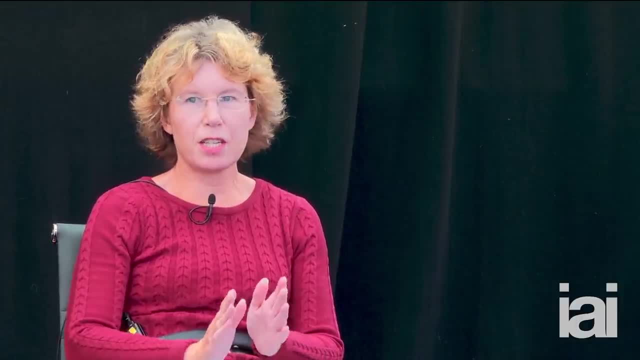 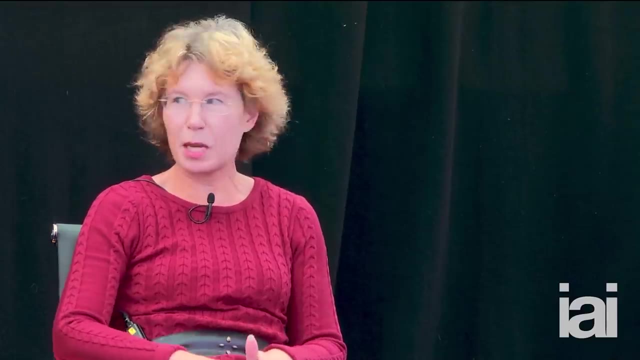 what the problem is, you know. is there too much room for maneuver? yeah, so that that's an excellent point, though i have to say, as it's often the case, uh, if there's a new result coming out, uh, there are a lot of people who already know it's coming, so they, they may not have written the papers overnight. 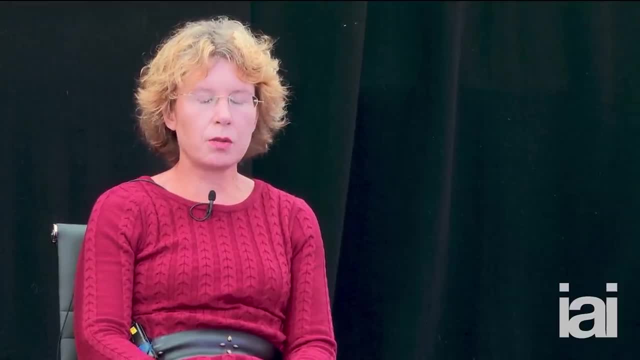 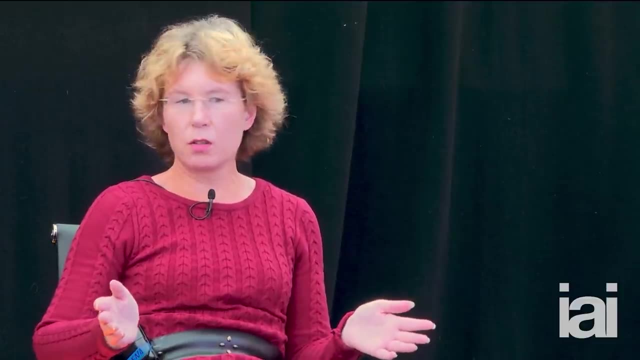 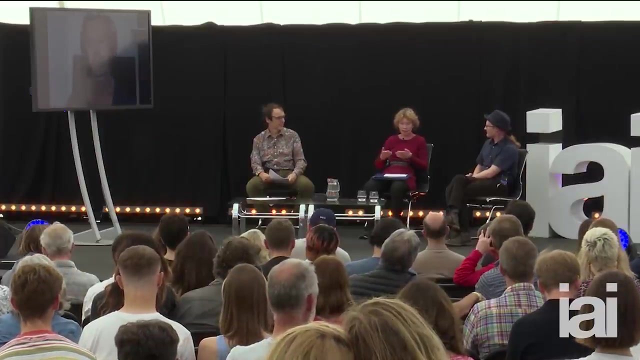 and they had some advanced uh warning. but it's certainly true, and- and that's exactly what i mean when i say we have a problem with theory development, when you can explain everything by your theoretical methods, uh then, since you were asking, you shouldn't pay any attention to those predictions. they're entirely. 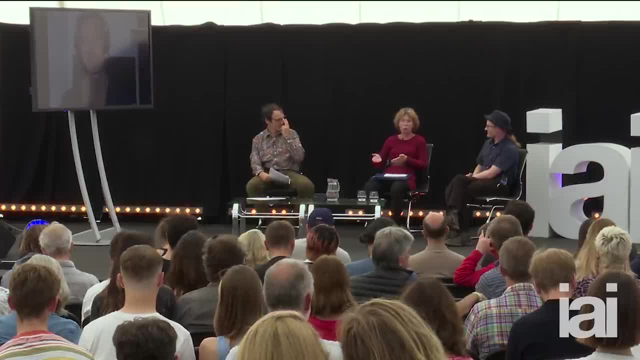 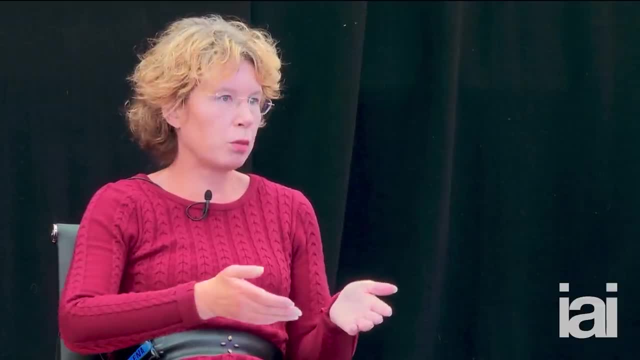 worthless, and that's what we see. that's why they're being ruled out over and over and over again. because you have all these theorists. they literally guess their models, because they like one particular particle, they like one particular symmetry, or they get obsessed with, you know, some. 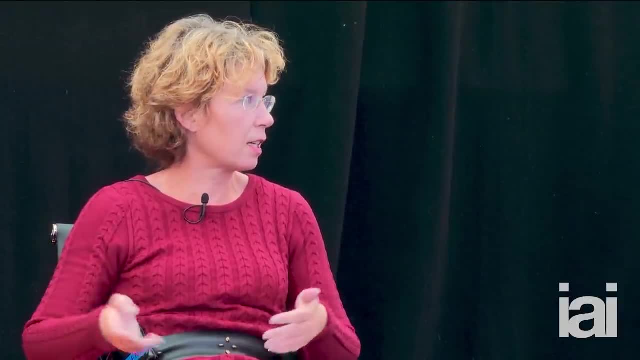 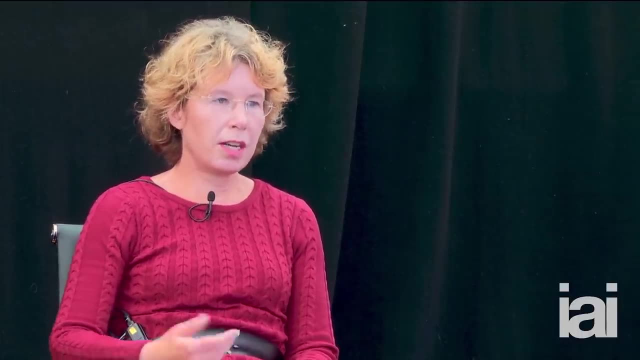 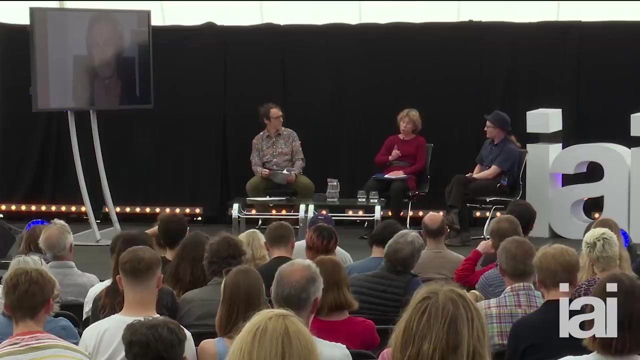 anomaly in astrophysics that's currently on vogue, and then the next year it's gone, and so on and so forth and it just leads nowhere. and i i really think that theoretical physicists they have to have a hard look at um their methods of theory development and throw out what didn't work. but the problem is exactly what bjorn said. 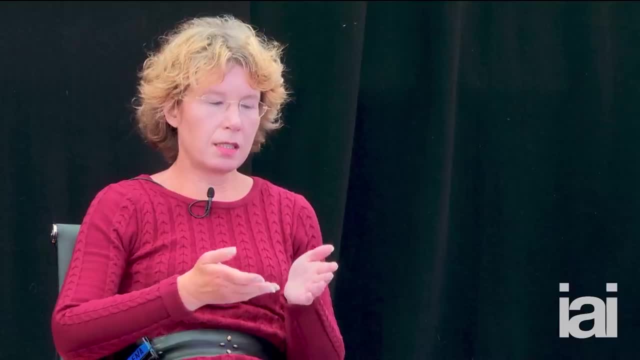 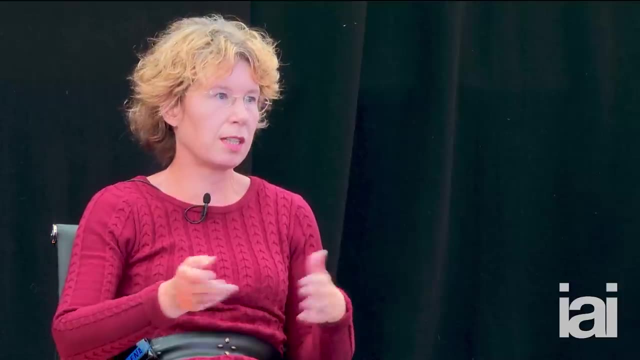 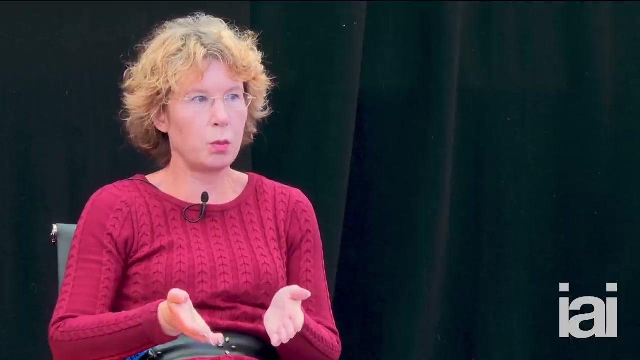 we have this path, dependence, and so we have settled on a particular method of making new predictions, if you want to call it that way, for new particles which you can then rule out, and that works very easily if you've learned how to do it like. this is what i was trying to do. basically, i know how it works and that's how you can write. 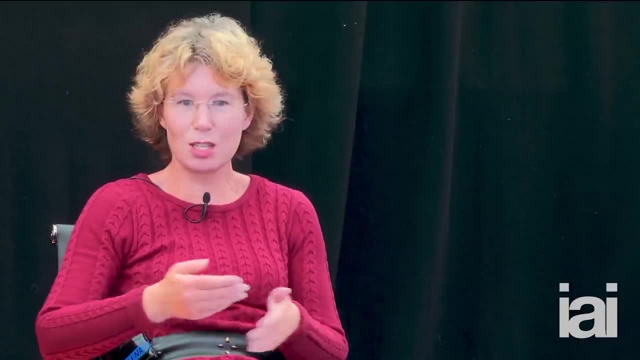 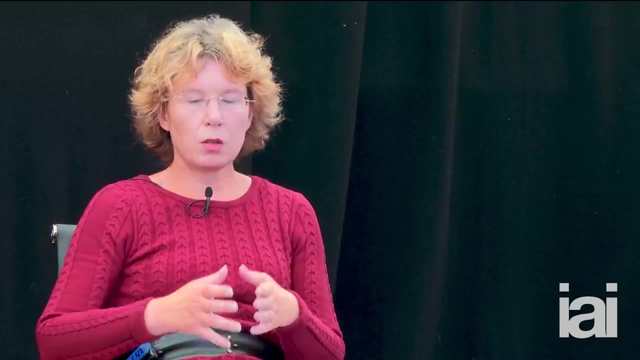 papers, and that's how you get grants, and that's how you get your students, and then the students become professors. so it just goes on and on like this, and if you want to do something fundamentally new, you'll have to start over again from scratch, and it becomes very, very hard to find any support. 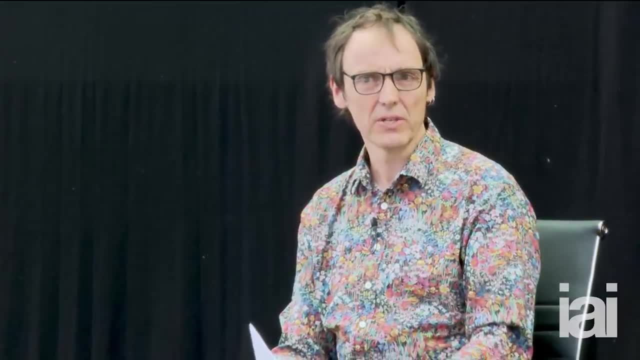 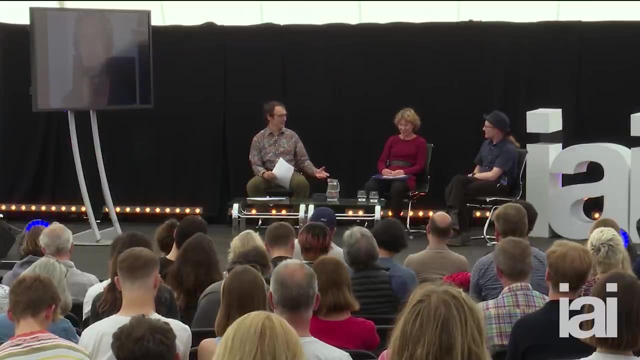 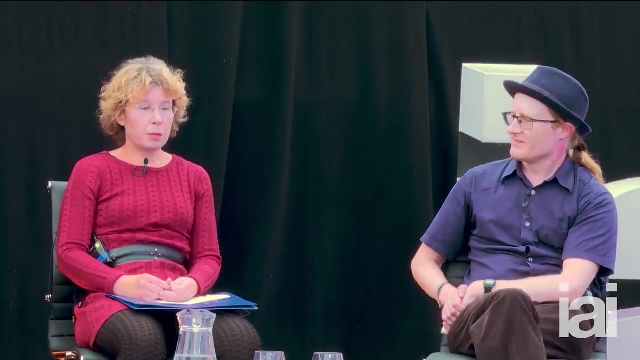 one alternative to that um is, and this seems to be the one that's in the air at the moment. we need a bigger machine to find out more um. you've expressed some skepticism about that, whether that's the right way, sabina. uh, yeah, for exactly this reason. i mean, we do know um, as i think we all agree that the 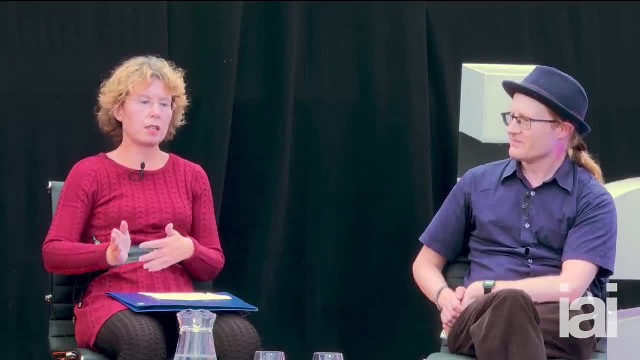 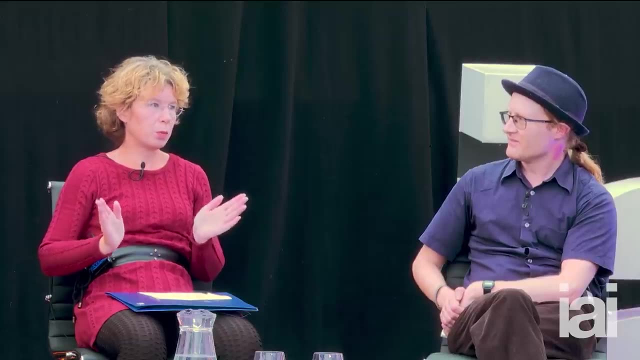 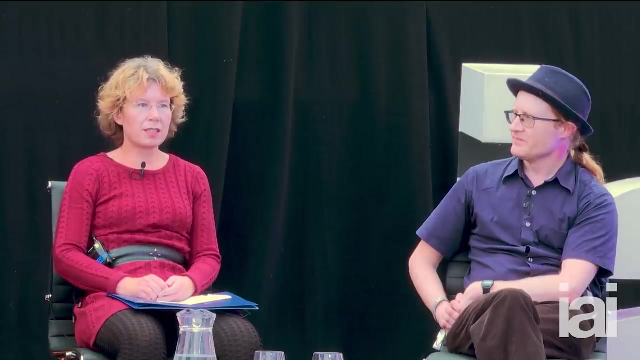 the standard model has some shortcomings and there has to be more to it. but there's no reason why building a bigger machine would give us any help in developing that underlying new theory. all of those anomalies, at various levels of statistical significance, they um may be resolved at much, much higher energy. so even if we build this bigger collider, 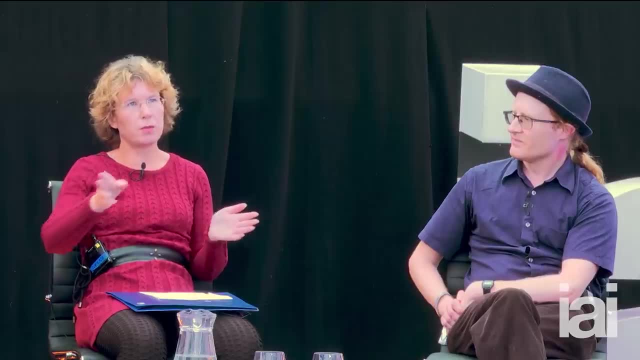 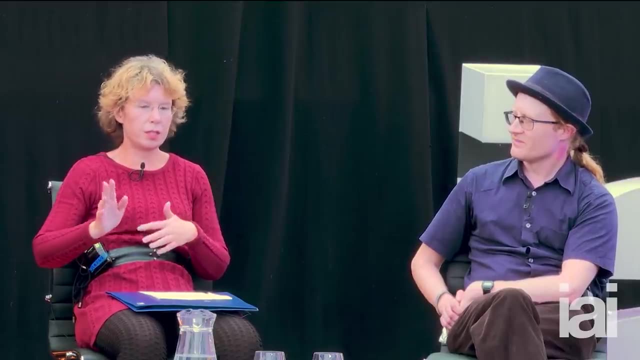 which they are planning for at cern and would have a circumference of, i think, 100 kilometers and cost like something like 20 billions, not counting the operation cost, which would be another 20 billion or something. so so we're talking about a huge bunch of money and the 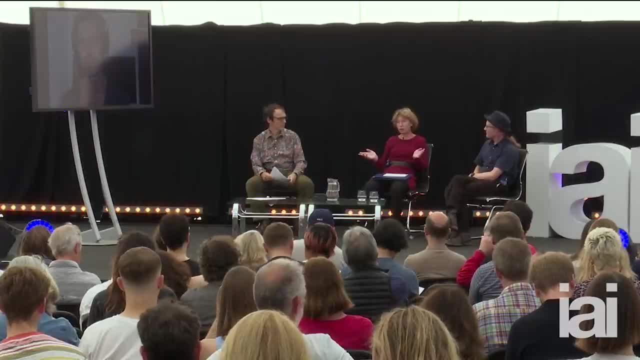 outcome may just be well, the standard model works just fine. and i think, um, that's a little too much money for the standard model and i think that's a little too much money for the standard model. and i think that's a little too much money for the standard model and i think that's a little too much money for the. 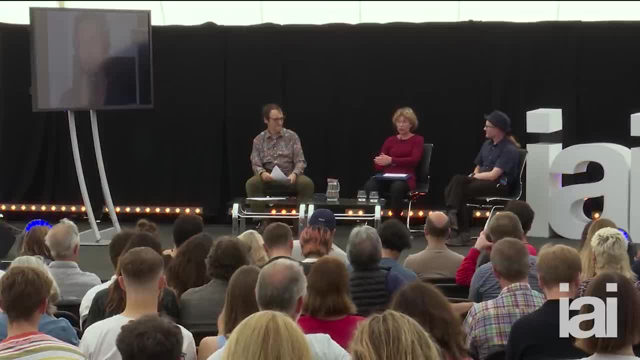 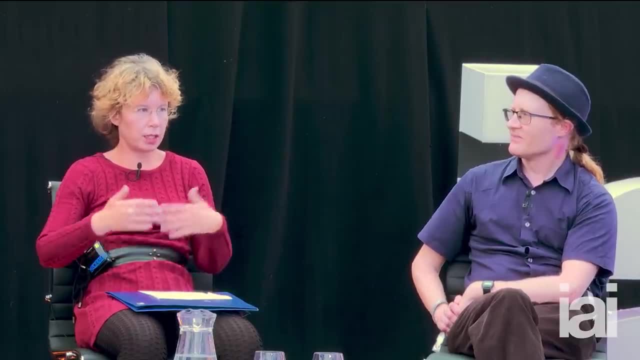 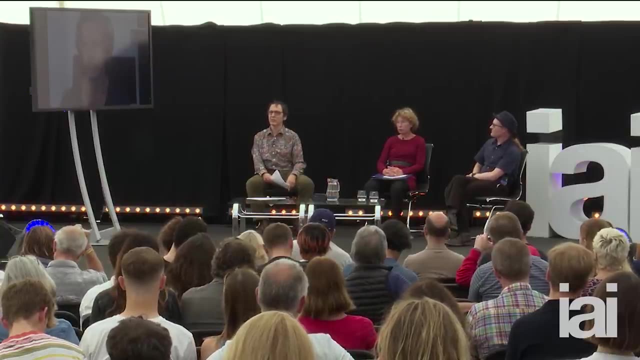 that little, uh, prospective payoff, which is why i think we have to figure out what are more promising experiments are to look at, where we can expect a bigger bang for the buck, so to speak, and beyond. it occurs to me that this is somewhere where the philosophy of science might actually be helpful. 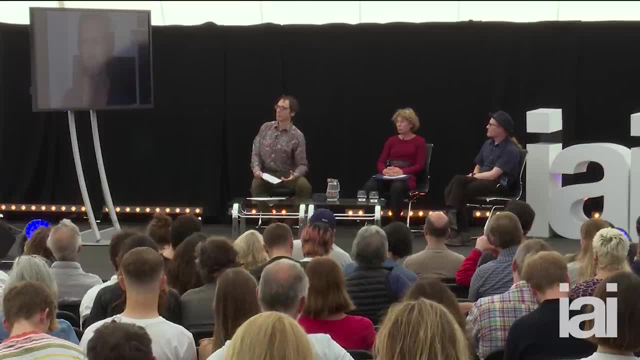 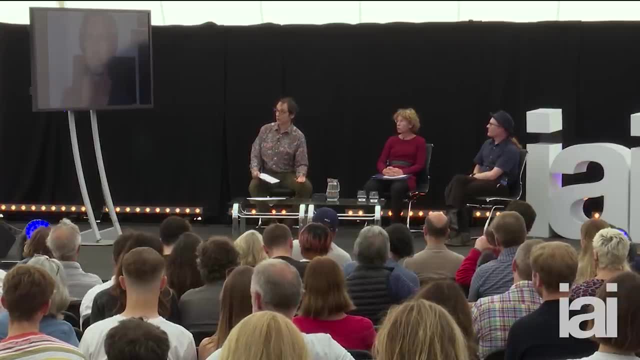 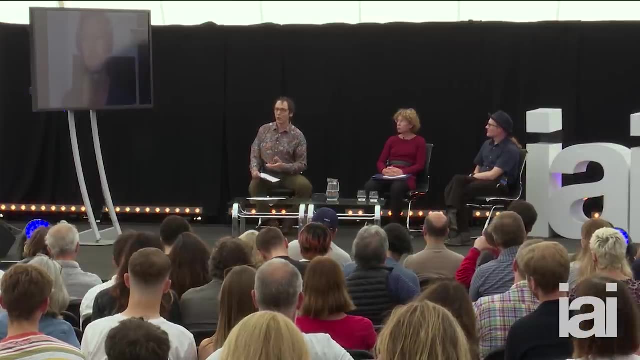 and it's been interesting to me that, um, there seems to be more dialogue now between high energy physicists, fundamental physicists and philosophers of science to try to find some resolution to this problem, and one of the issues, as you've you've touched on, is how you know when. 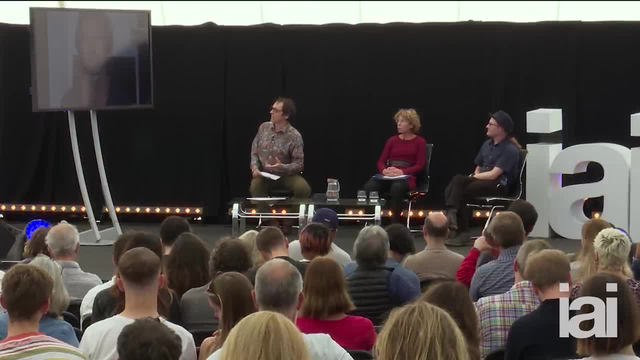 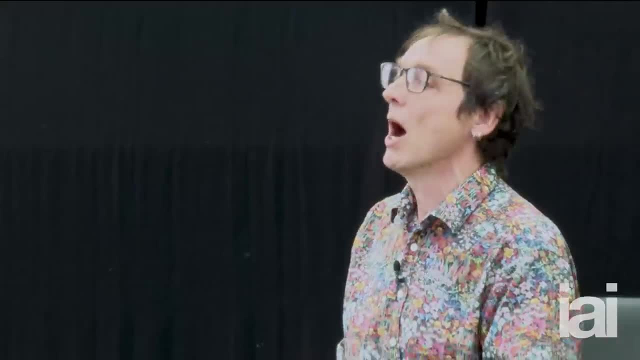 when, uh, you, you just keep waiting because you have a theory that seems to do a lot of things pretty well and so you don't want to throw it out, you know too casually. and when you actually decide, no, hang on a minute, we need to turn back, we need to go back down the path and rethink some of the 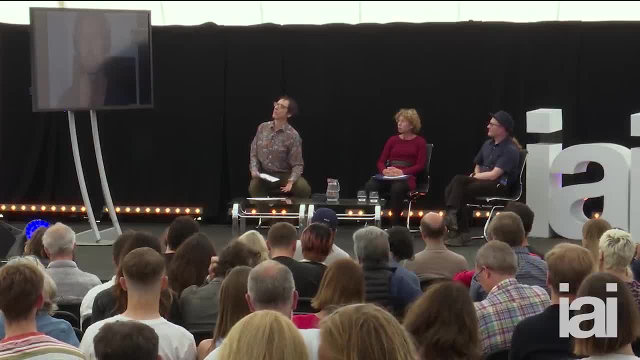 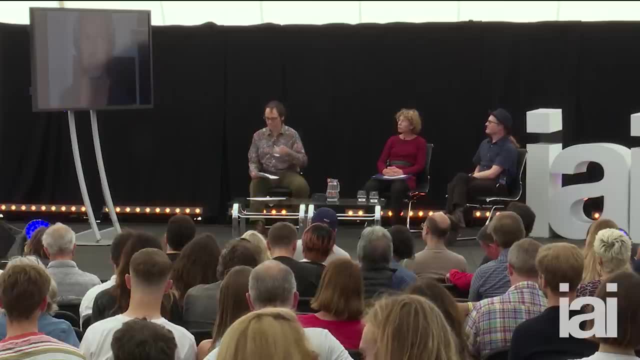 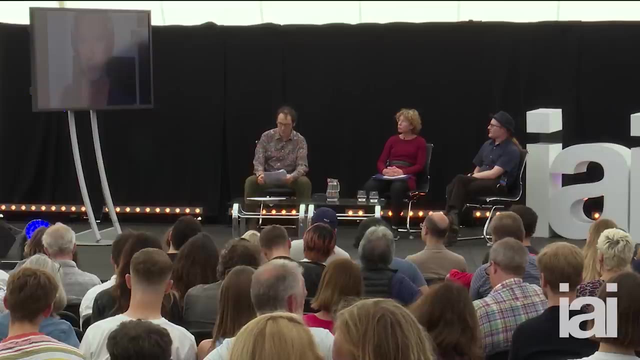 fundamentals. is there any guidance that the philosophy of science can give to the people who are in the field to give to that question? well, i'm, uh, i am also positive about like i'm seeing increasing dialogue in these fields, when it comes to the nature of evidence, for example. 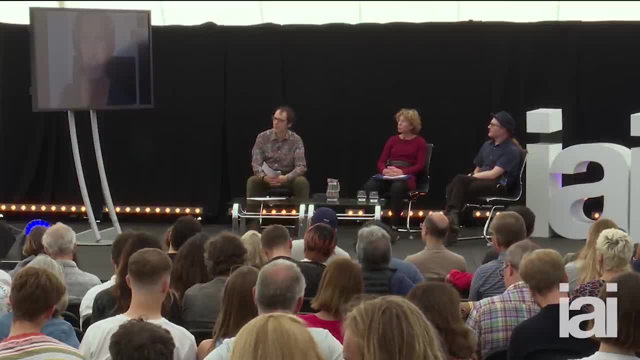 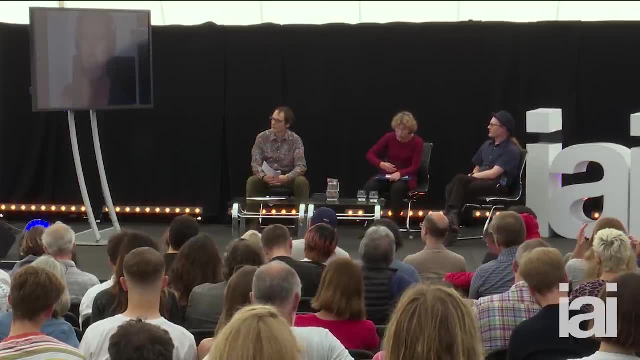 this is where it's. it's worth noting that we're talking here in the context, for example, of dark matter or these latest uh experiments. uh, something like evidence is often bandied about and there's a um, there's a sense in the field that something has more or less. 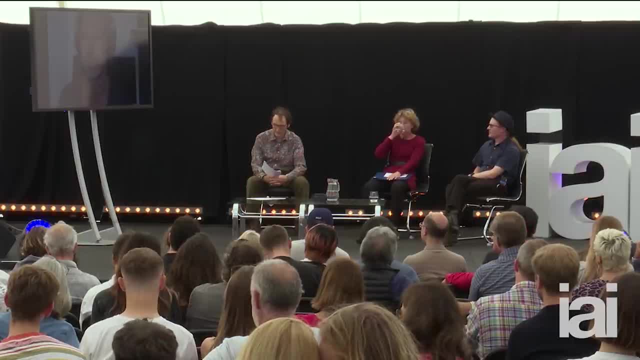 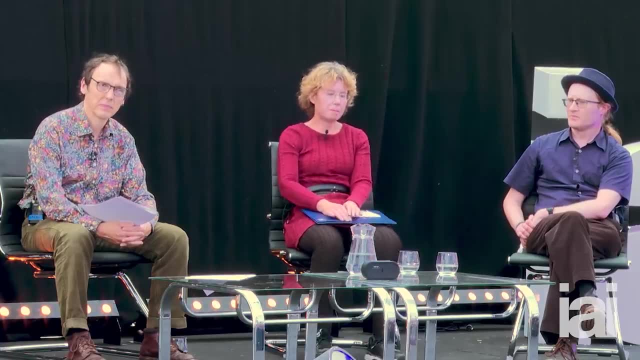 been proven. something like dark matter is taken by a lot in the scientific community and beyond as just more or less proven to exist, and it's worth pointing out that how the evidence for something like dark matter comes about is not in any direct empirical sense. in fact there is no. 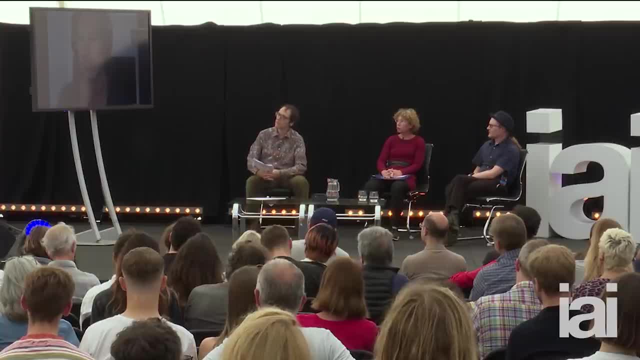 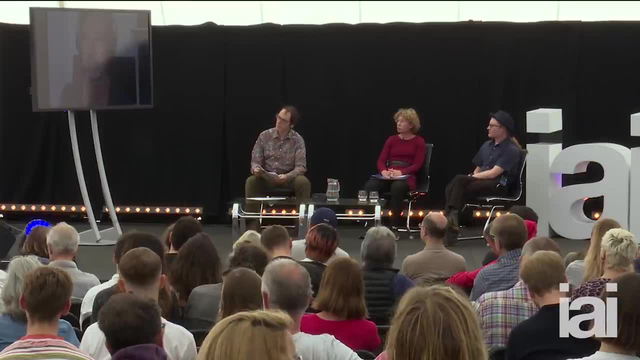 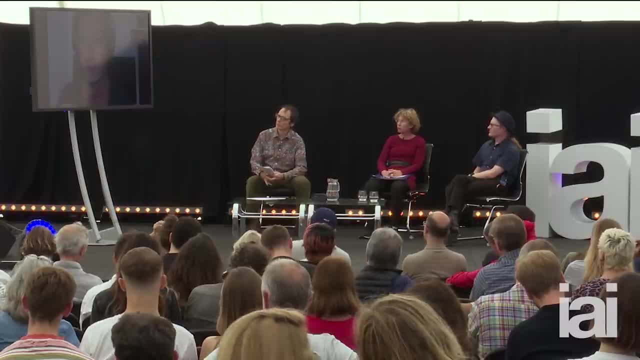 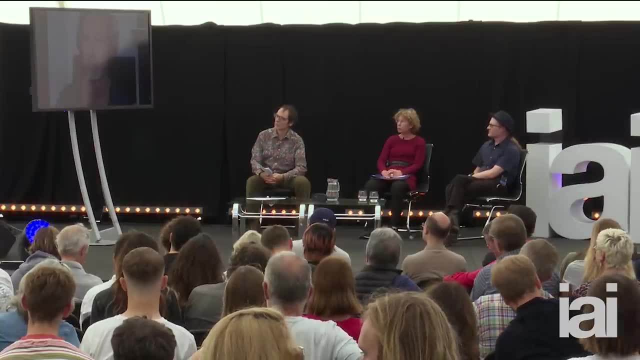 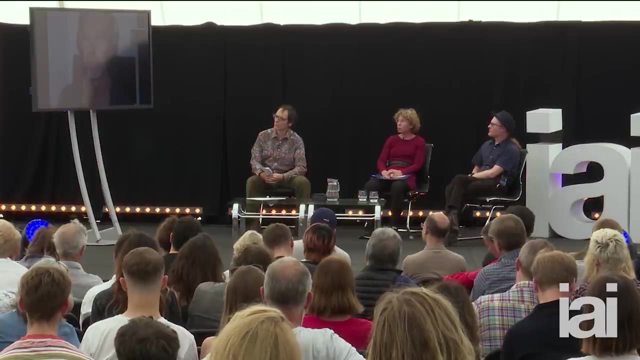 this is that, uh, the. if the model that we're using is correct, there has to be something like dark matter or a new force or something to explain that gap. uh, this is a familiar pattern in the history of physics, and this is especially true, i think, in cosmology, that the more observations we make, 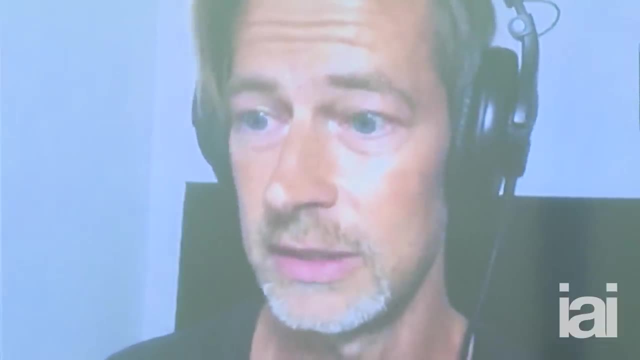 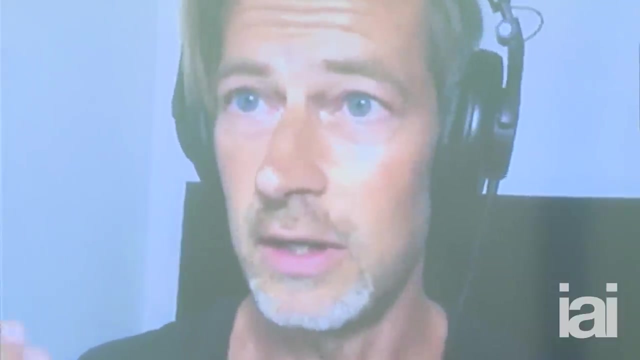 the more discrepancies we find with model predictions, uh, the more cosmologists adjust or add parameters to fit observations. uh or they propose additional hypothesis, or new physics, or such as a new force, and uh or like in the case of this latest experiment, which is all very exciting for scientists because this means a path for more research. 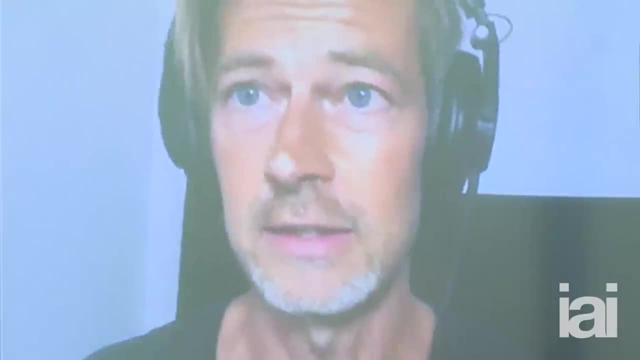 but it's just worth pointing out that what a lot of these kinds of solutions have in common is they also preserve the core assumptions. they add on something or erase a new question, but they they make the more fundamental or radical questions almost impossible to reach, and so 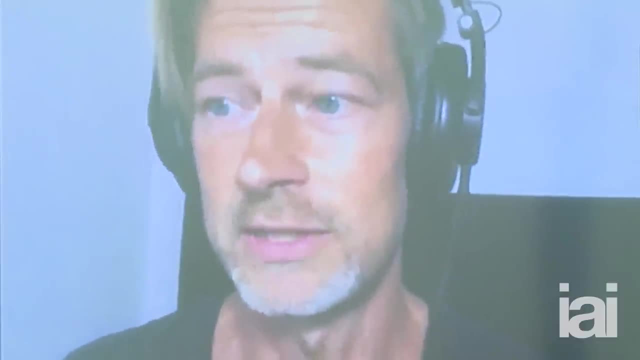 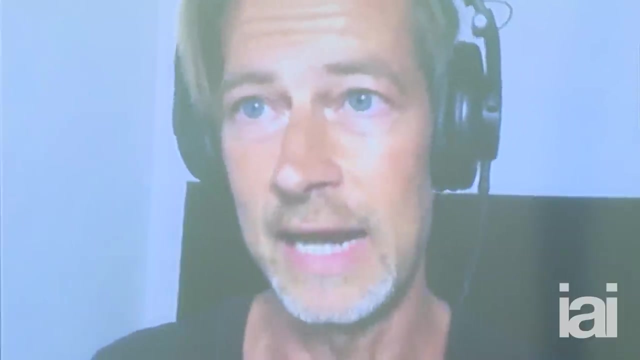 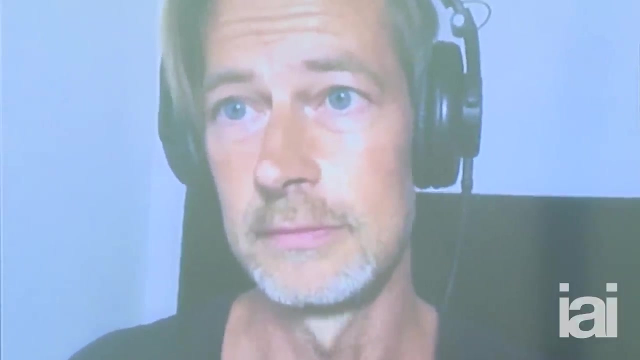 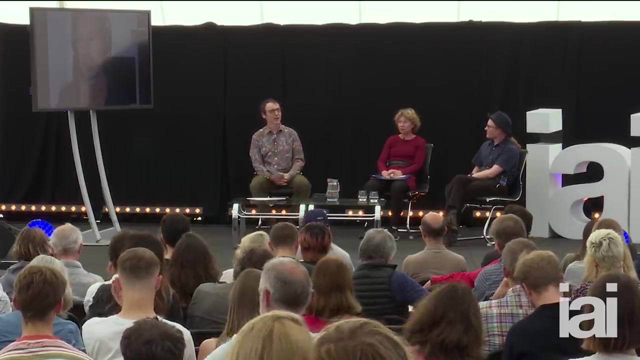 i think the philosophical view i mean it's very limited. i'm not in a position to judge the merit of particular kinds of evidence, but if there could be any help in asking more fundamental questions about how we got into the situation in the first place might be helpful. right, um sam? i'm also wondering whether um is is just a bigger machine, the only? 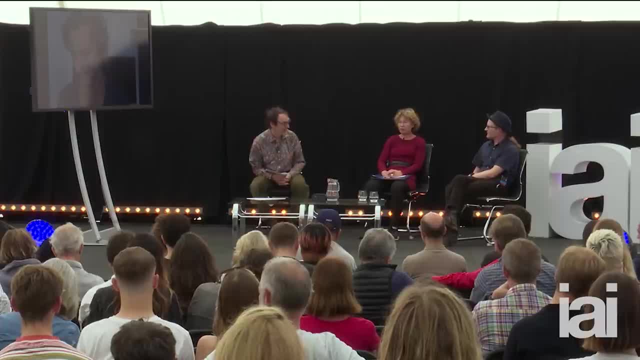 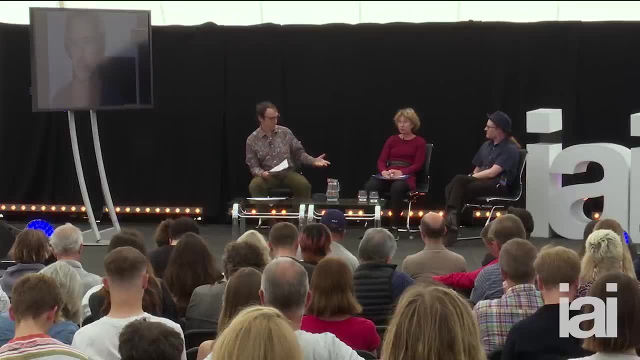 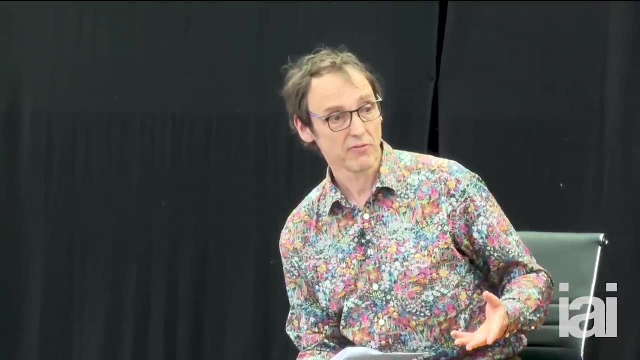 alternative, the only um empirical alternative we have for addressing these problems. i mean, we talked a little bit just beforehand about, you know, ongoing work on the muon g minus two issue using the, the devices we have already. are there other ways that we can already be seeking for a path? 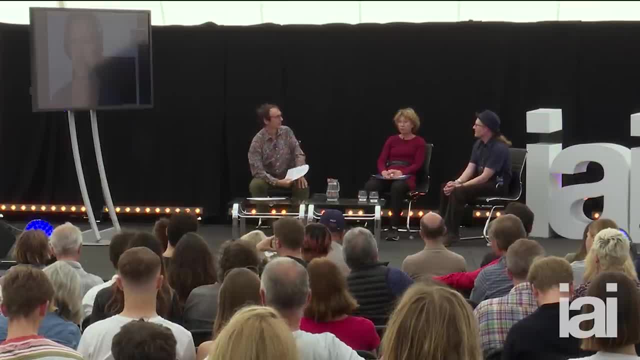 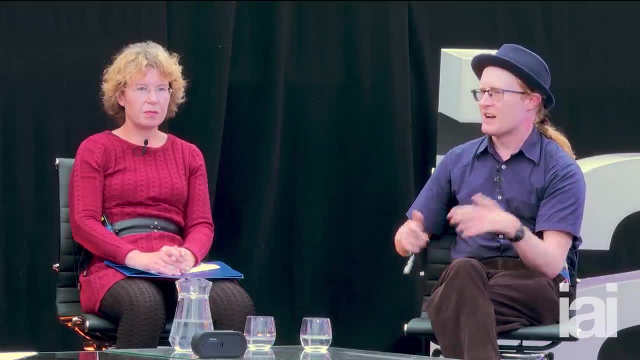 forward, uh, without having to build this even bigger collider. well, i think that this is an open question in particle physics at the moment, and so, yeah, there certainly is this, this uh plans for a future circular collider, uh, but i think it's by no means- there's no means- agreement among past. 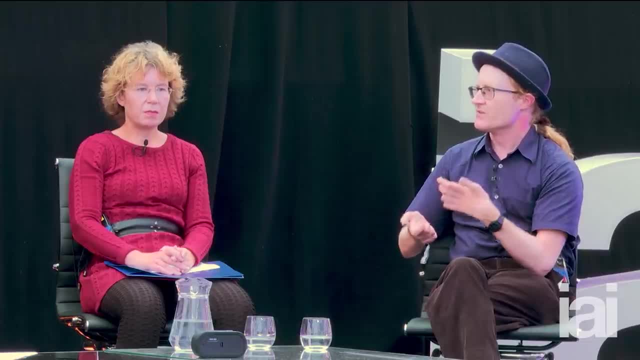 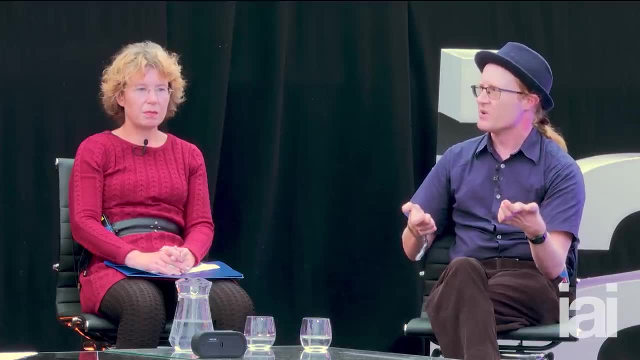 assists about whether this is the right way forwards. um, for the reasons that spina has said, that you know, it may well be that we build such a machine and it doesn't actually find anything, and, uh, you know, of course that's very difficult to predict, but we do want to focus on 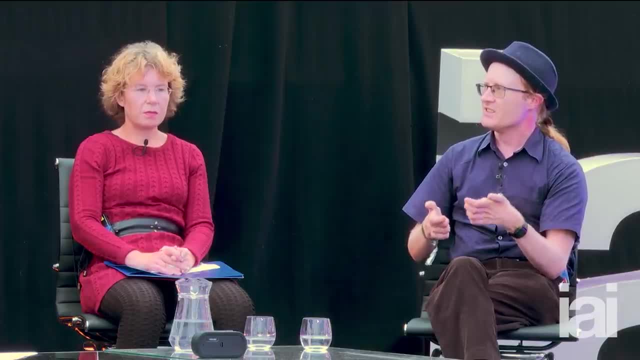 the experiments that are most likely to deliver an interesting result, the alternatives you know. it could be that, yeah, more precision measurements of particle properties, um could be interesting things, like the muon g minus two experiment. also measurements of the electric dipole moments of particles. this, this is another way of doing particle physics. 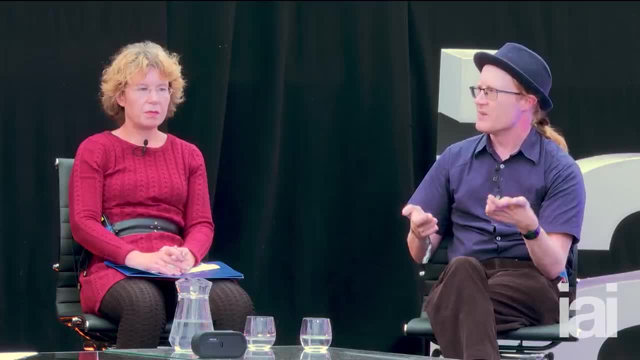 but there's only so many of these experiments, uh, that we, uh that we see at the moment. i mean other possibilities, and maybe do we need to look at ways of studying the ultra high energy cosmic rays that are bombarding the earth from outer space. that energy is far higher than anything. 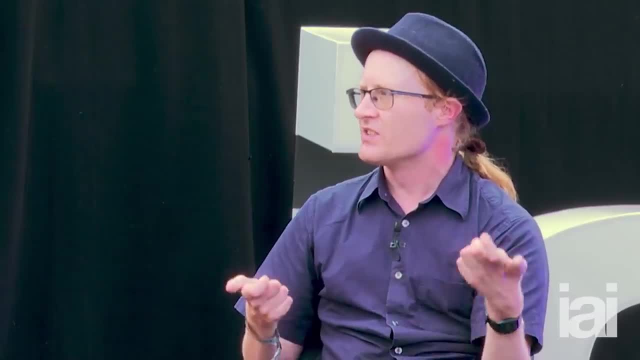 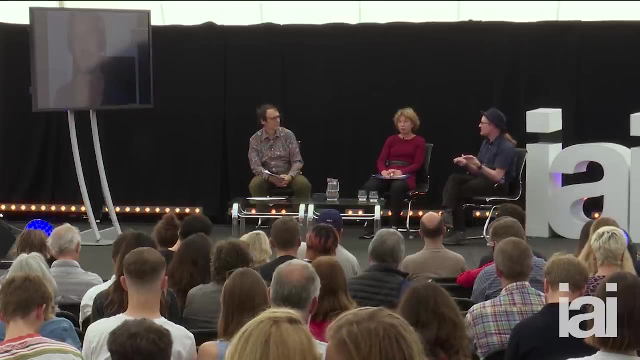 we could ever reach with a, with an accelerator we build, or do we want to study, neutrinos, which are a completely different game to studying other particles. so there's all sorts of different experiments that we could be doing in the future and, yes, this is an open question in. 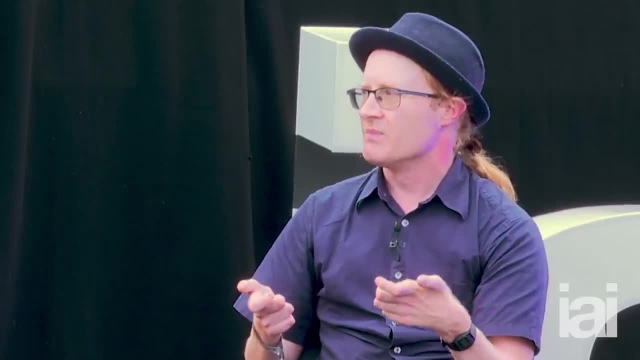 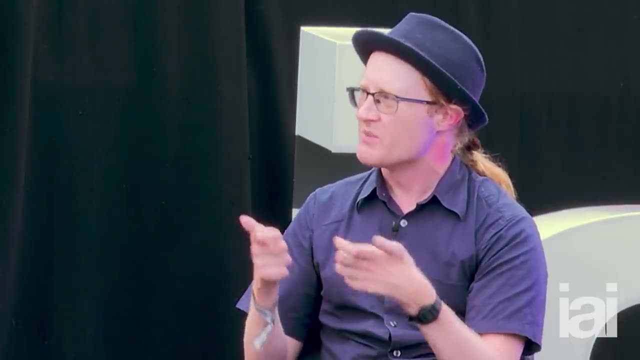 the field at the moment is: what direction do we want to go in? and maybe this is, i think, what we'd really hope is that, uh, you know, if we discover some particles at the lhc and that suggests that there's going to be more a little bit further, then that will build on the case of 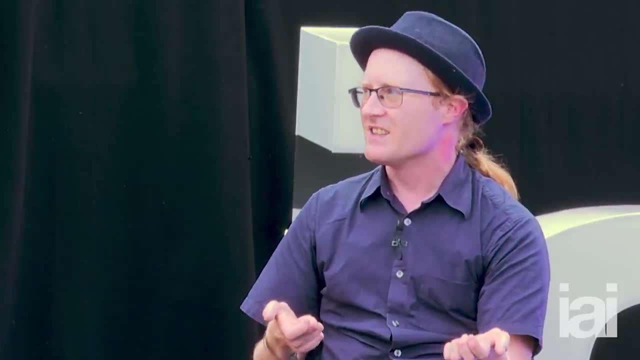 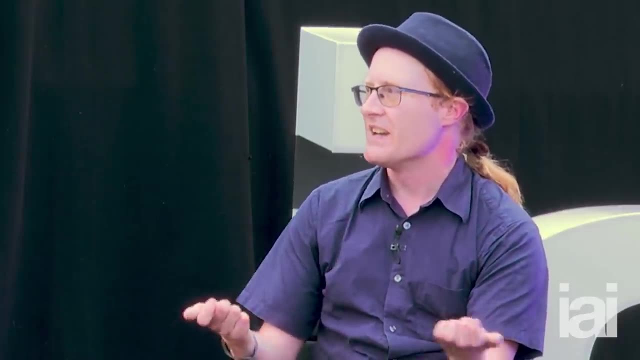 building a bigger accelerator. if we don't discover anything, then i think it's quite likely that people are going to listen to theorists like savina and say, actually no, this is not the right way to go. and and then we. but then there will also be other people who say, well, we, you know. 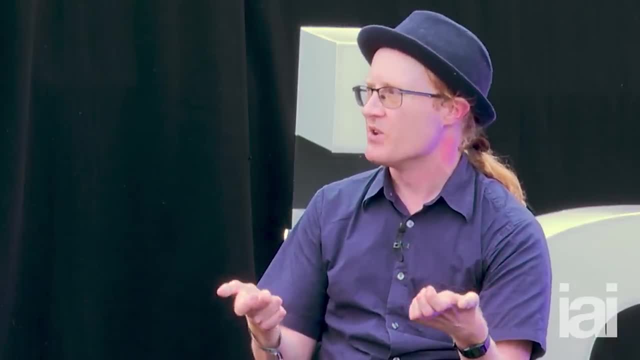 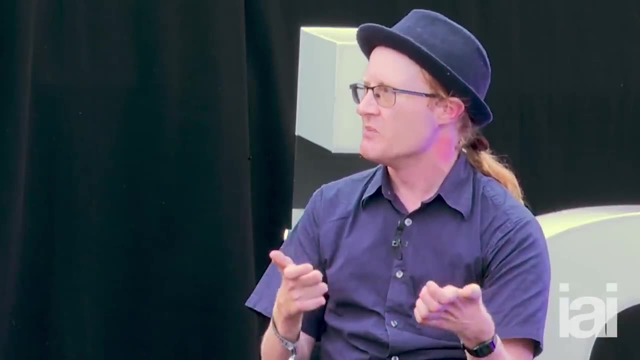 we still need to to explore further. so you know there is a case for building such a machine anyway, because you know we just need to explore to higher energy scales and if we stop now we'll never go further. you know, even if a new machine doesn't see anything, it would be at least a technology. 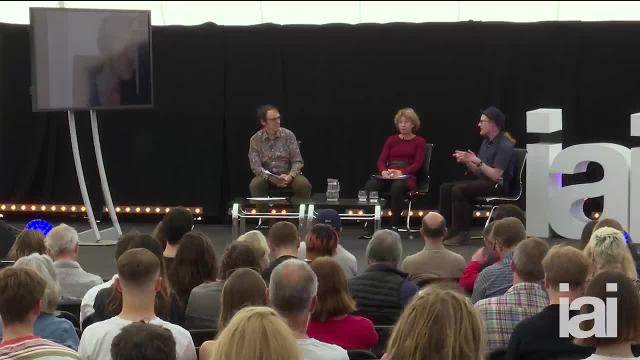 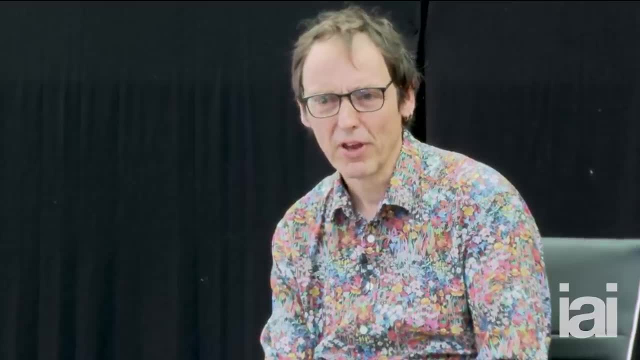 demonstrator for the one that may come after it, but i think that's going to be a very hard argument to uh to uh to convince somebody to spend 20 billion on such a project, right, um, i, i wonder. before we move on, i'd like to, um, just say a little bit more about the dark matter problem, because, 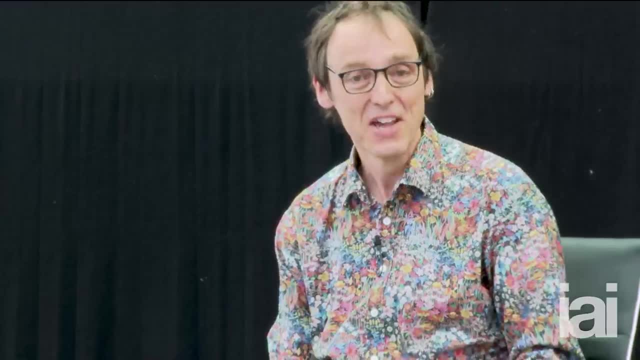 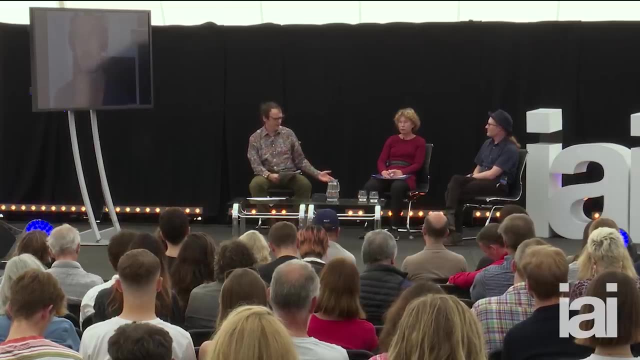 although it's, you know, not the only, clearly not the only puzzle facing fundamental physics, it's probably one of the ones that people hear most about and know most about. um, and you know, here we've. there have been many searches for dark matter particles that have still found nothing. 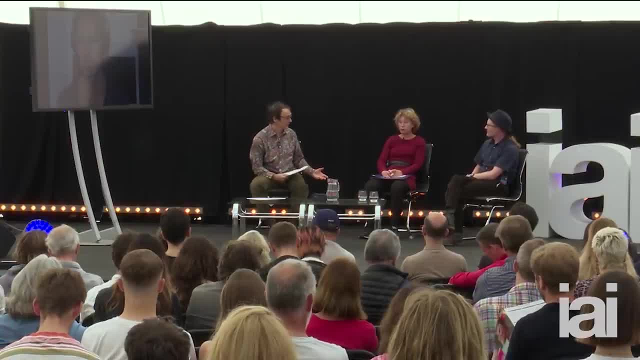 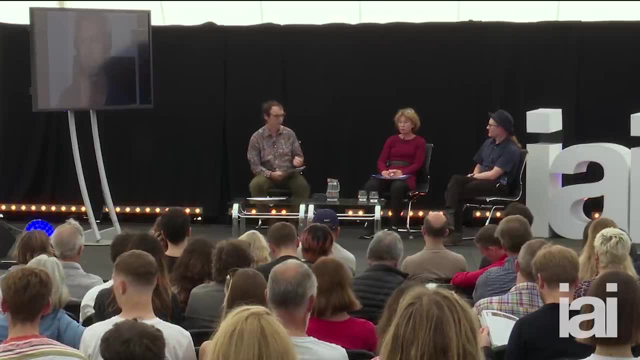 sabina, do you think that we just in in that particular case, we just need to keep looking, or is there something else we should be doing to try to resolve this, this issue of why we seem confronted with a need for dark matter? well, as bjorn said, um the evidence that 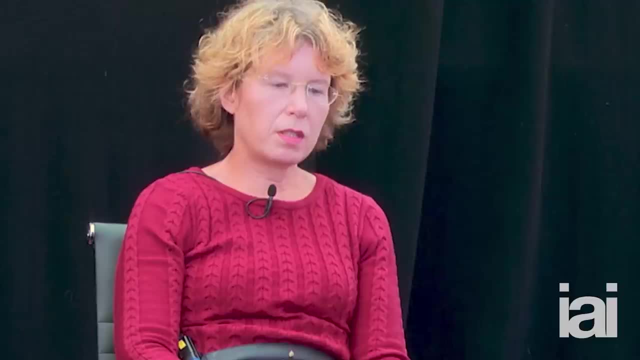 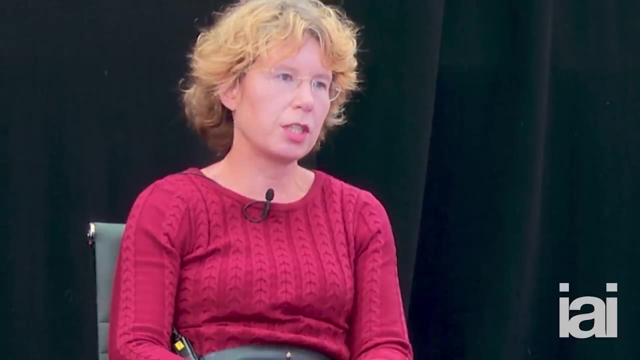 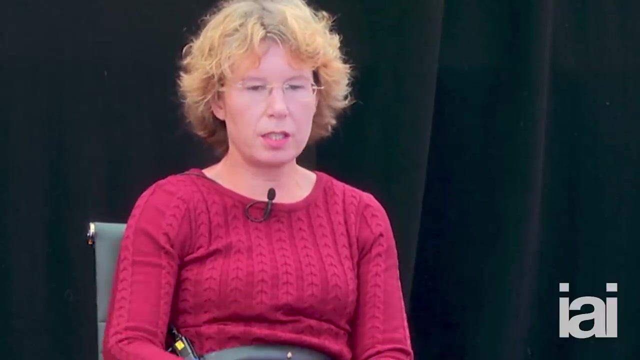 we have for dark matter is, uh, indirect, um, so we infer that there has to be. if you believe that it's some kind of matter, we infer it from astrophysical observation, gravitational lensing, for example, or galactic rotation curves, motions of clusters. we measure the velocity and we just know that it doesn't work with general relativity and the standard model. 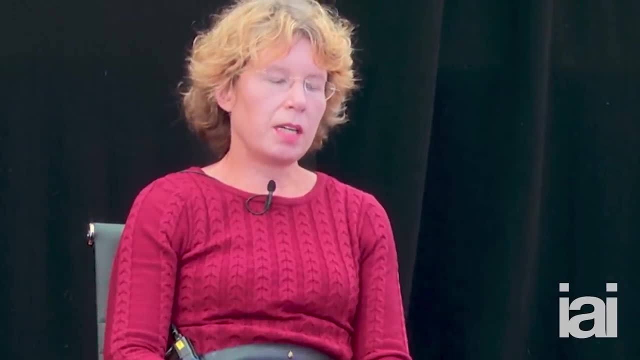 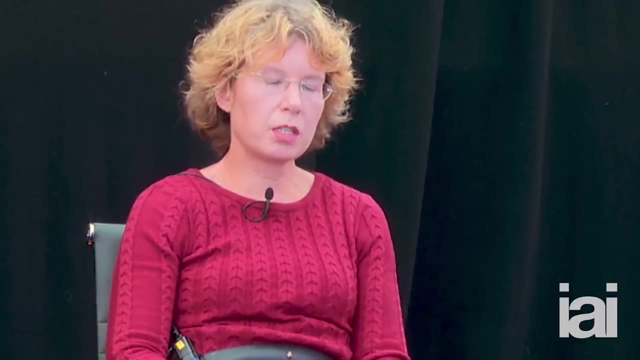 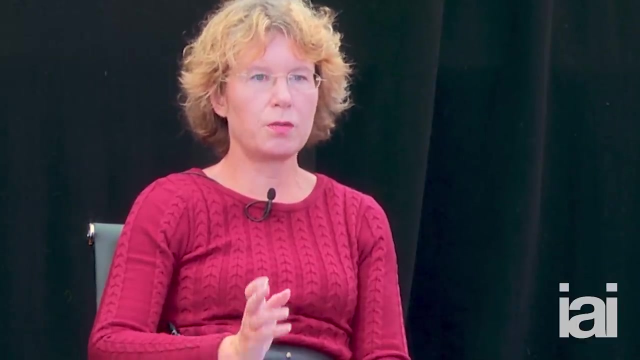 if you combine it it doesn't come out right, and adding a new type of matter is the easiest way to resolve this discrepancy between the observation and the theoretical predictions. but these are very unspecific about what exactly the properties of this dark matter are, if it exists. 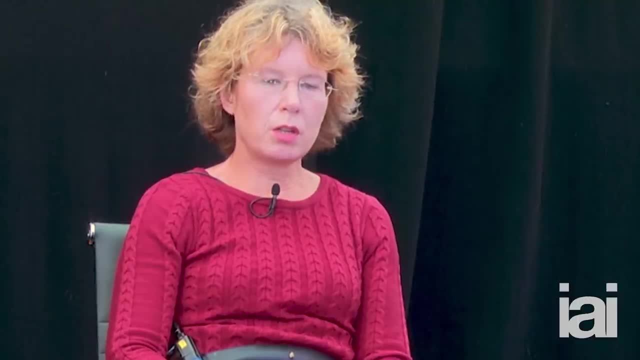 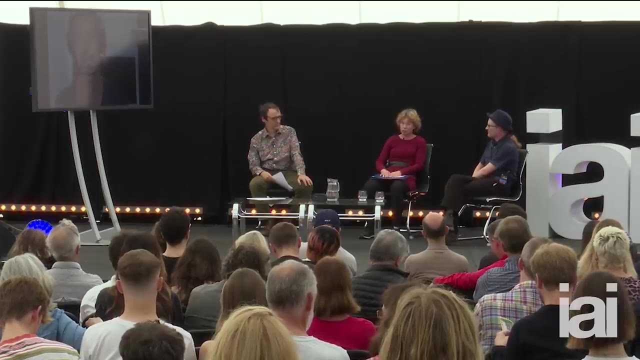 so we don't really know what's the mass of the particle. we we don't know how it interacts with itself, um, or with other matter. i mean, we do know that it doesn't interact with light, because that's why it's called dark, but that's pretty much it. and so if you know that little about a particle, 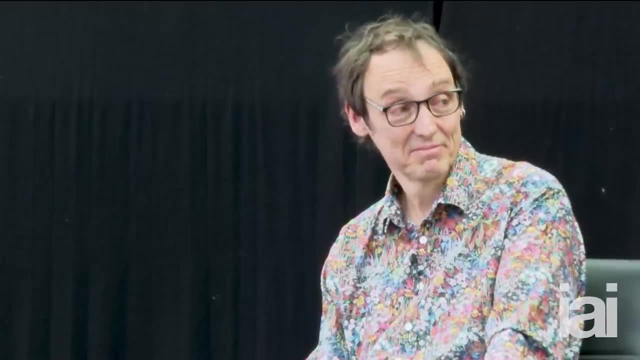 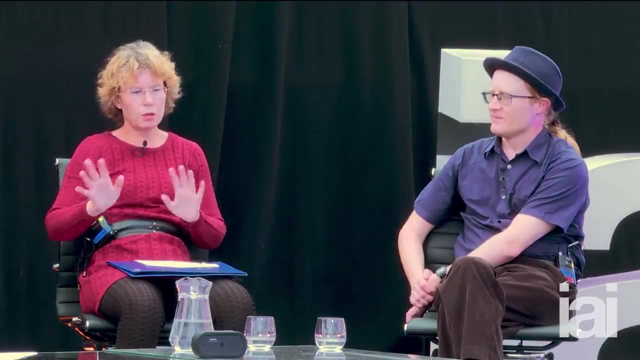 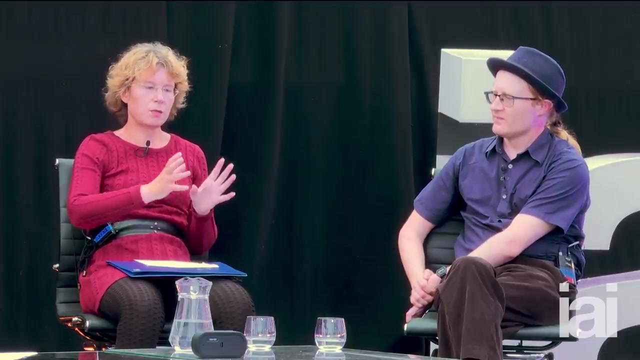 it's really really hard to build a detector for it because you don't even know what you're looking for, and so the reason we've built a particular series of detectors. actually, they're kind of two types of experiments. uh, one type is looking for a type of particle that's called a wimp, a weakly interactive. 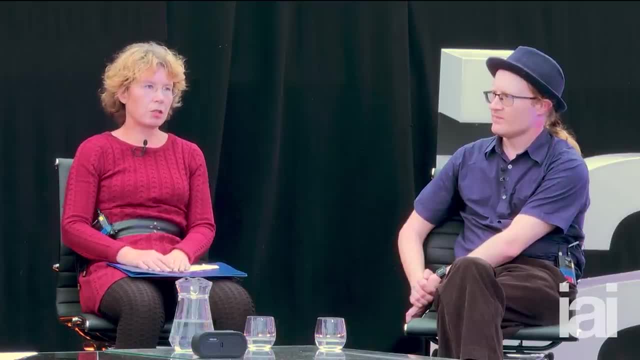 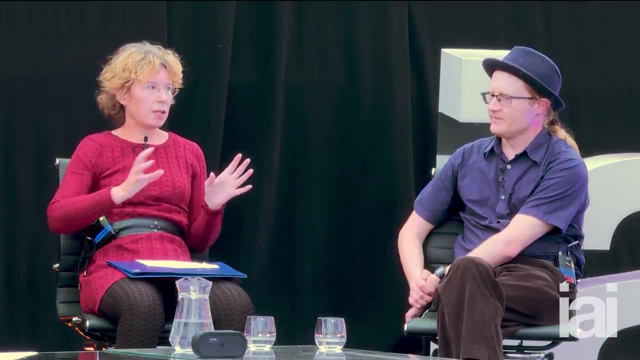 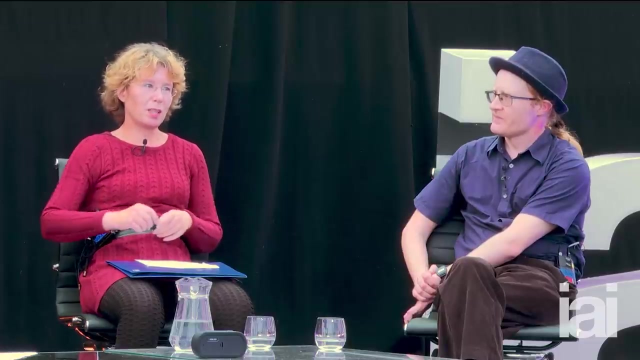 interacting massive particle and the other one is an axion, and both of these particle types, so they're actually classes of particles. you could say um were motivated by theoretical arguments, and that brings us back to the problem with the theory development, because you can ask how well motivated were they actually? um, so wimps in. 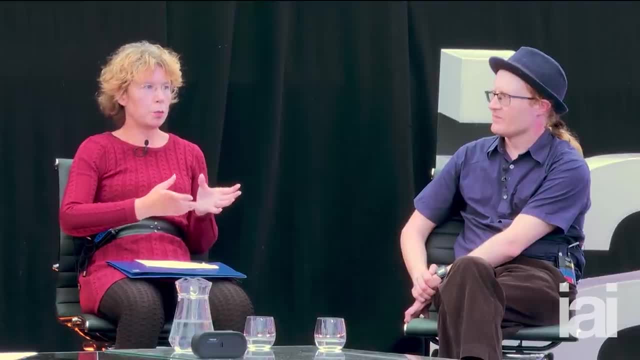 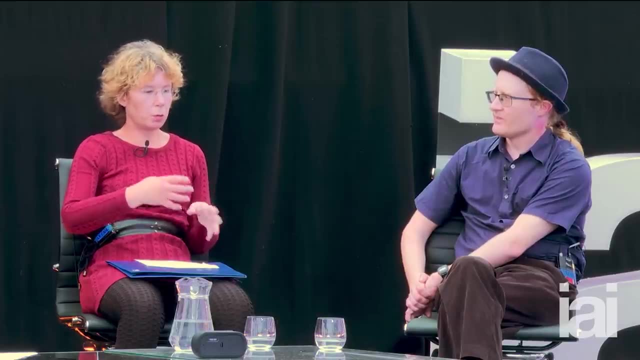 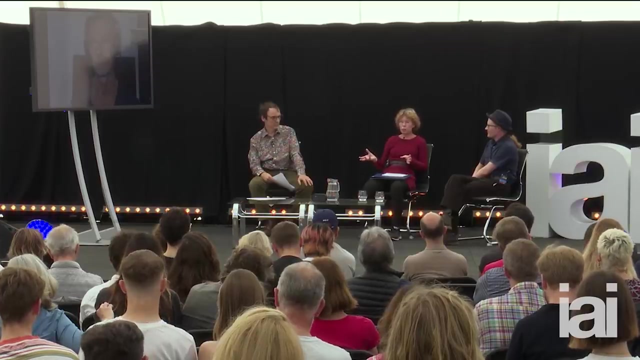 particular, were very popular because they come out of supersymmetry, um, so it brings us back to what i said in the very beginning about how particle physicists came to like symmetries and the axions they were predicted basically to you know, make the standard model a little bit prettier and the 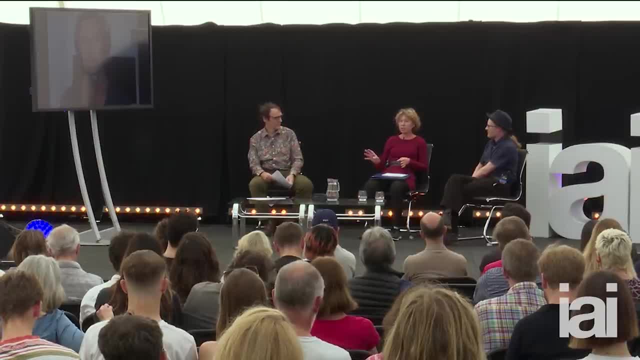 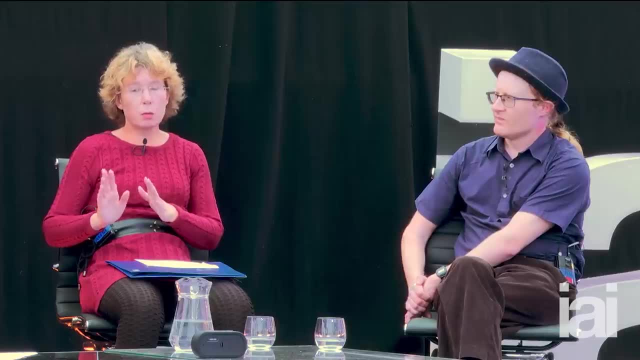 version of the axion actually was ruled out very, very quickly in the 1970s, And what happened afterwards is that physicists just made the theory more complicated, And this is something, by the way, which we see over and over and over again. Bjorn already mentioned this- that, if you 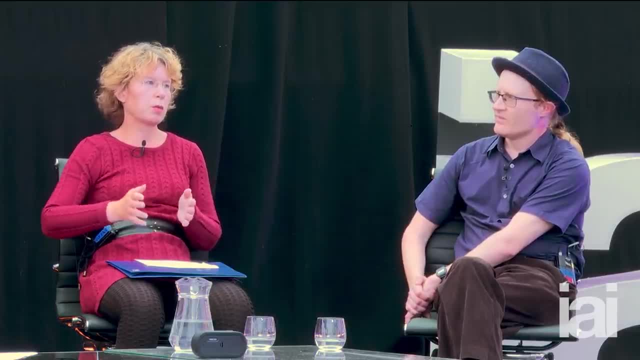 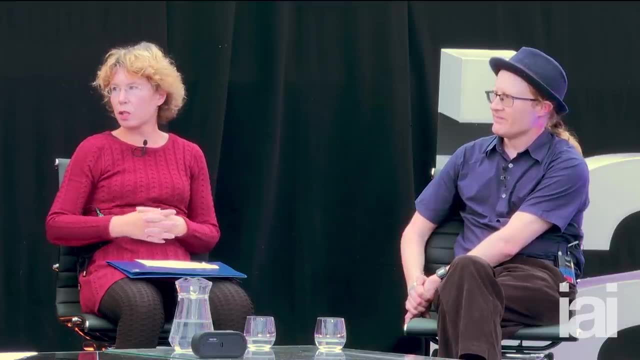 have some prediction that runs into conflict with the experiment, then the theories just go and make the theory more complicated, So in the end it can just accommodate everything. And that's also what happened with the axion And that's what happens now, when every time these dogmatic 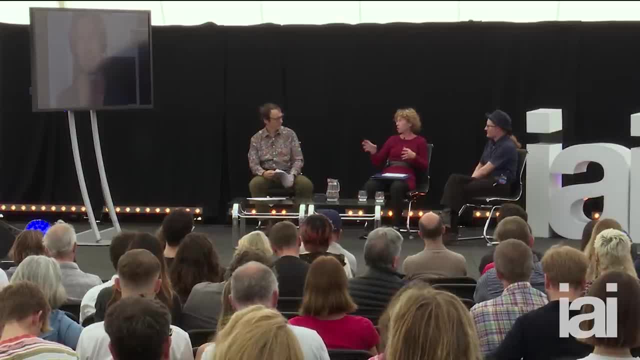 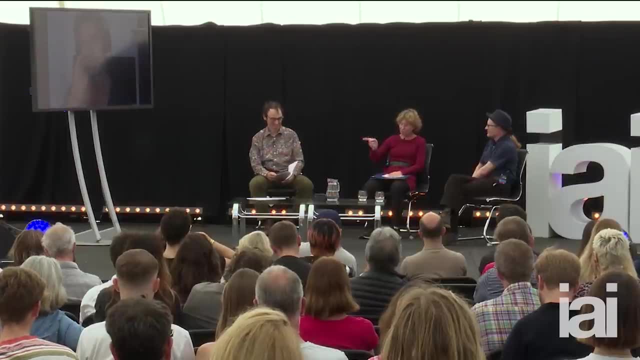 experiments don't see the particle that they were looking for. the theorists will just go: oh, it's a little bit more massive, It's a little bit less strongly interacting, And we'll have to build a bigger collider detector. Sorry, Okay, Well. finally, I want to ask: why does it matter? 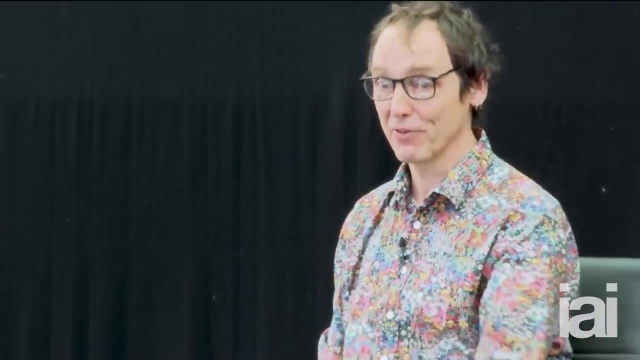 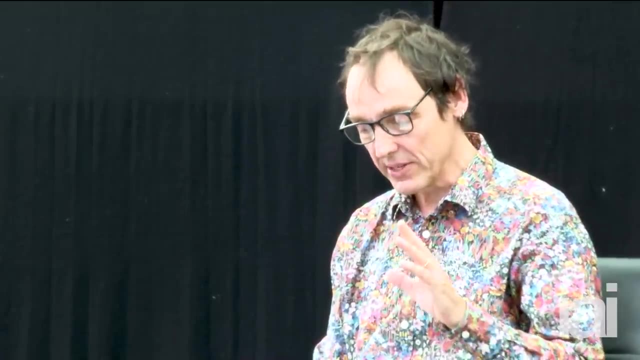 Why should we care? And it's really lovely to see that presumably for all of you, you do care enough at least to come and hear about it. But really the question is, if we discovered- I mean Bjorn, for example- if we discovered that you're right. 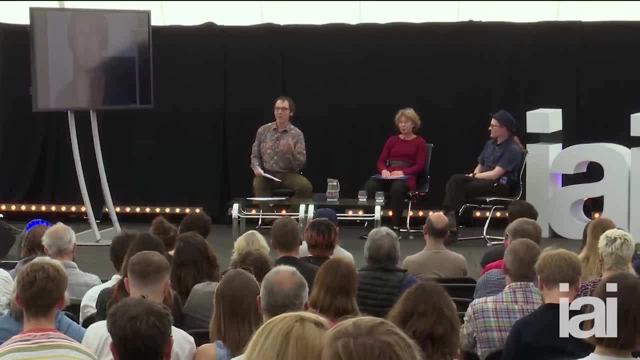 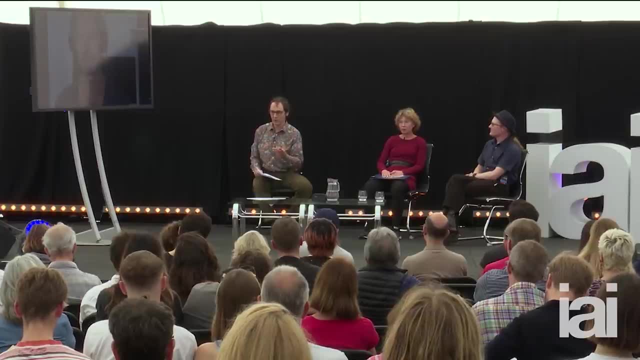 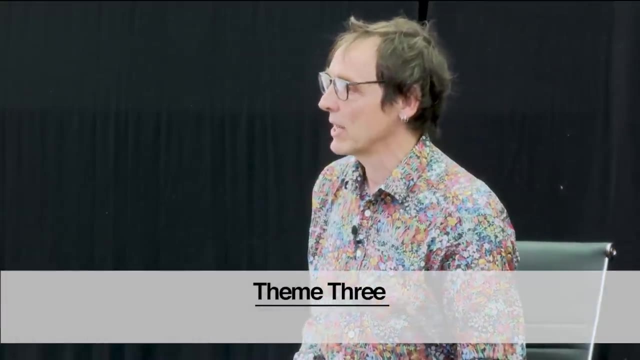 in thinking. we actually need to go right back and really fundamentally think about, and perhaps change, some of the assumptions that have brought us to this point so far in terms of the standard model or the standard models. would that significantly? would that have wider implications? 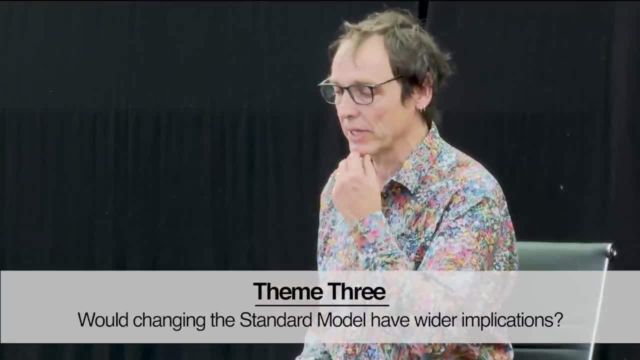 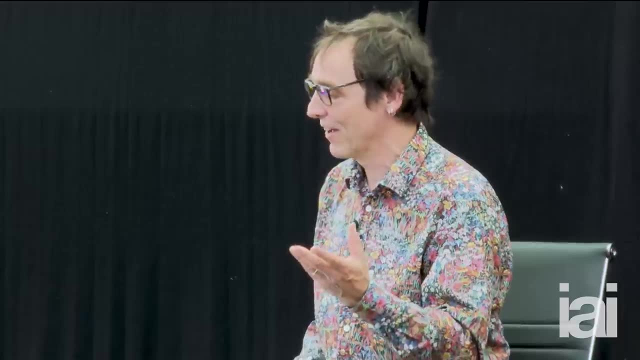 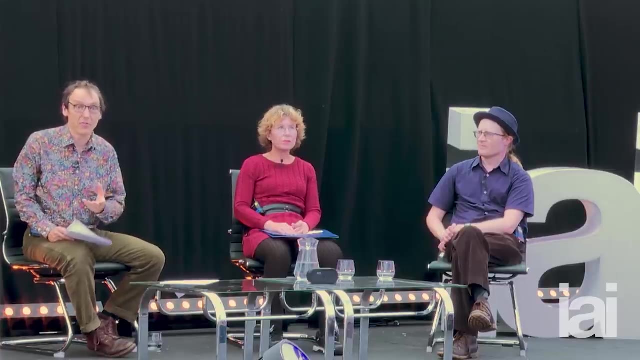 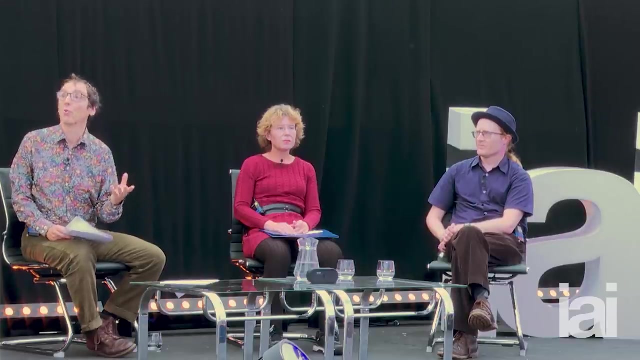 philosophical and social. I'm thinking here. you know that clearly in the past, changes in our cosmological worldview have done. the heliocentric theory did seem ultimately to have broader implications. The discovery of the Big Bang, you know, arguably changed our view of where we sit and what our role is, if you like. 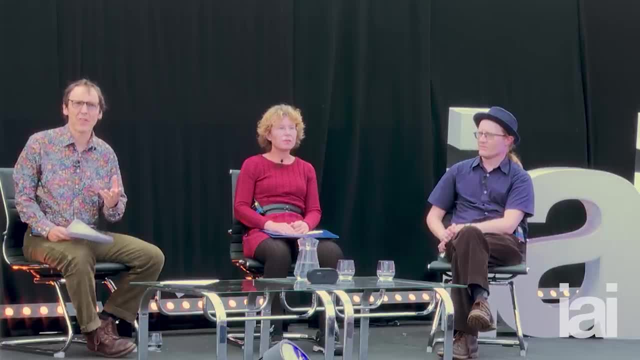 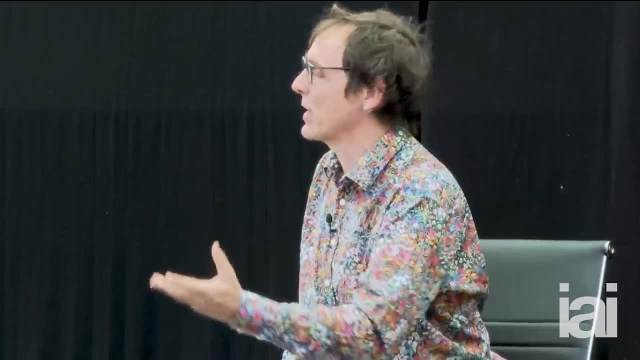 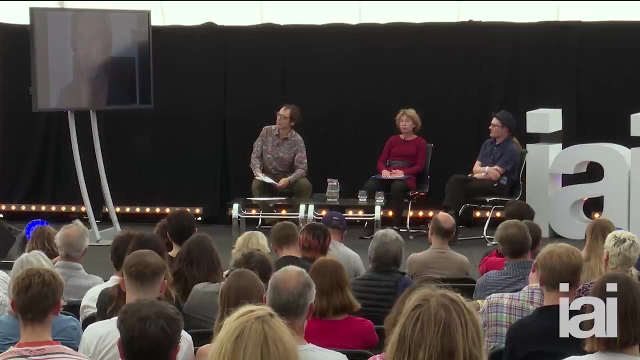 in the universe. Do you think that there is the potential, here at least, for that kind of fundamental rethinking of our position that reaches beyond questions that are, you know, really only of interest to specialists? Well, I think I've tried to make clear from the outset that my own view on this is a little bit. 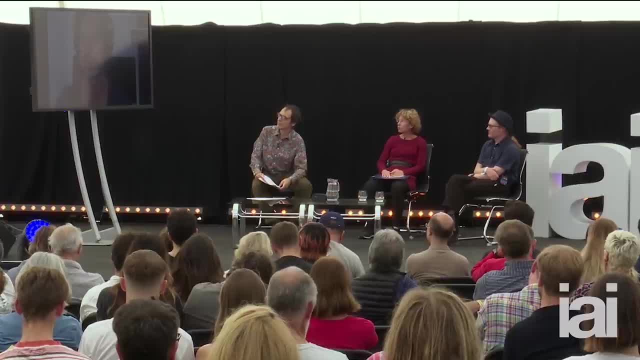 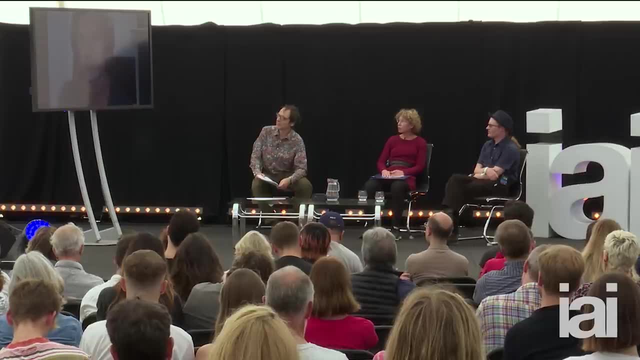 skeptical of how major changes can come about. But to the question of whether it matters and how it matters, this of course does depend on what we would change it to, what a change would look like or how radical it is, As Sabina just described, I mean. 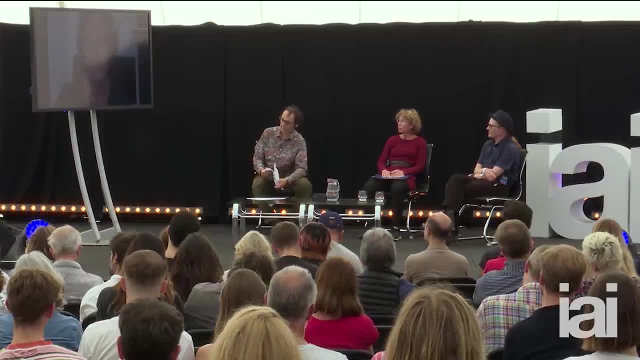 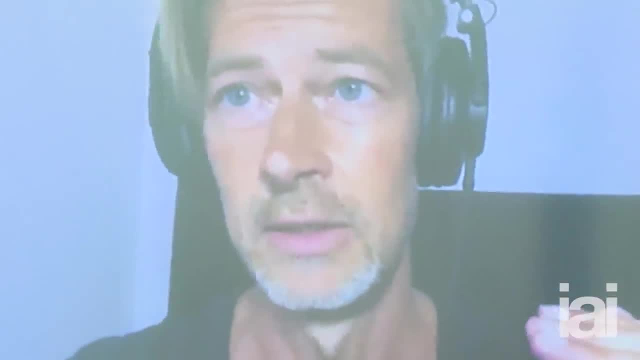 the standard model, the standard model of cosmology that I've been looking at the structure of is like a series of building blocks on top of each other. It's a very, very complicated, multi-layered theory. It looks, when you map it out, like Jenga, if you're familiar with this. 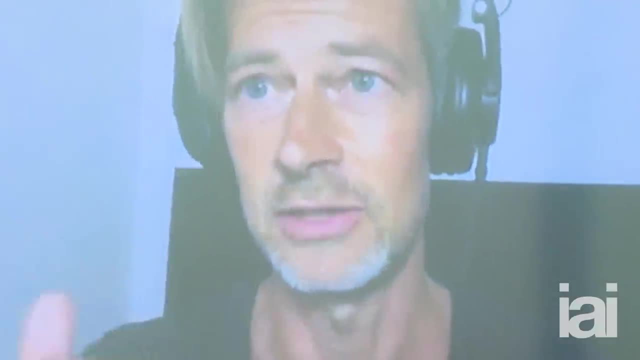 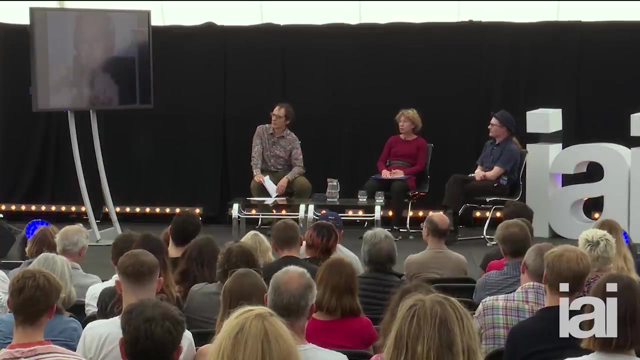 game where it's like multiple blocks that sit on top of each other And if any of the blocks underneath fail, some of the other ones will fall or you can replace one and put another one. Dark matter is such a block somewhere in the middle of that structure that there is a lot of 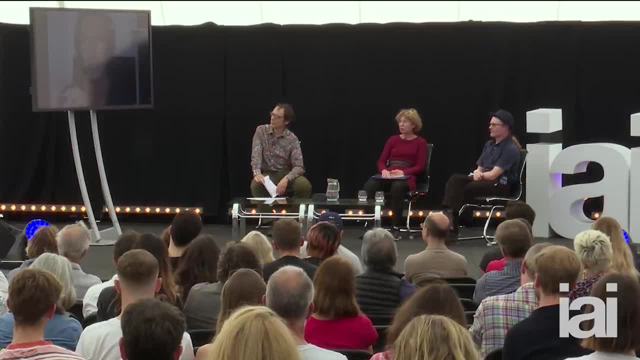 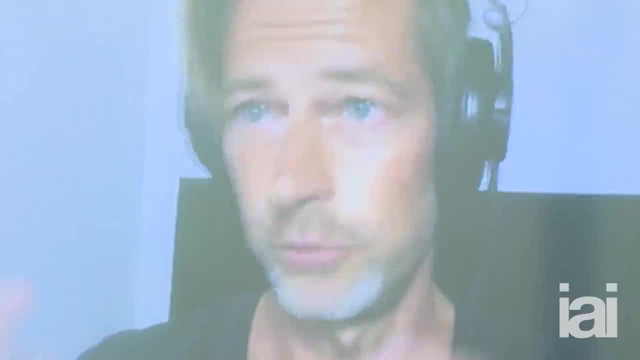 uncertainty, And that is another contender for which I know Sabina is working a lot with as well- modified Newtonian gravity, or MOND in short. So to put this in perspective, if what we call a paradigm shift is, for example, that dark matter becomes more or less abandoned, and in favor, like 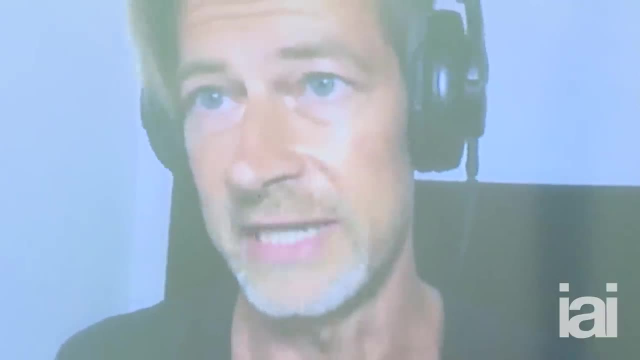 that we move in favor of modified Newtonian dynamics. if that were to overtake something, I doubt that it would affect many lives outside of the scientific world. But if we are talking about a new understanding of light or new understanding of gravity, 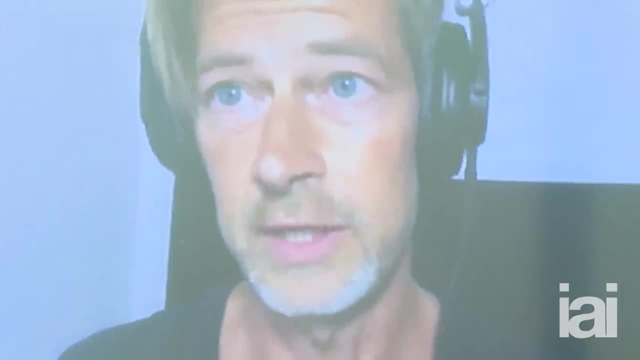 electromagnetism or other forces, or even if we are questioning and talking about the origin story, that the universe began in a hot and dense state. a paradigm shift like that would, of course, have enormous cultural impact, And I think the point I would like to make is that our understanding. 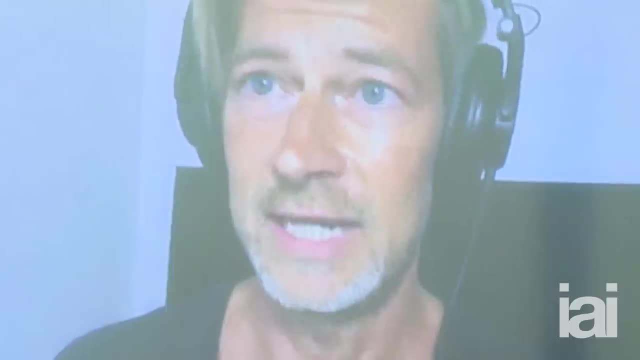 since we are talking about how we understand our universe. understanding relies on explanation And the power of a theory traditionally lies in its power to explain something. And when you look at the field of physics and cosmology, the way it's developed over the last century historically, 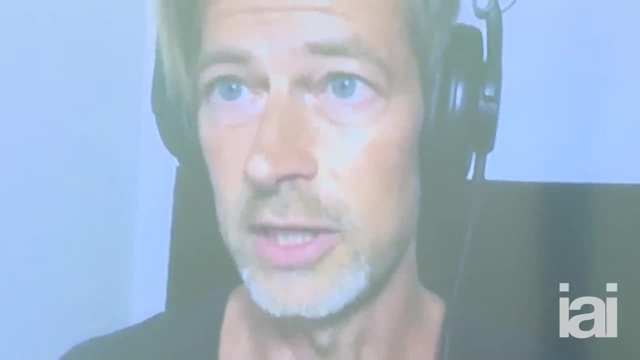 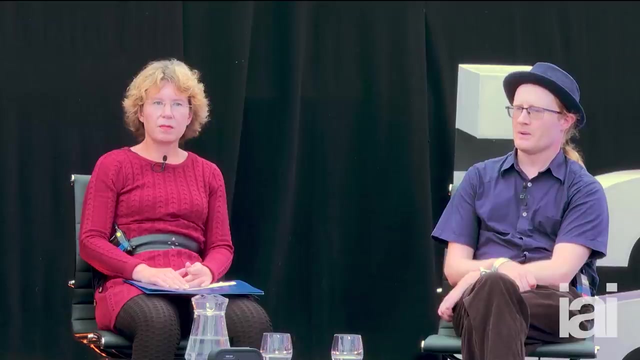 speaking, it's become better and better at describing phenomena with more precision and detail and layers, but it's also become poor at explaining them, And I think this is part of the problem: that there is a lot of people inside and outside of the scientific world who are not. 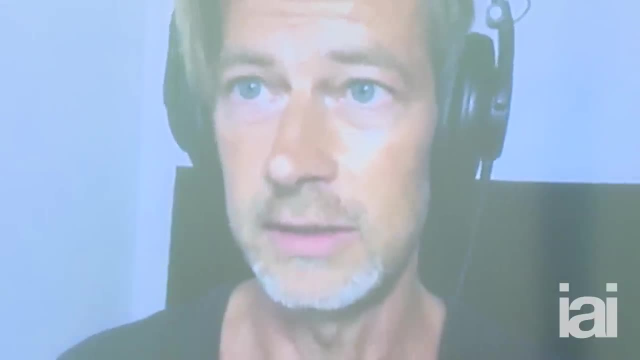 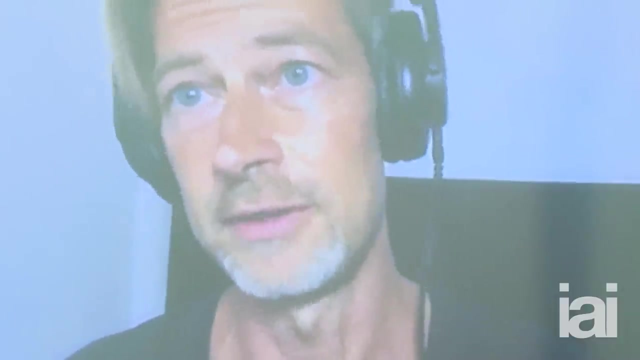 outside and outside the scientific community are finding the current paradigm wanting for. something like it doesn't explain very much. For example, if Maugham becomes the favored theory over dark matter, what does it mean, for example, that the implication that gravity is variable at large? 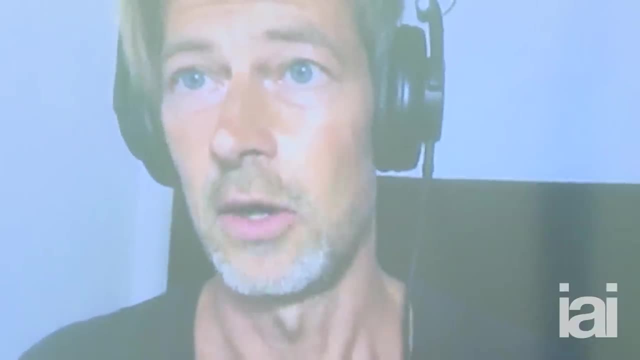 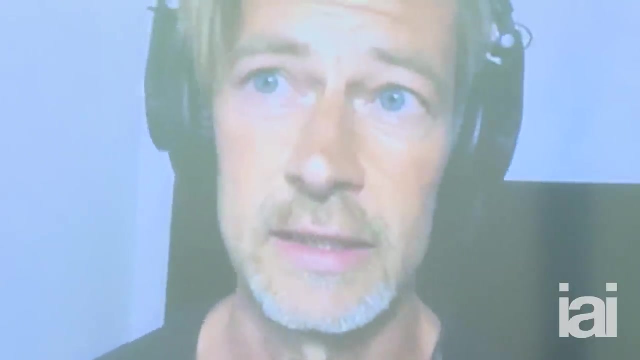 distances, which is what Maugham presupposes- that our loss of gravity as we know them, in our, in our own galaxies, that don't actually translate further. what is the implication of that? And that is, I suppose, these are the kinds of questions we can get to, But I am not sure if 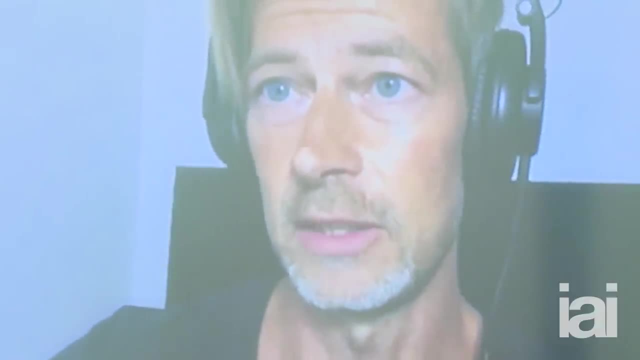 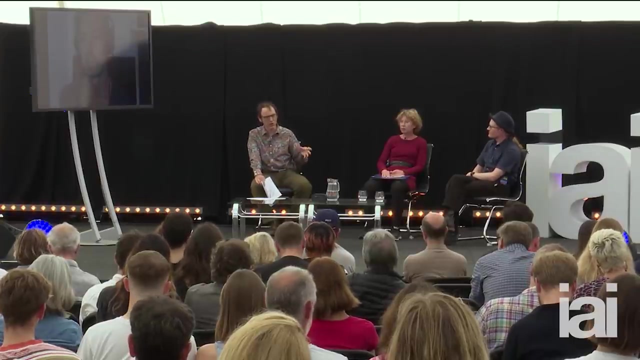 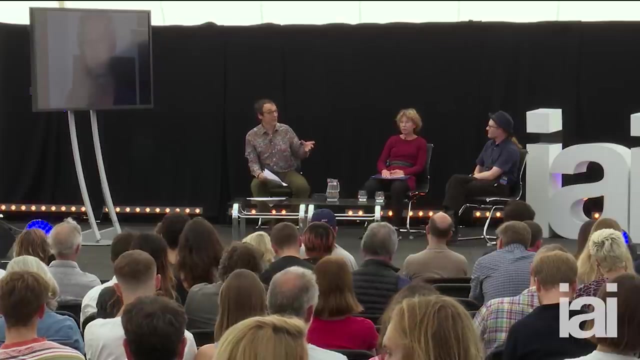 this alone warrants a major paradigm shift in the context that you're discussing here, Sam. I wonder about these issues from from your point of view as someone who's working on these experiments. that happen, of course, in vast international teams, trying to look for things that are very, very hard to see and probably you know making. 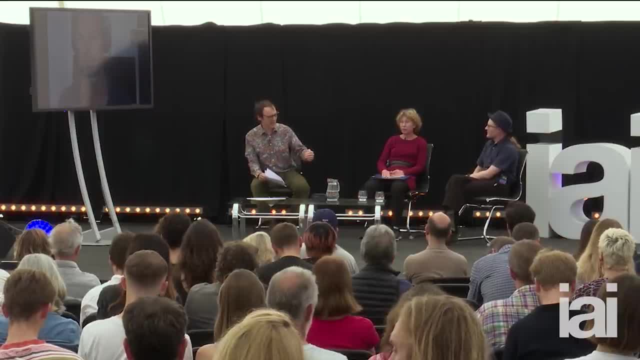 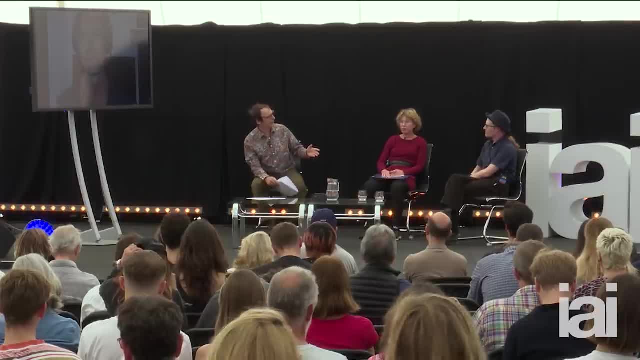 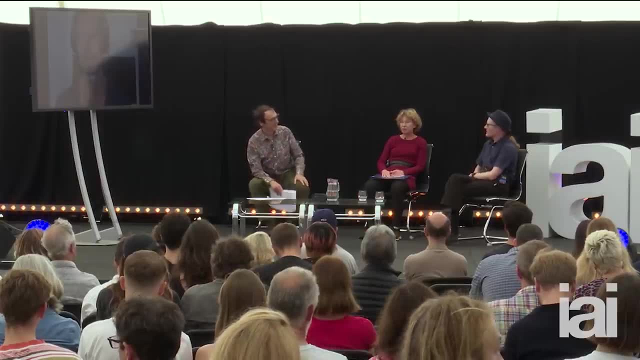 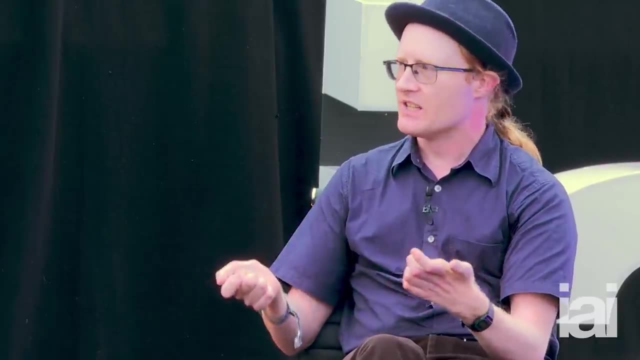 you might find something that really profoundly upends our understanding of the way things work. Is that part of the motivation? Well, I think that's. that's not something really we expect to find, because I guess everything we do is always building on everything that's happened over the last 20 or 30 years, And so 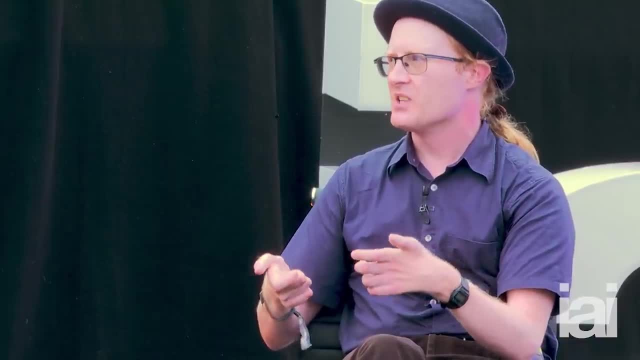 any changes that we expect to see will be for a short time. long term, Long term. Thank you, Sam. Thank you, Elian. Elian from Chief Energy can probably be explained by just introducing another particle into the standard model. 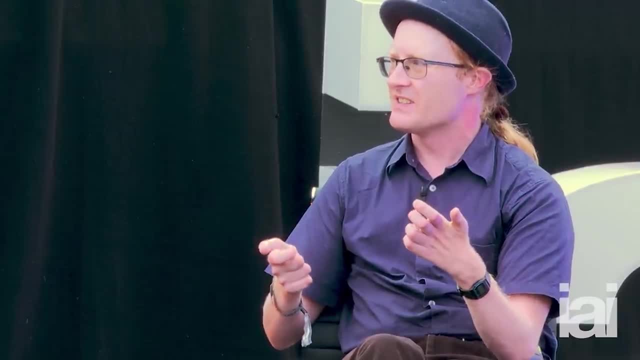 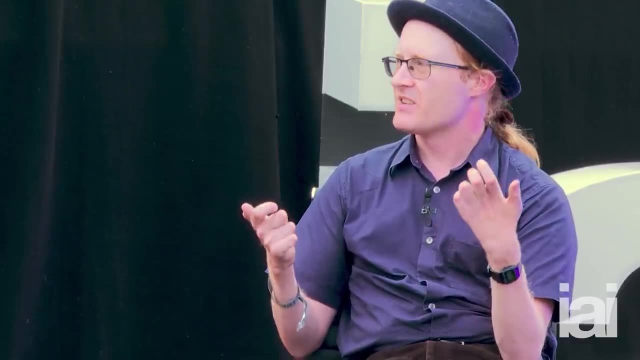 But I suppose we always live in hope that we're going to see something really unexpected, And I guess maybe one way we can imagine what might happen is: let's think back to a great paradigm shift that never was, And that's 10 years ago when, for a short period, the 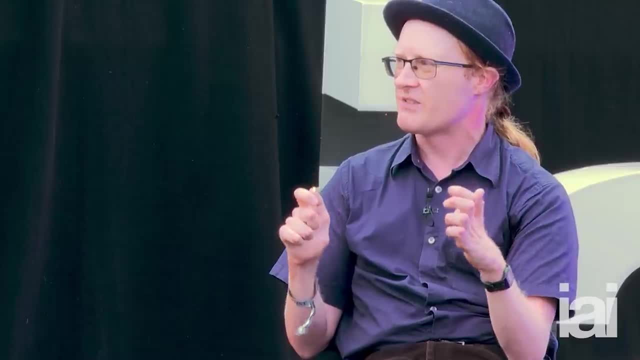 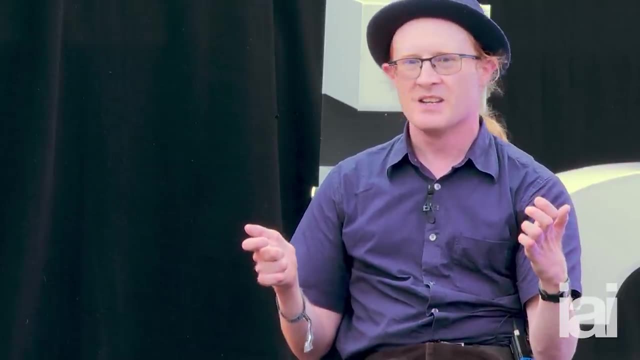 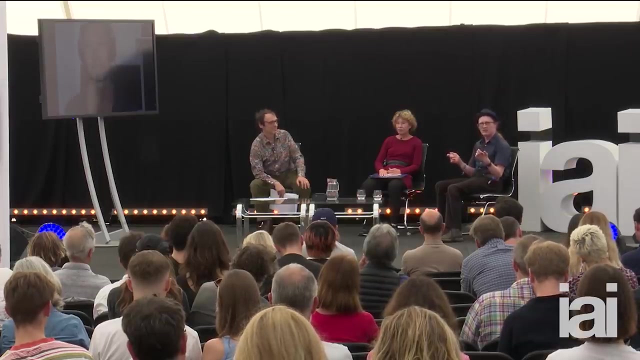 OPERA experiments convinced everyone that they just might have seen neutrinos traveling faster than the speed of light. And nobody believed it because it was very difficult to fit in with our existing framework. But the idea was just so exciting that for a short period it was all people could talk about. And how could we possibly rewrite the laws? 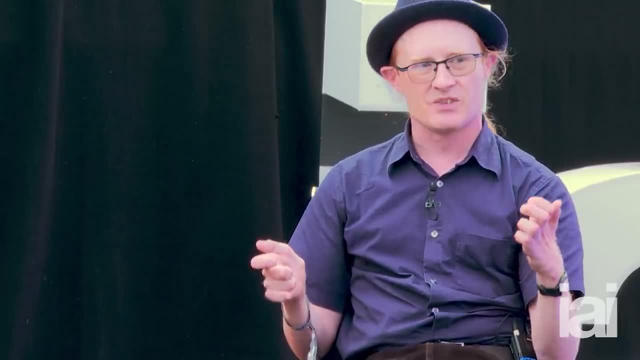 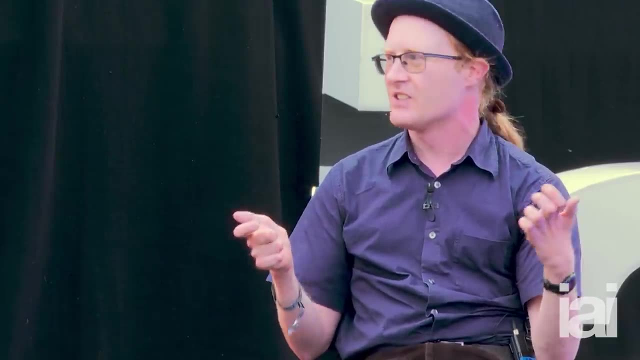 of physics to accommodate that, And everyone was really excited about it, And that was not just in the particle physics community, It also got a lot of media attention. The idea that particle traveling faster than speed of light got a lot of attention, And so for. 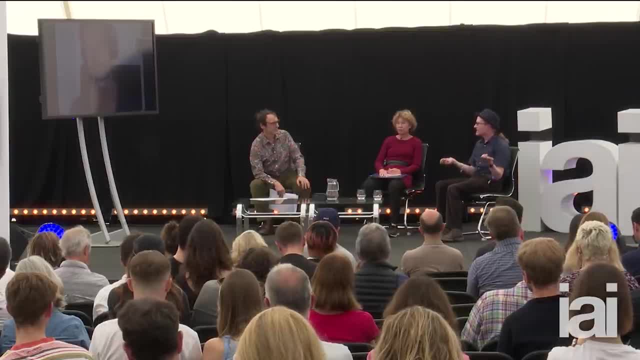 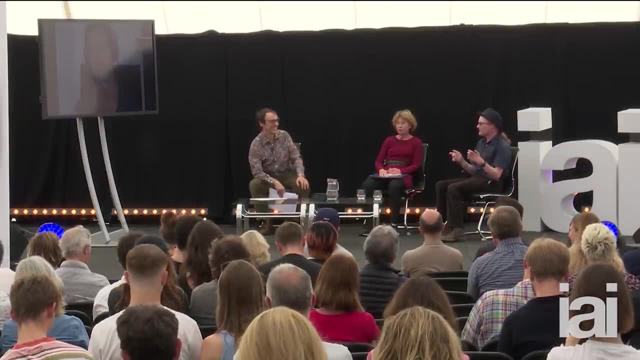 a brief period it was really exciting. And then of course it was a rather sad end that it turned out to be a faulty electronic module and an optical fiber not properly plugged in. But I think that at least gives us some sort of idea of the kind of excitement we'd see. 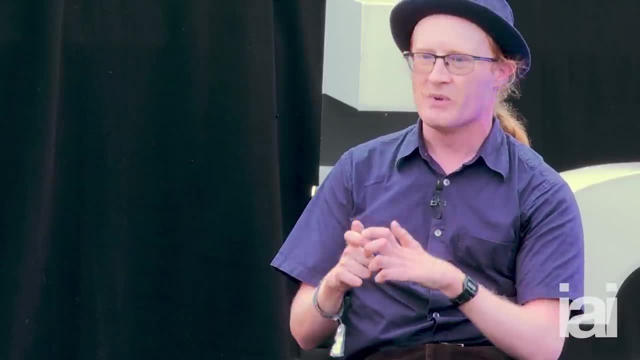 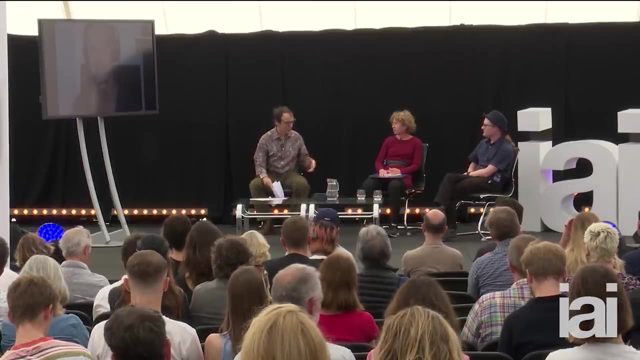 if there was some sort of unexpected result that did point at a that we need to completely rewrite our whole framework. Serena, I get the impression from you that sometimes part of the motivation you have for thinking about these things- and it seemed to be what you were sort of saying in Lost- 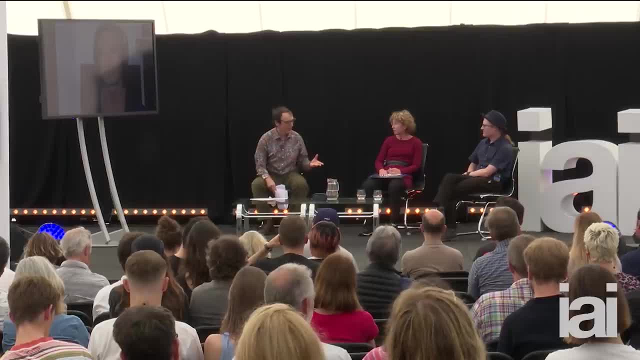 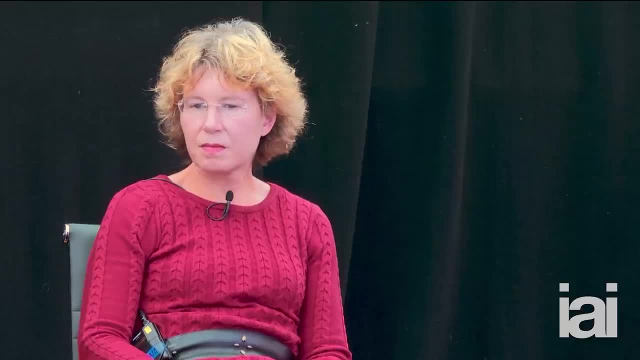 in Math. is that you want to challenge the way that I might be too broad to say the way science is done, but there are some things about the way this science is done that you feel could be done better or differently. Can you say? 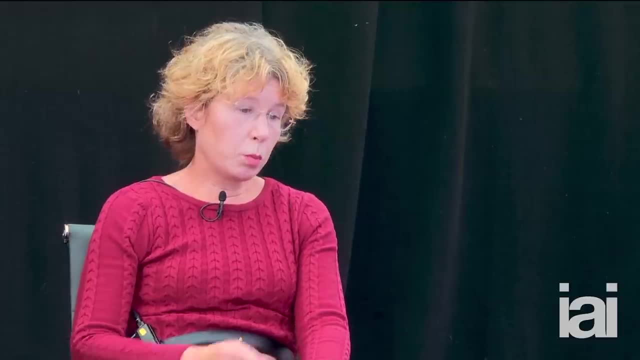 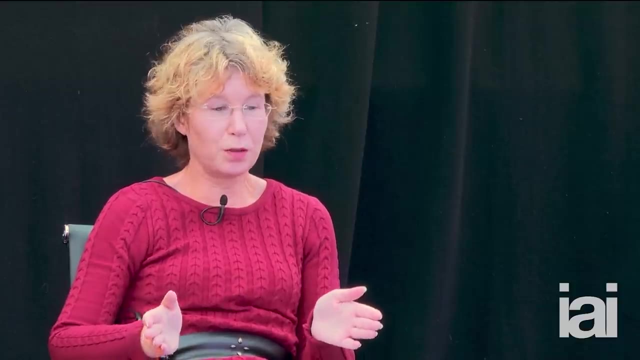 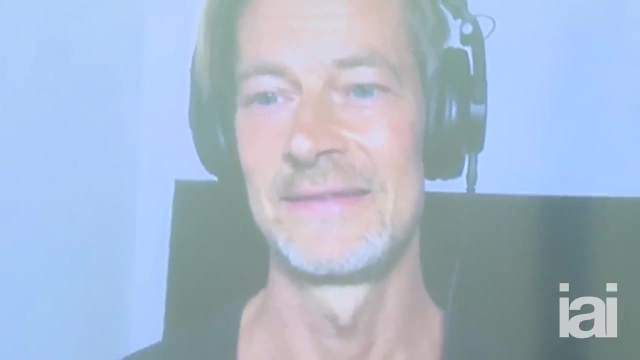 something about that. Yeah, exactly. So the opera anomaly, by the way, was another example where theoreticians were very, very quick to find all kinds of explanations, which drives home the point that it's fairly easy, with the current methods that are currently accepted, to explain pretty. 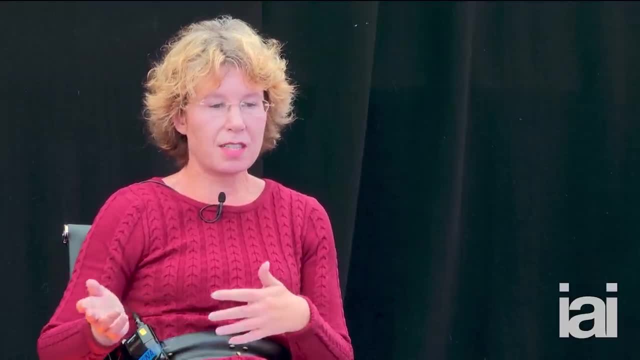 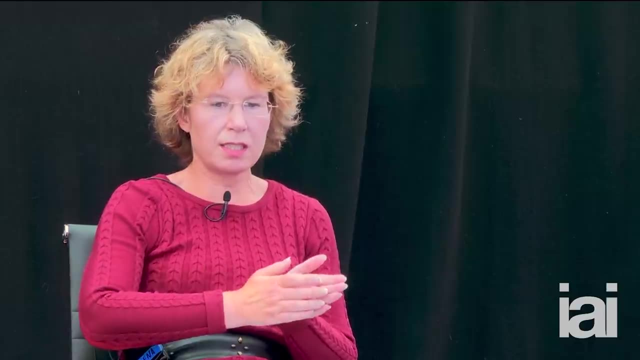 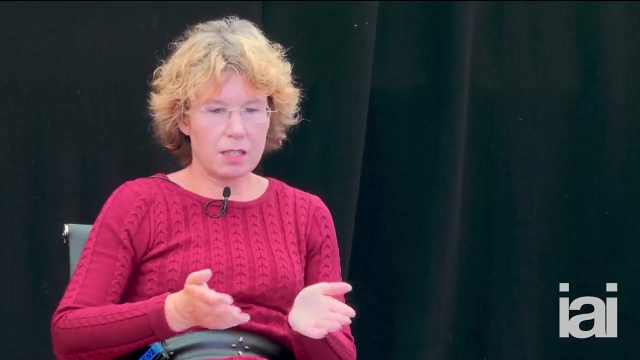 much everything, And so we talk about the scientific- I mean the scientific method- as if it was a fixed thing. but it's a living and evolving thing, and what counts as good science at one point in the history might no longer count as good science 100 years later. And I think that in the foundations of physics we have 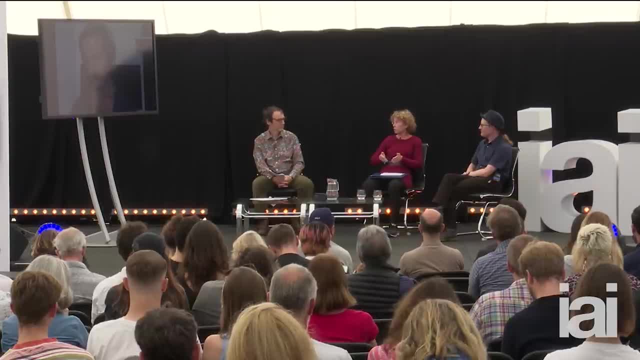 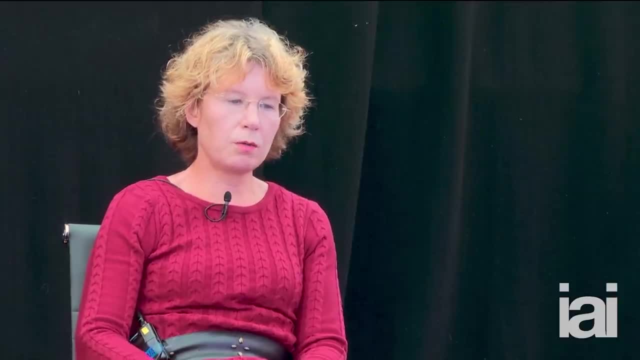 to ask like: do we need to update our methods? And for me, the answer is clearly yes, we have to. We have to be more careful in our theory development, more careful to write down what the assumptions are and to ask questions. 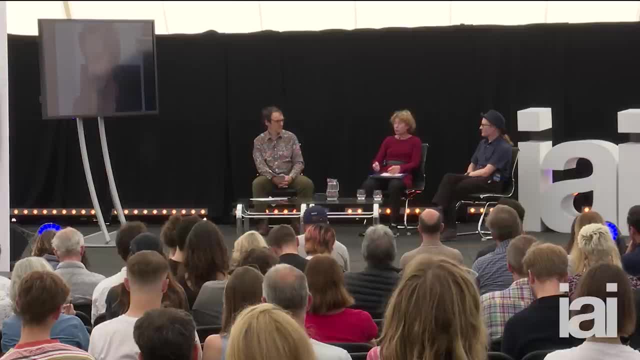 So I think that's a really important point, Thank you. I think it's important to ask whether they are justified. So, for example, this conversation we're having here. I think it's great that we're having it, but I think there should. 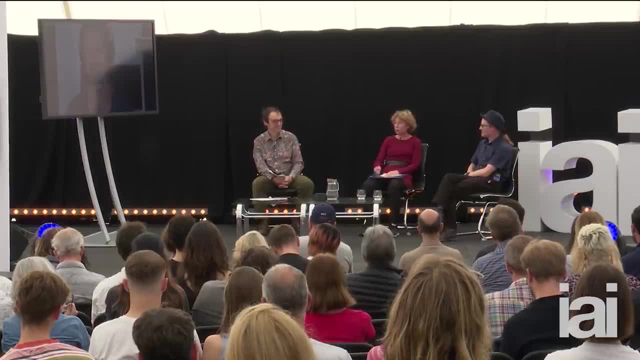 be more physicists having this discussion. But maybe if I can say something about your question of, does it even matter, which is kind of you know, if you ask this question among physicists, it's kind of blasphemy. It's a question you're not even supposed to. 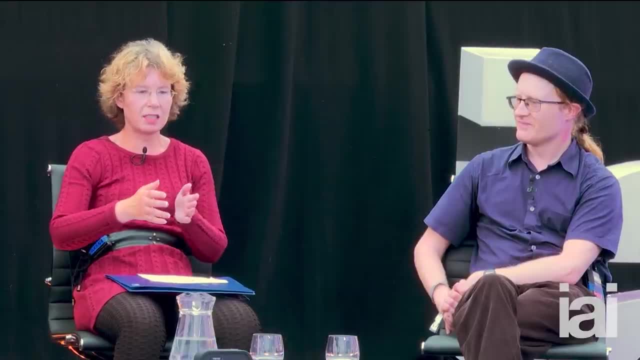 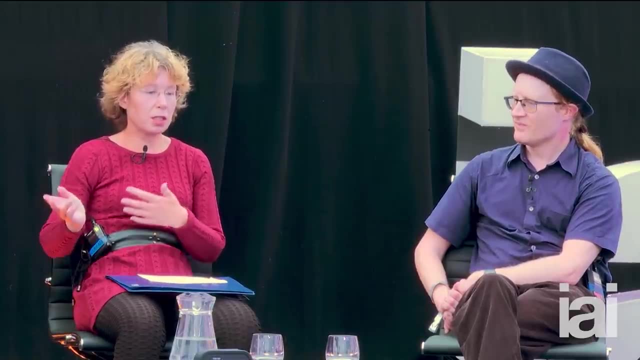 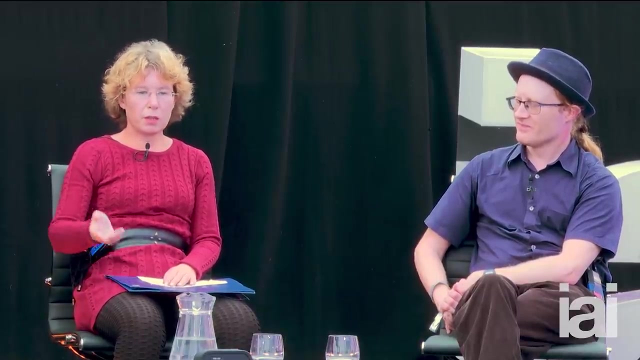 ask, But I think you have to be more careful about adding like: does it matter for whom and when? So it clearly matters For particle physicists, you know, if we don't build a bigger particle collider, that matters to them. But does it matter to society? if you know, we find a crack in the standard? 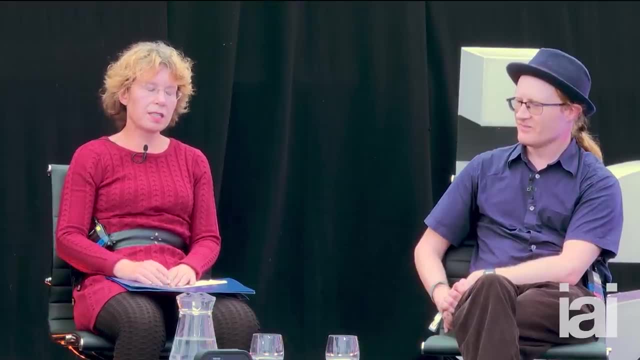 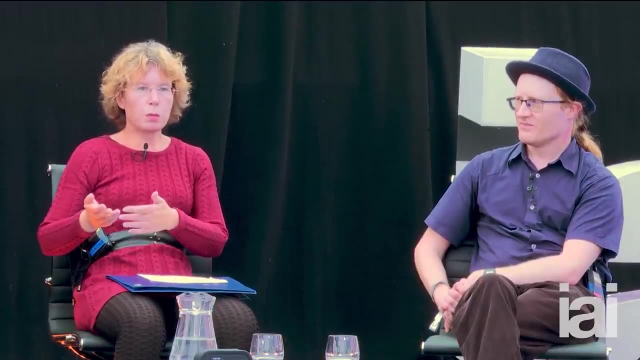 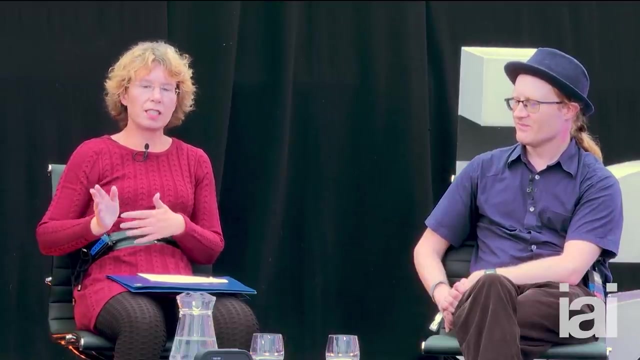 model, if we find a new particle, that kind of thing, And that depends very strongly on exactly what it is. So, as I said earlier, physics is a very mature discipline and the easy things have been done. This also means if we find something new, it's very unlikely. 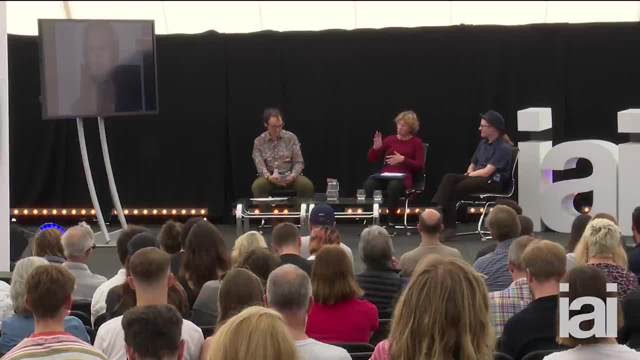 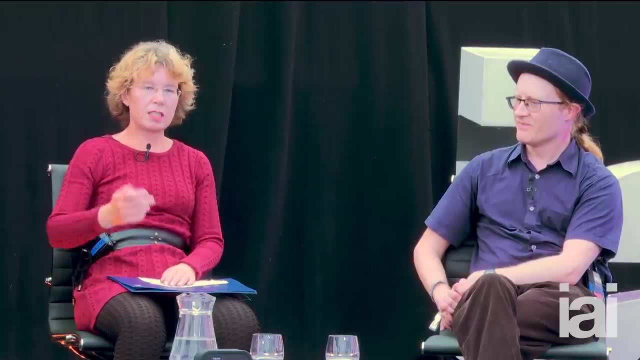 to have an immediate impact on daily life, Just because if it's difficult to measure, it's probably also difficult to use. So if you know we find some particle that makes up dark matter, I can't really see what difference it would make for daily life, But there may be some- you know- consequences in the future. 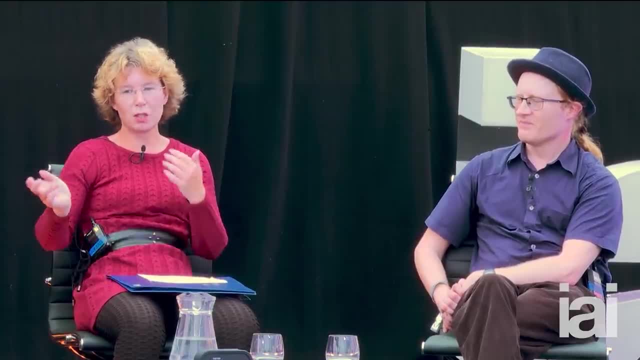 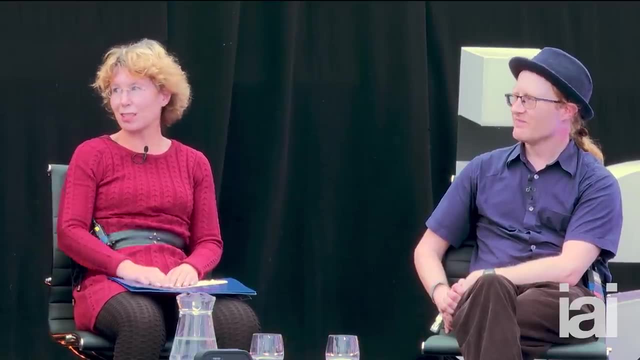 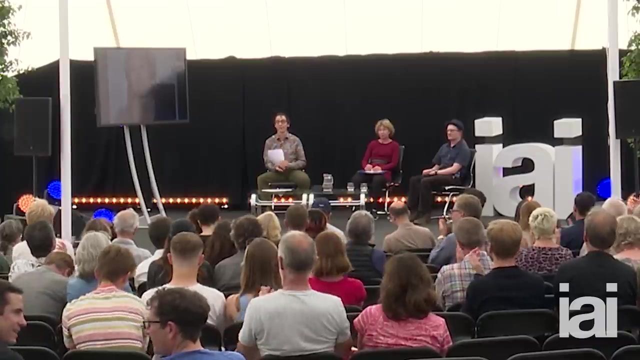 You know you just discard MOND as something that would never be of use to anybody. But I don't know. You know, if one day our civilization manages space travel, maybe we should know how gravity works. Can you please join me in thanking our panelists today, And thank you all for coming.